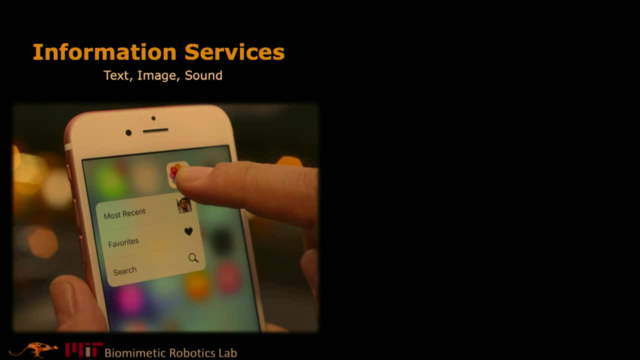 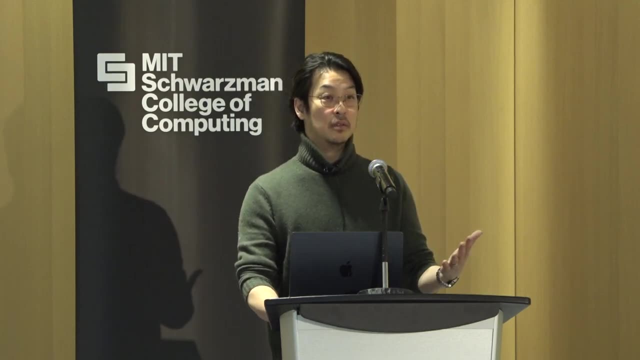 You know, always we underestimate the consequence of long term. It's still progressing. The amount of the screen time, even adult, of course the teenager- is still going up. This is very staggering. I thought it about five, six years ago. 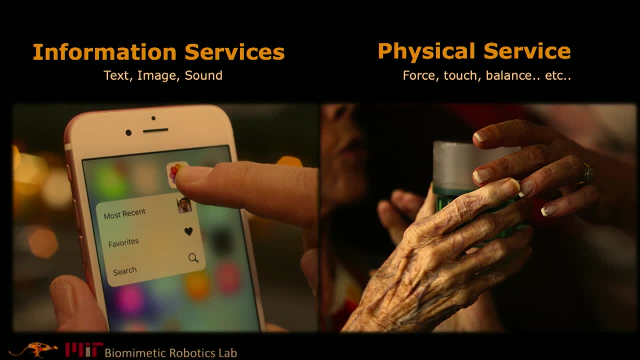 This is going to saturate Service. there's not much we can do. I didn't expect people are going to spend way more on this device, So still there's demand going on. But again, if you're going to the real critical life, critical issues are all in physical. 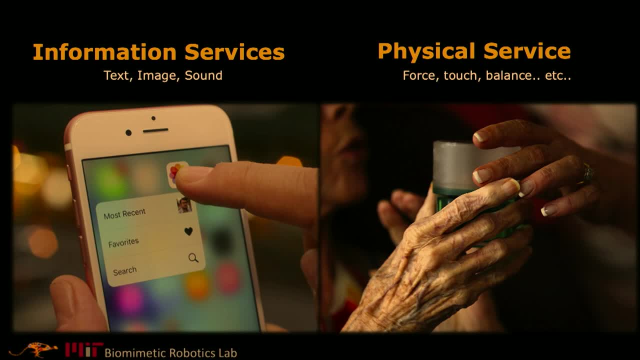 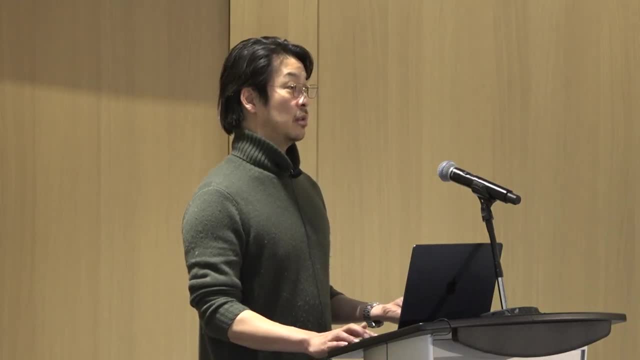 We still need to eat, still need to deliver stuff, You need to heat up your house and all these service. in the physical world, You can just gather information in the information service, And that's where it's going to be really crunching. 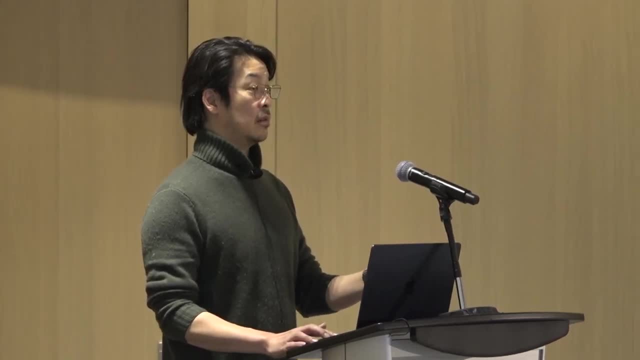 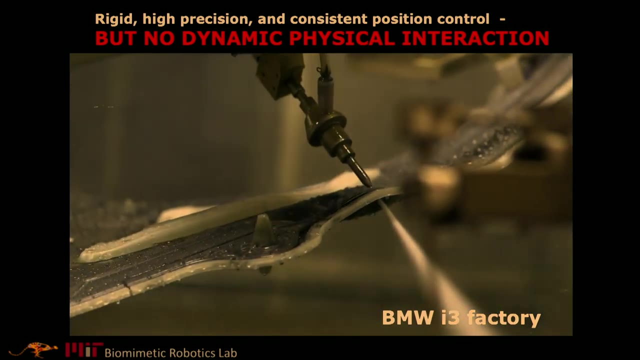 It's already happening in all this company, a country like a manufacturing company Like China, Korea, Japan and so on. So I'm going to talk about physical services And I still think this is like this industry has been progressing relatively slowly. 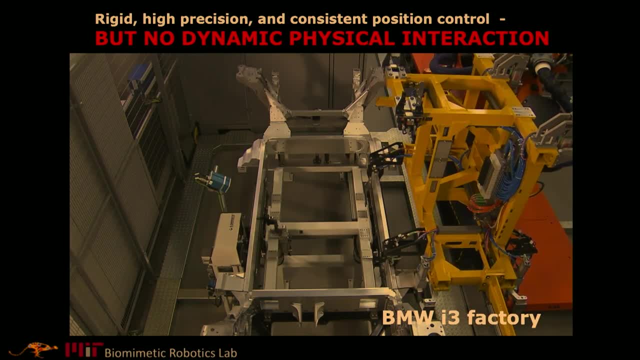 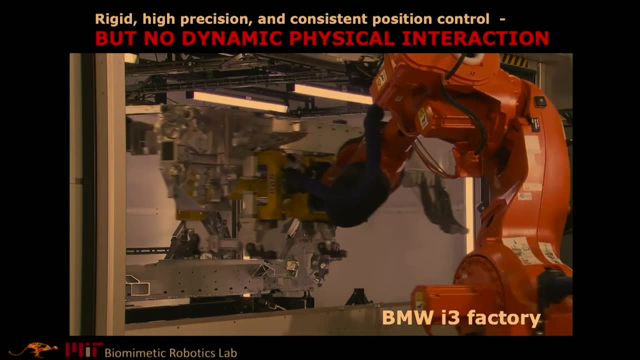 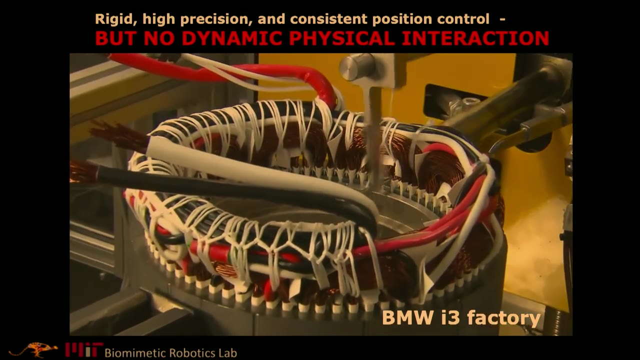 but fundamentally didn't change much from 1970s After Victor Simon, who invented the first program of six degree freedom arm. These are the physical services that actually have a bigger, like a significant impact in our life. That's why we could buy cars in $20,000, not $200,000. 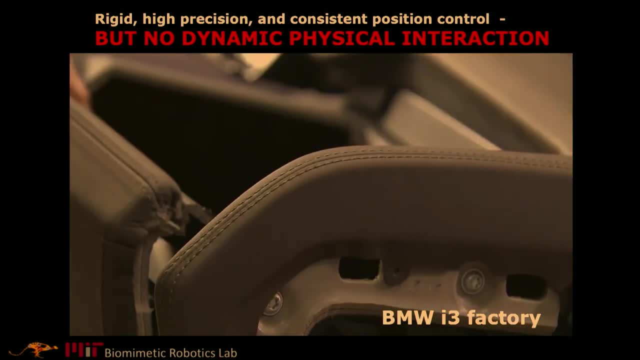 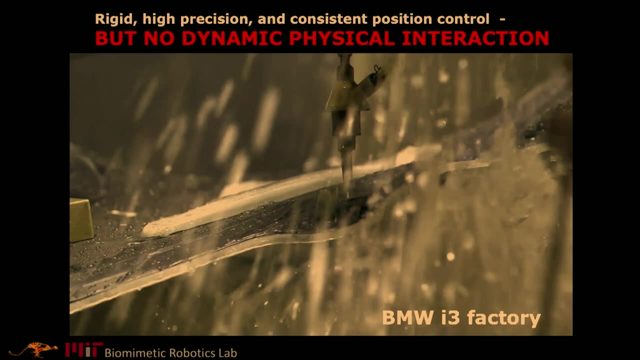 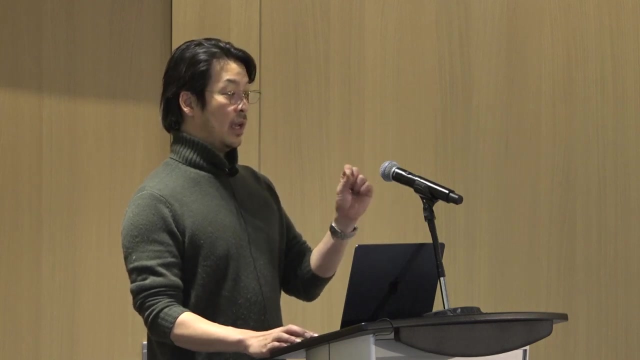 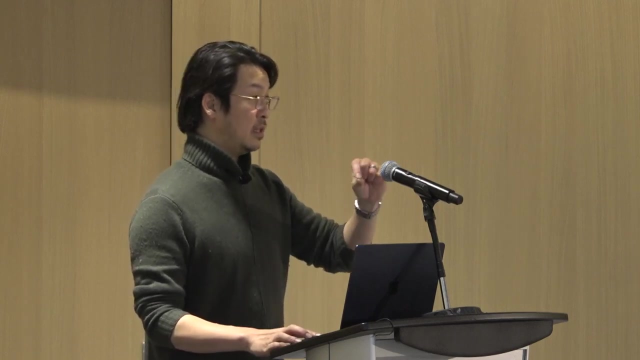 Yet this is probably the most automated space. humans are there Because these tasks cannot be done by manufacturing robot. One of the reason is that they avoid any dynamic situation, any collision situation. Every problem is solved by just push of control, Because anything else, any sensor feedback, is going to have a potential errors. 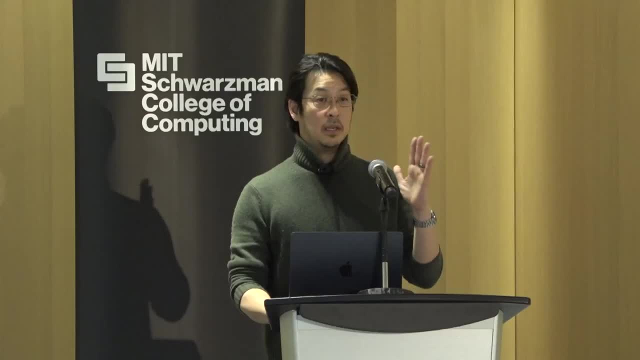 And then that will have an impact on their reliability. I'm not sure if you guys are familiar with. the actual useful success rate of machine is actually 100%, Maybe 99, and then there's about 29. maybe A lot of people post success rate in the papers. 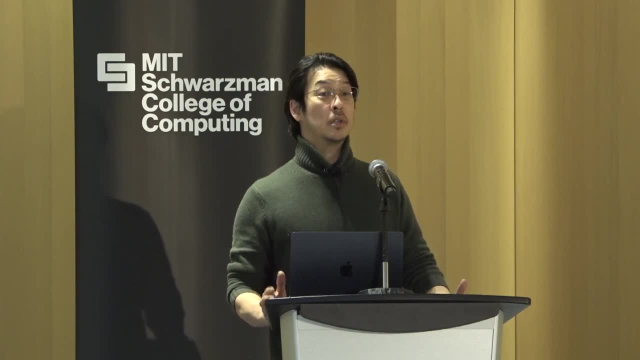 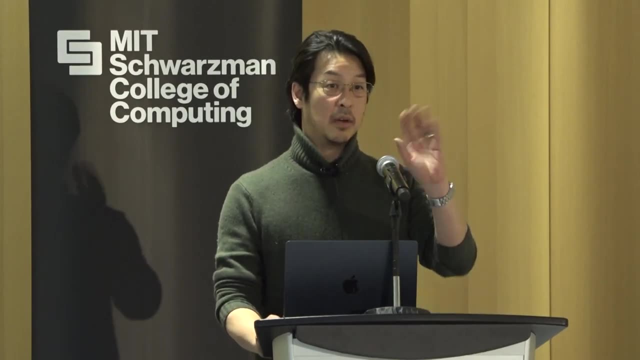 99.9%. I never heard of, which is useless in the real world. All these robots are 100% or 99.9%- At least 10.9 after this, And then it's becoming useful. So I want you to really understand that part too. 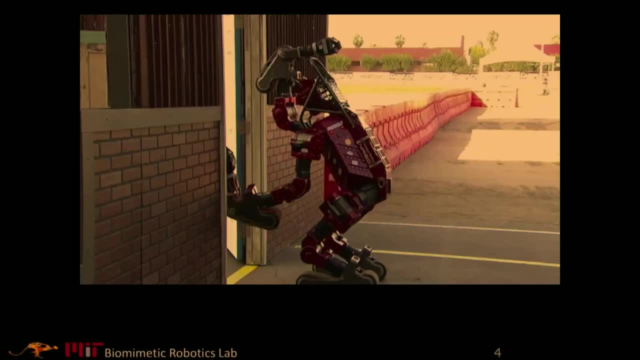 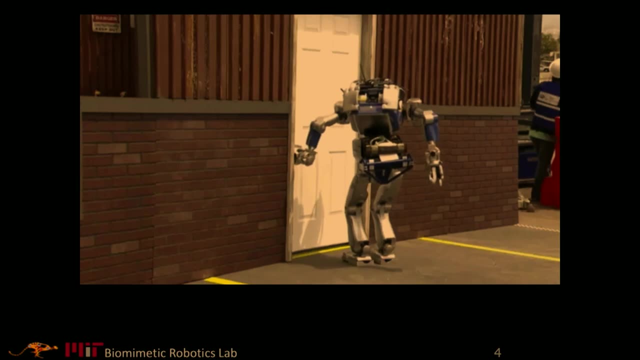 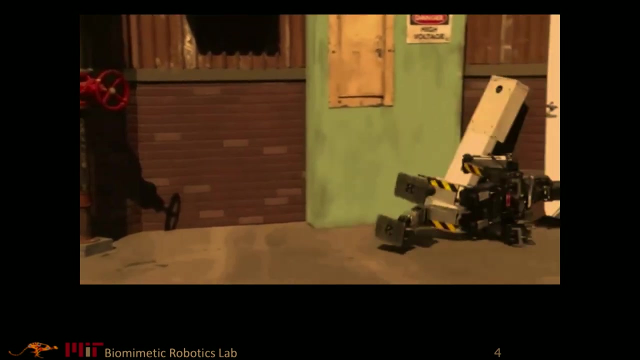 That's why they're avoiding all these complex vision based touching. No, no, there's all push and control blind machine with some sensor based. emergency stop 2015,. probably any of you already saw video- still relevant, Because this has been a pretty big push from the DARPA, spending several hundred million dollars. 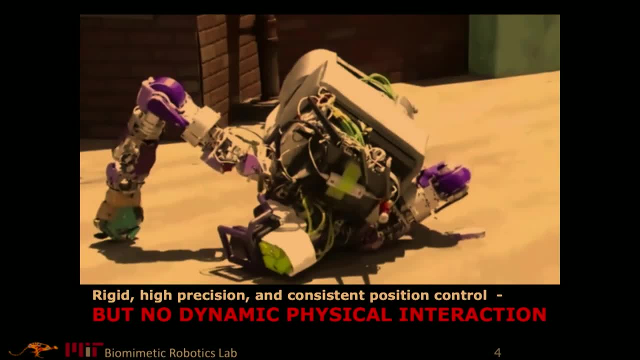 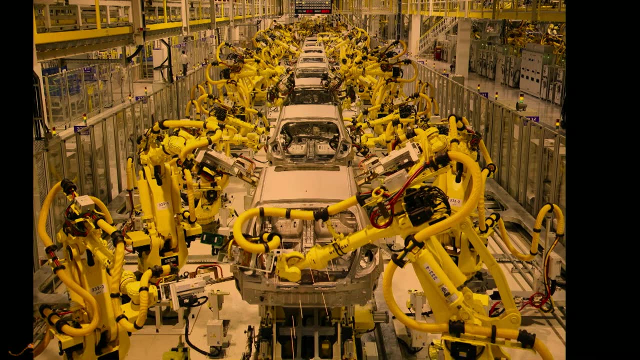 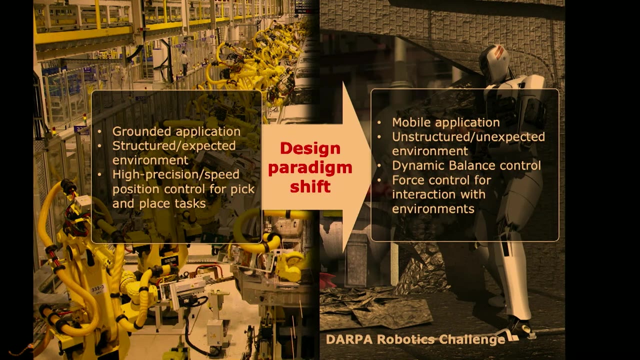 They look like all superhero, But if you look at, take a look at inside, These are all same technology, as you saw in the previous slide, is manufacturing robot. So in my career at least at MIT, I've been trying to Shift the design paradigm from more like a manufacturing setting where position controls over everything, to more uncertain environment. 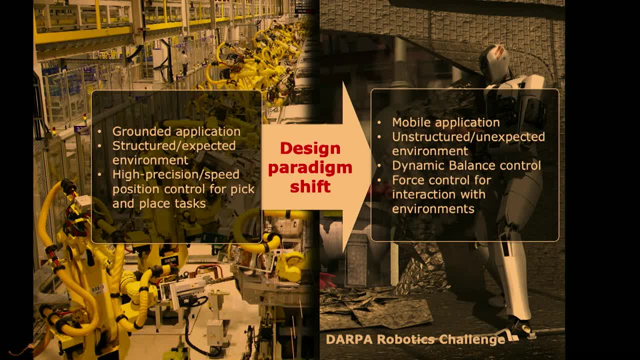 The closest thing, like closest to things that are about to happen is like Amazon picking or Amazon stowing. Amazon stowing team is actually Led by my friend And he gave a wonderful talk, which I wish you have more real roboticists like that in the campus. 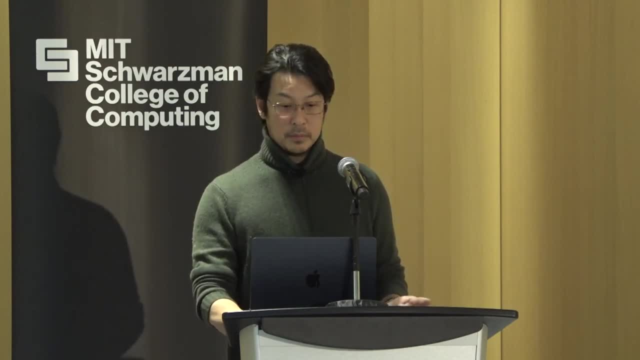 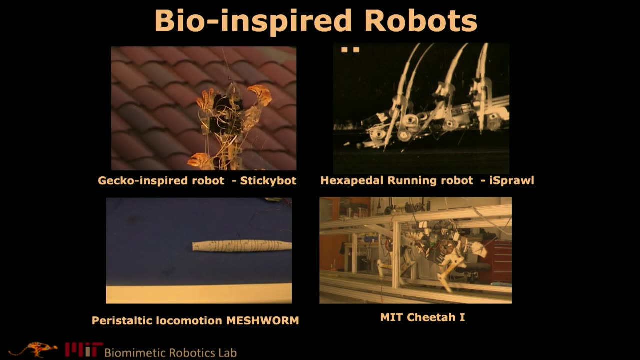 We can actually understand real world. But before that, because of the topic is bias. but I will briefly talk about my previous work, which is before I came to MIT. I'm not sure if you heard about directional adhesion. The sounds oxymoron, but it's actually my PhD work. 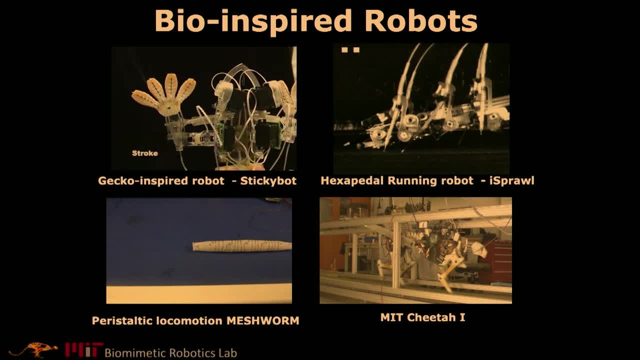 This adhesive only works one direction. Doesn't work in the other direction. Sounds very strange, But that's how It works in the other direction. So it works against gravity. It can hang stuff, But once you take out the gravity it just comes off. 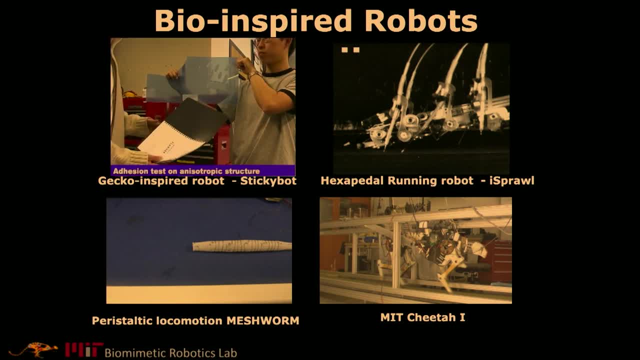 You probably only see this kind of behavior on the hook. There's no hook, It's a smooth surfaces And we. If you do that with a double sided tape like a typical outside carpet tape, it doesn't work. You have to pull out with a lot of force, which is not a good thing. 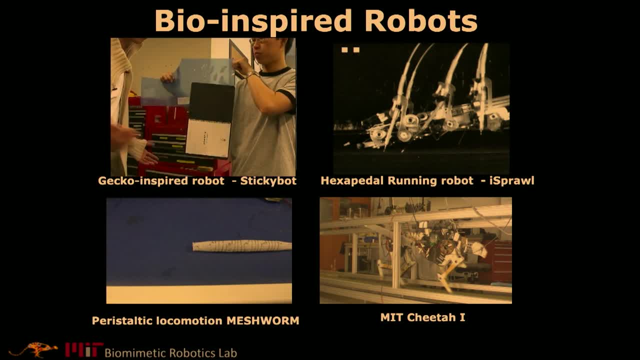 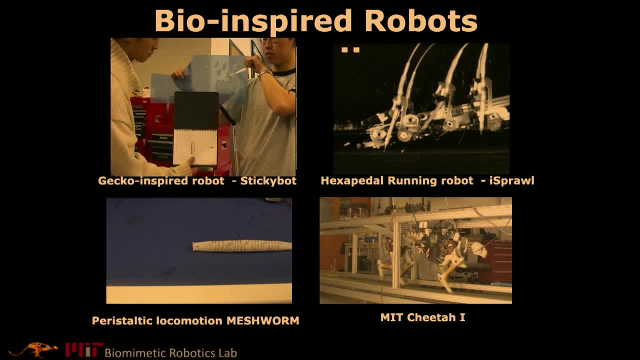 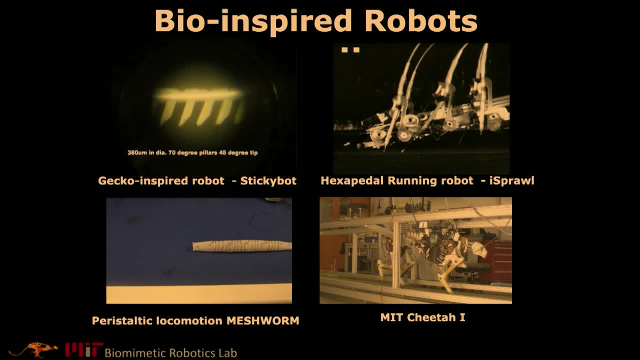 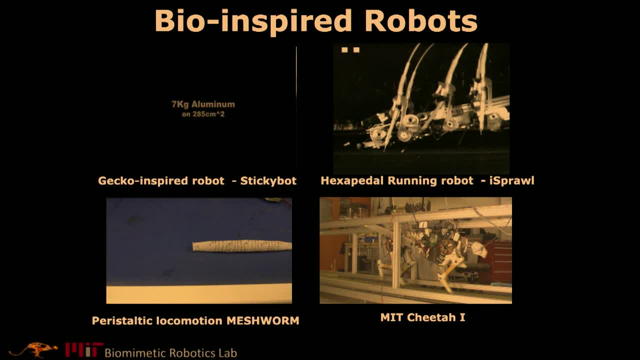 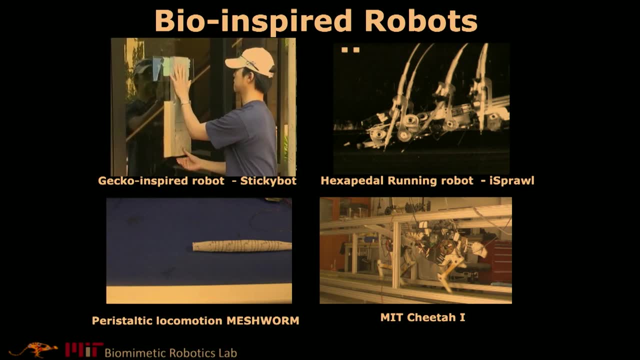 and geometry, And Gecko has the orders of major- more complexity, with the orders of major more smaller features. to achieve this, We grabbed the principle to achieve this And we could hang 15 kilogram aluminum And then you can detach that from glass with a zero. 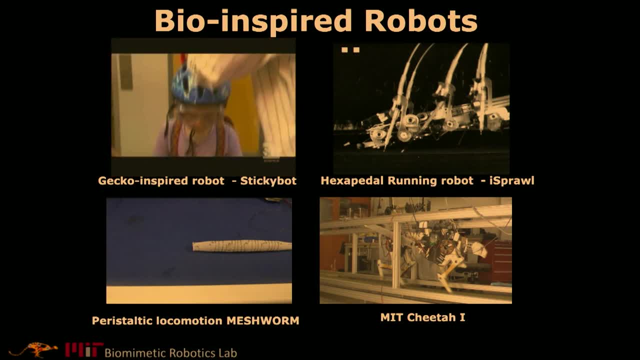 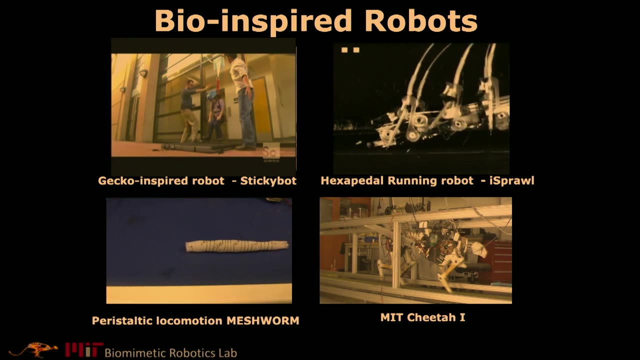 zero force and then we hung a person on it And, of course, once she's out, there's no force on the glass. I don't want to spend too much time. I've been working on cockroach inspired running robot and some soft robot. 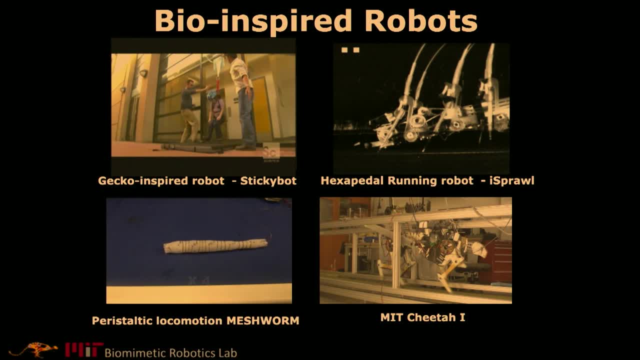 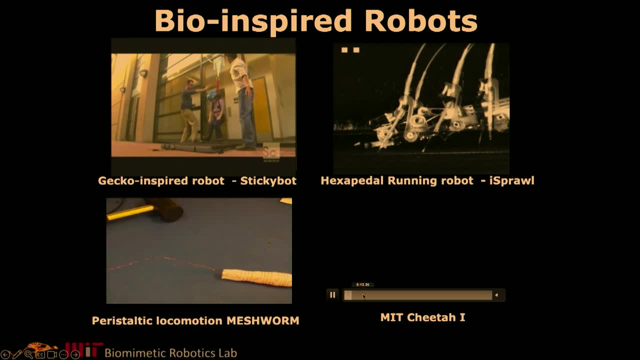 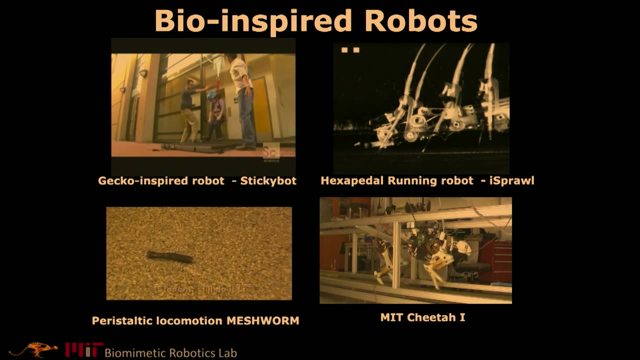 This is one of the earliest soft robot which has no rigid components, And when I came to MIT I started working on bigger machine And I want to build something that can really serve in our environment. So I built a cheetah. I bump up the weight of the robot at two older megatons. 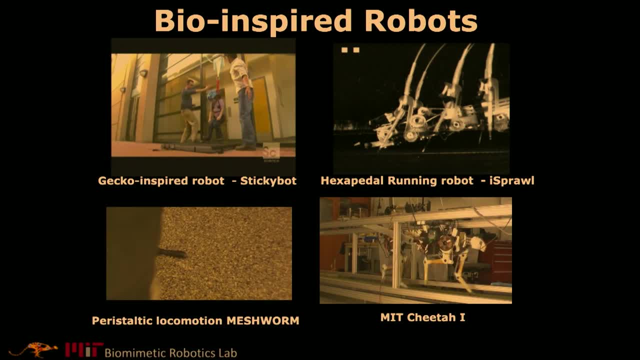 The smallest robot I built. the biggest robot I built before was like 400 gram. This was 40 kilogram And then this wasn't be able to run without any support. But we learned a lot about what kind of actuator we need to use. 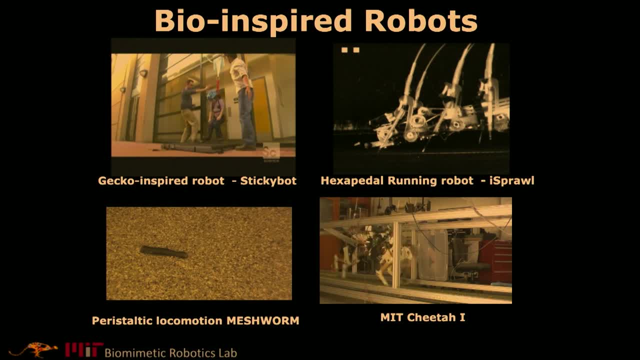 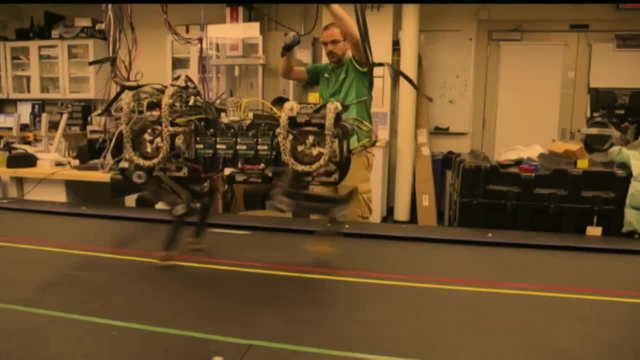 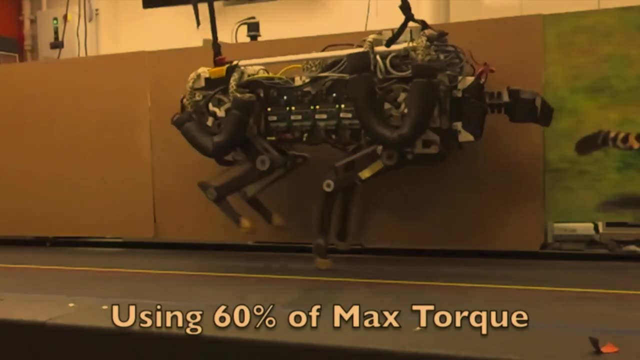 This paradigm is completely different from manufacturing paradigm so people didn't know. I'll briefly explain that. later I'll show you a summary video of after story. This is mostly quadruped robot And this robot was still the highest efficiency holding the, and then at the time, the fastest robot. 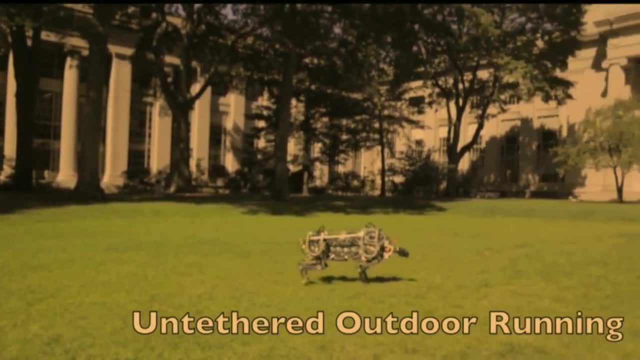 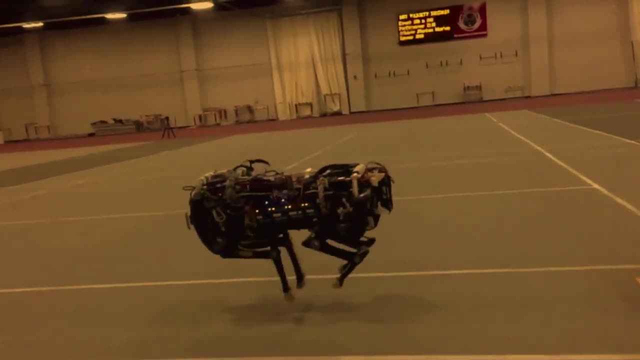 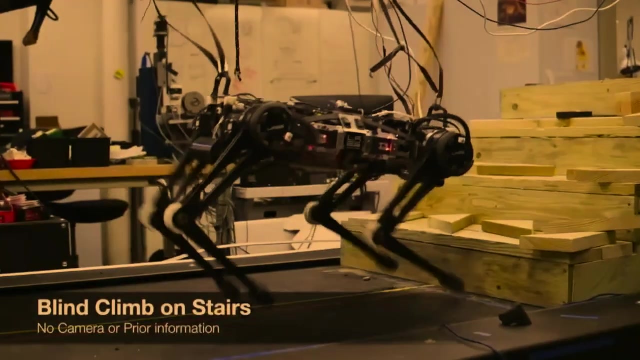 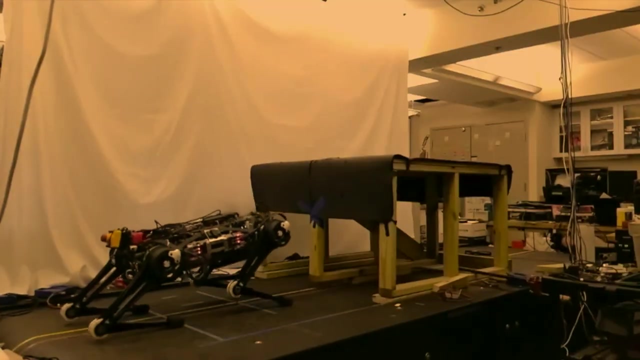 you can run and familiar part of the campus. And these are all heuristic based controller with some very simple physics. It's very similar to what how? Boston Dynamics building controller. And then this is where we start moving to like true MPC Model Predictive Control. 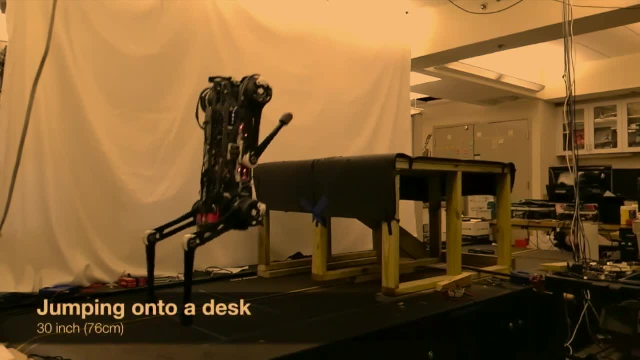 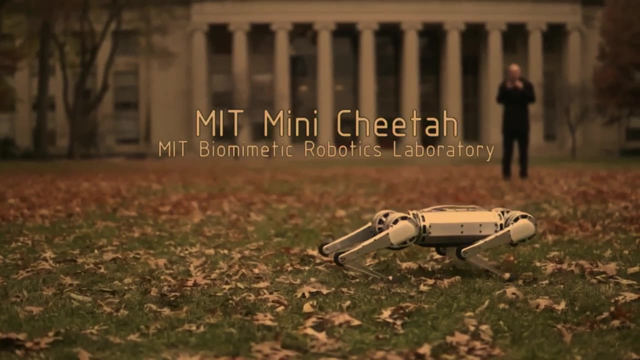 Very versatile so you can go to many different gates and so on. This is just show off our muscle, Because we actually do research on actuator as well And we really wanted to make it safer. robot because 40 kilogram robot with the torque of a regular car. 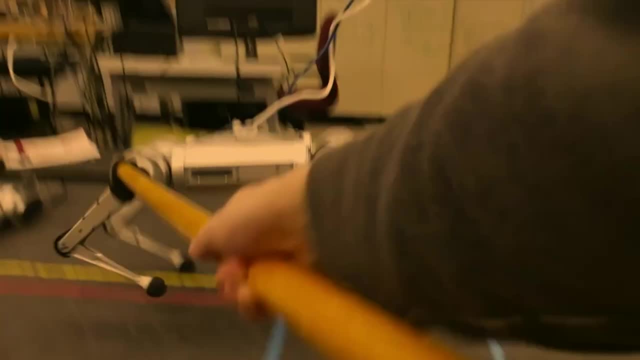 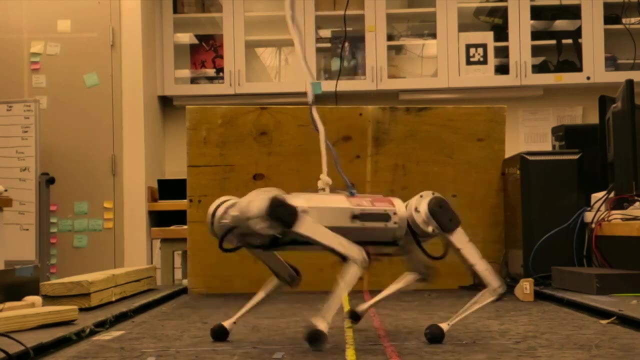 engine is too dangerous, So we built a smaller machine. If you're familiar with the allometry scaling, the weights go scale a length, scale of power of three. Torque goes a power of four. So if you reduce 60% your torque will come and drop like. 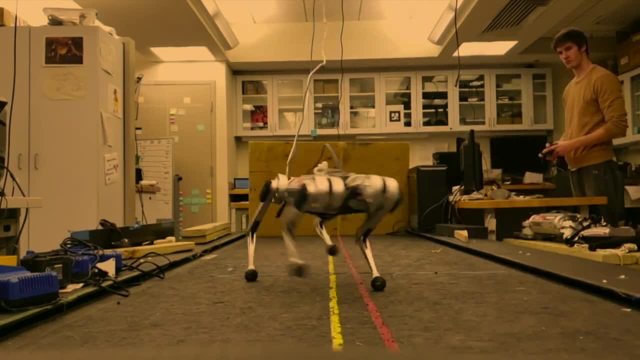 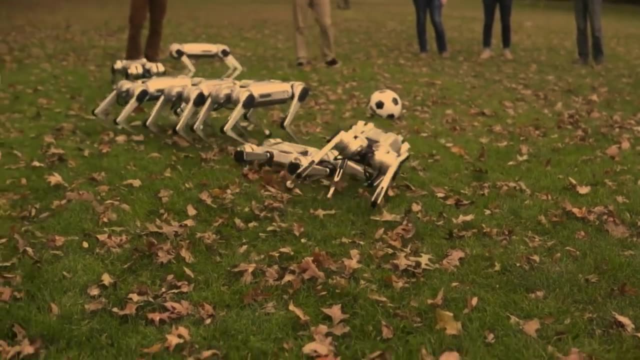 significantly, like 12 times or something. So we got very, very safe And then they get popular. Now they're about- I lost count- like the 30 plus. companies are copying our machine and then selling Mostly education purpose. There's no real market. 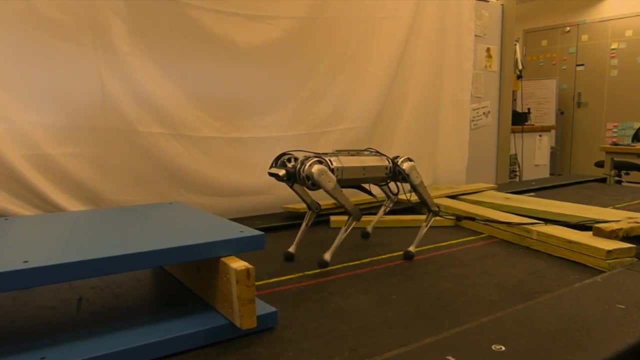 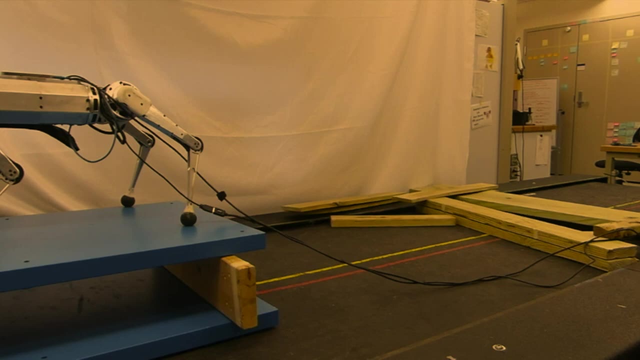 I think Boston Dynamics will get mad at me If, if I said it. but the market is relatively small, The service market, there's no like a large volume market yet I think it's mostly education and then the key was that enables this robot. 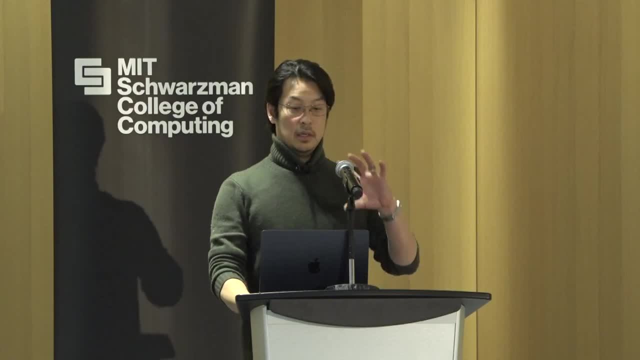 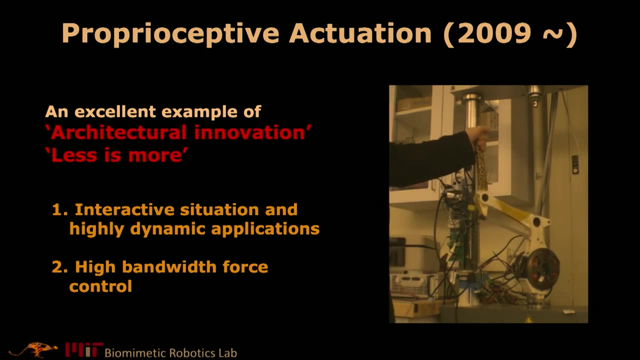 without using hydraulics was all innovation and the actuation. Again this 90% of robotics companies still don't understand. If I go iCloud this April, if I explain this, probably still 90% won't don't understand. 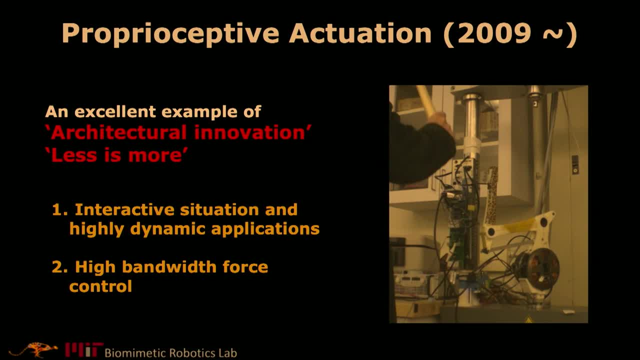 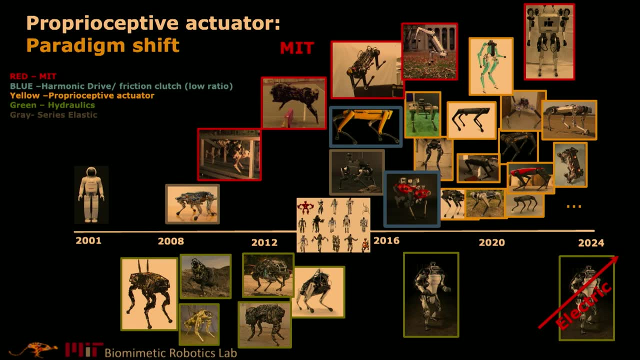 So if you have any question I can get back to you. This wasn't even common sense before we show this robot. So if I quickly summarize on with my personal bias, the bottom, the all the robot below the line, the ear lines, are all hydraulic machines. 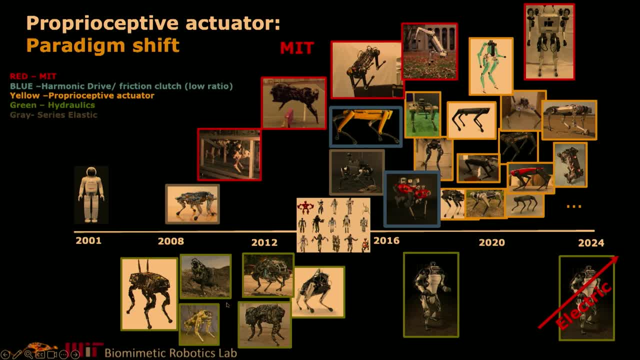 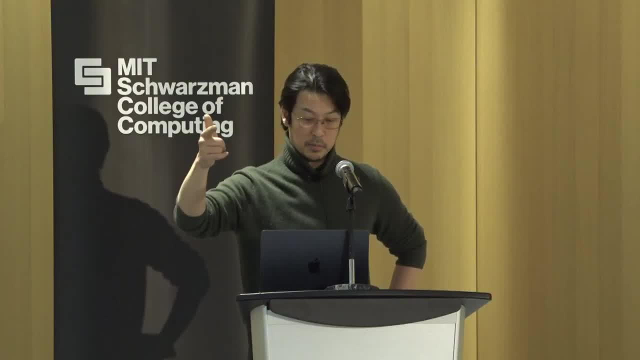 So when I first start MIT lab, the hydraulic machines were dominating Well, mostly by Boston Dynamics, And then. but the Italian is copying a hydraulic machine and Korean company copying, Chinese company copying Electric motor sucks. All the hydraulic has to be dominating. 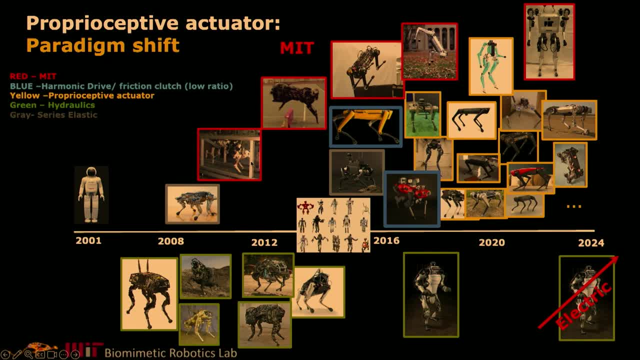 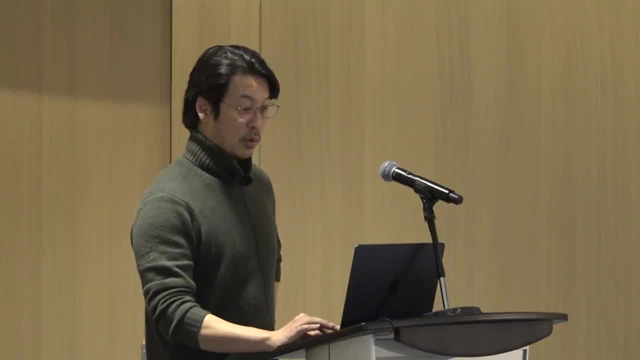 That's where I start working electric motors. Everybody says, like, what are you doing? I got even like a review from, like a renowned professor said: you're, what are you doing is science fiction or something. And then we showed running, jumping over and then landing on the show for the robot. 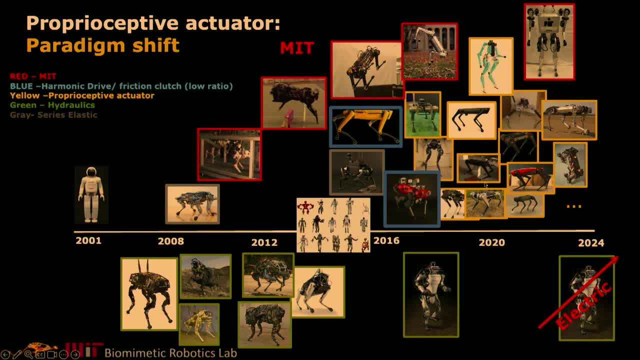 And then, after that Cambrian explosion, Almost every current company you can find- probably find easily ten Chinese companies copying our actuator to build the humanoid at this point, because Elon Musk just hyped up the humanoid. Hyped up the humanoid for no real tangible future. 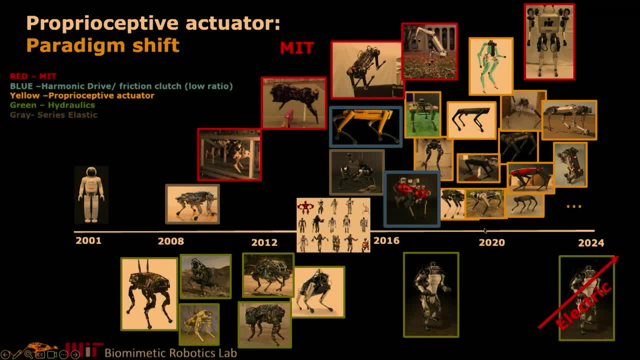 I shouldn't say for short, tangible future, maybe a long time later And after for a while. only hydraulic machine that is actually showing their feet is actually Atlas. that's the only one. Everything else is out of commission. And then my student joined Boston Dynamics and then killing hydraulic machines. 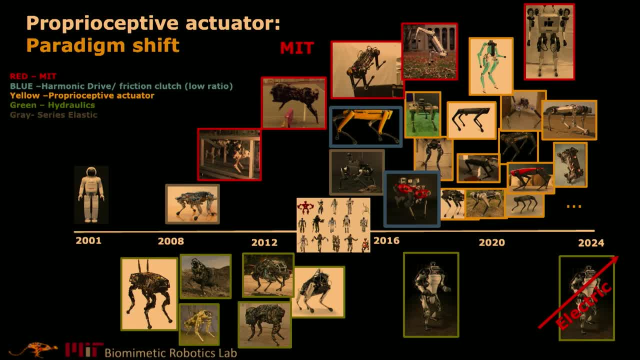 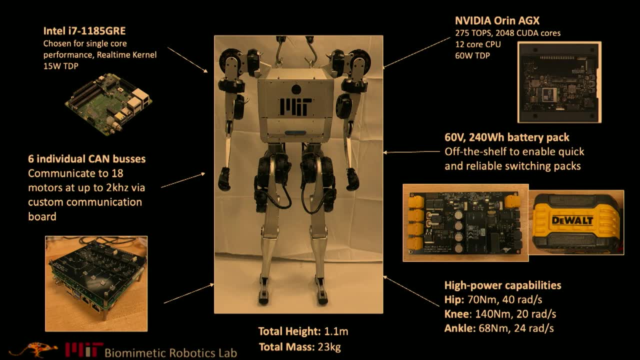 So everything is going to be every robot moving around. pretty much it will follow our actuation scheme. I don't want to talk about details, but this is basically all hardware sharing in our lab. No matter which robot you build, we're having the same infrastructure. 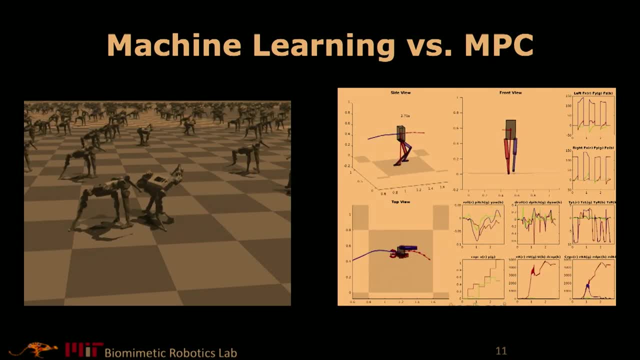 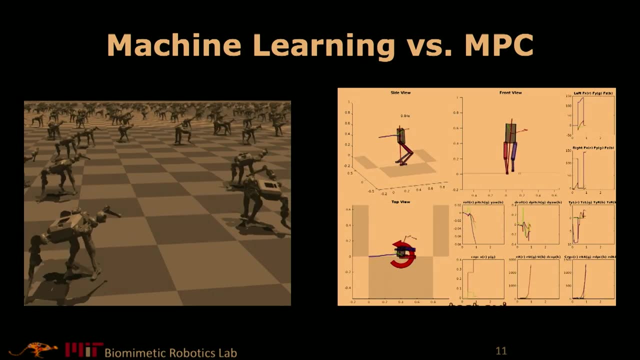 This is still probably the most heated debate, at least in our lab. I'm not sure it's just a heated debate in the conference, but we are still debating about this End-to-end. we're decisively not going to do end-to-end. 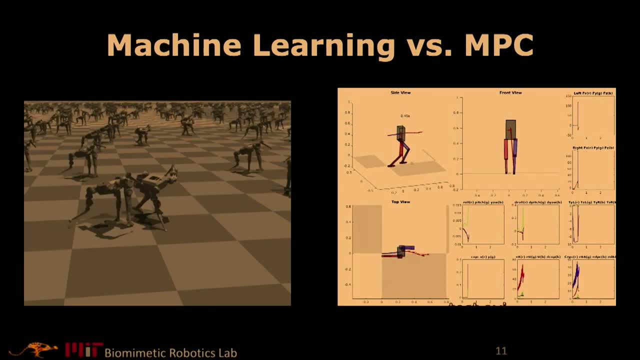 I know the majority of the communities are already doing end-to-end and then starting to do end-to-end. I know the majority of the communities are already doing end-to-end and then starting to do end-to-end. stop asking question. We had an experience with end-to-end. It's not good for mental. 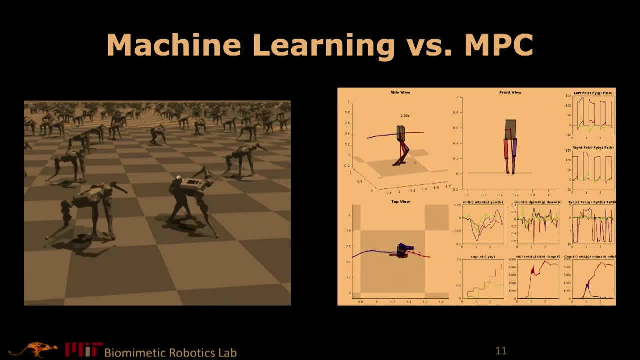 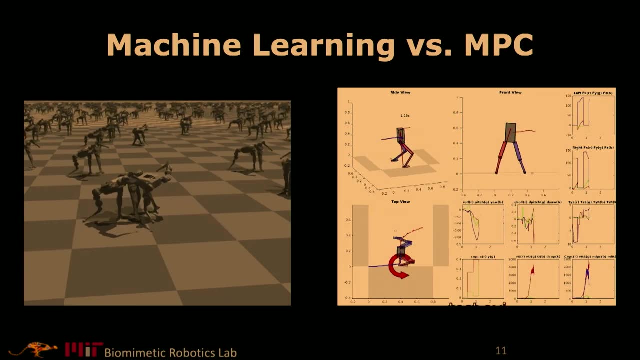 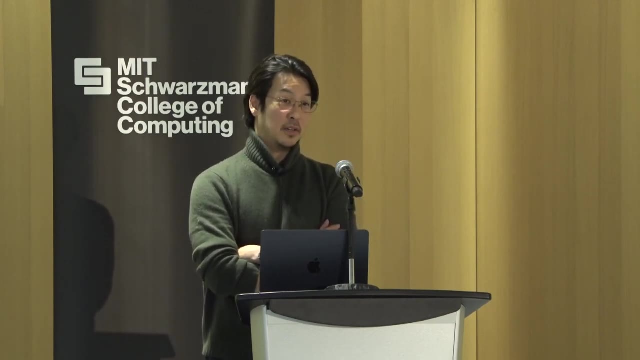 health of our grad student And we, when you hit the bottle, when you hit the progress plateau, nobody know what to do. It's not: all research lab companies are doing exactly the same thing. I'm not saying that that doesn't happen to machine learning, the MPC, All these. 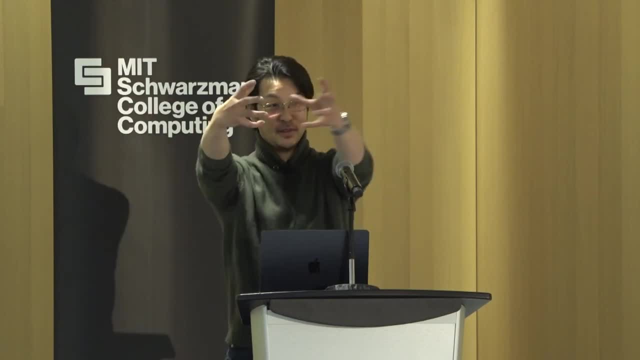 companies are put together- heuristic, with the compartmental machine learning MPC, They hit this, the progress bottleneck as well, plateau as well. Boston Dynamics hit that too, using all heuristics. So I'm not saying like one is dominating another, but the problem. 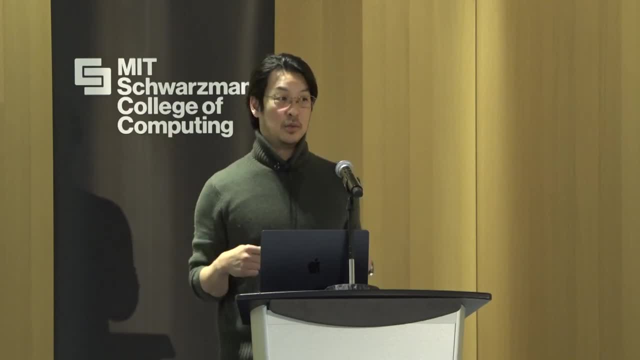 is when you have some problem. can you diagnose it, Can you understand why it does it, Can you reason about it. So, but we don't want to lose the end-to-end, like the versatility and then coverage, domain randomization and so on. So we are actually trying to shove. 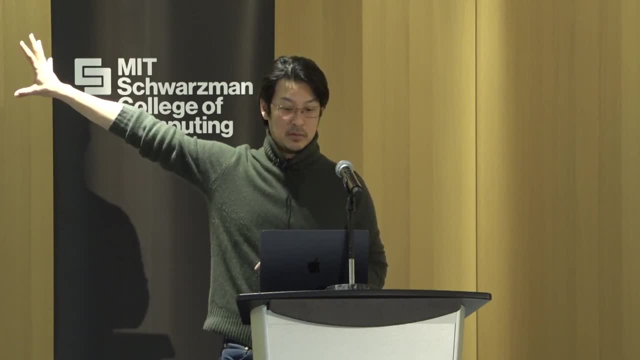 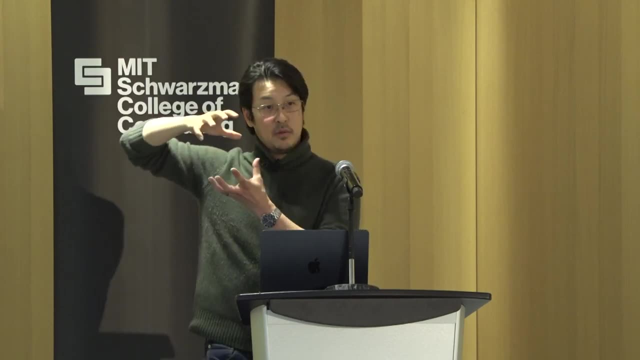 this, by the way, the right side is MPC is very fragile but very listening, very well, but fragile. very powerful, but doesn't listen, doesn't know how to talk to us. We're trying to carefully push this model in the middle of the machine learning, without breaking this. 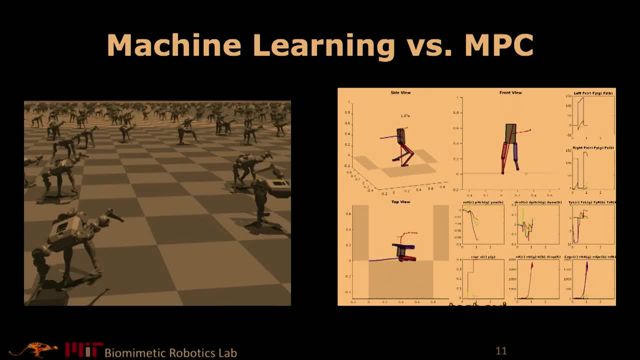 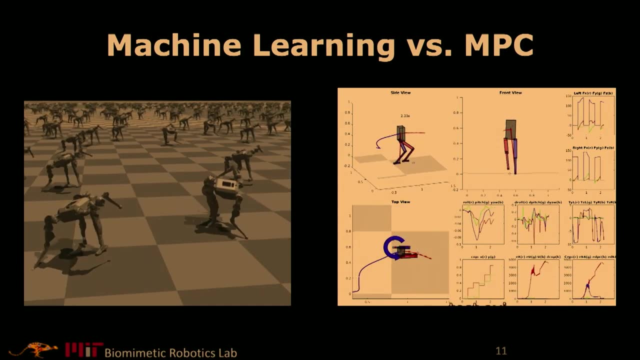 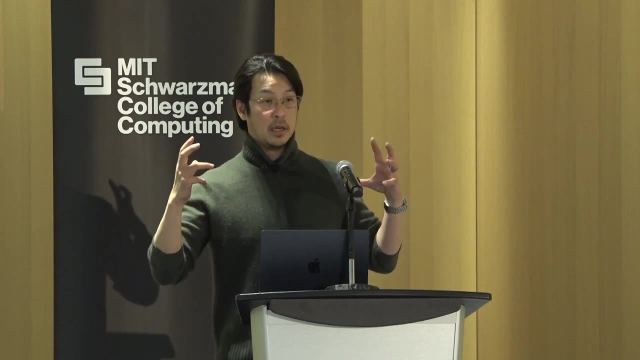 end-to-end. So like some sort of like a guidance. There's many papers having same, similar uh architecture but we're still trying to better, have a better architecture so that the tuning of those cost functions and all these parameter, meta parameters are actually um is healthy. 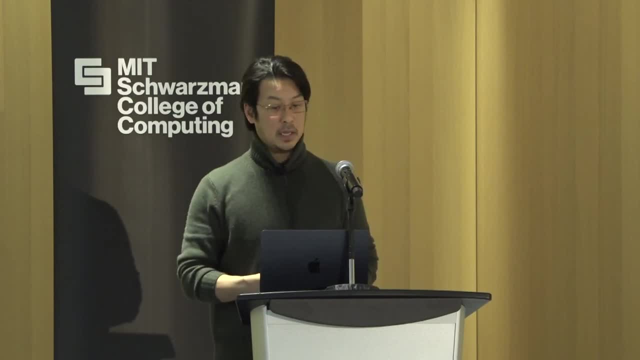 It's, it's give us intuition makes sense Because, at the end of the day, you're going to hit this performance plateau. If you, if your performance plateau plateau is not 99.9 after 10.9, you're stuck. I actually believe that Tesla- I heard Tesla hit that very close. 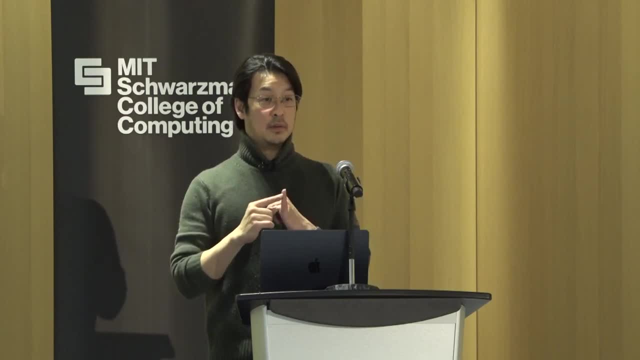 to that. I believe all these uh conventional, uh autonomous driving car company, um Waymo Cruze, already had an issue. All these companies already hit the plateau long time ago and then they don't know what to do anymore. So I think having models still, especially this. 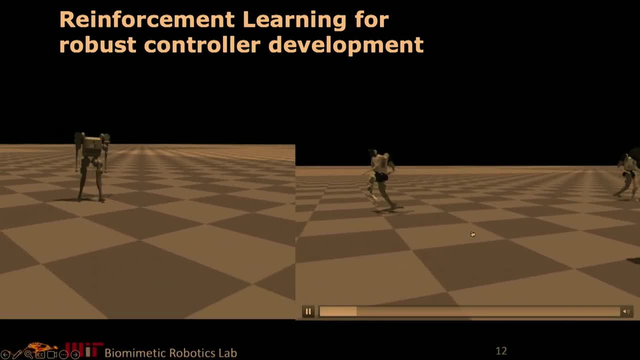 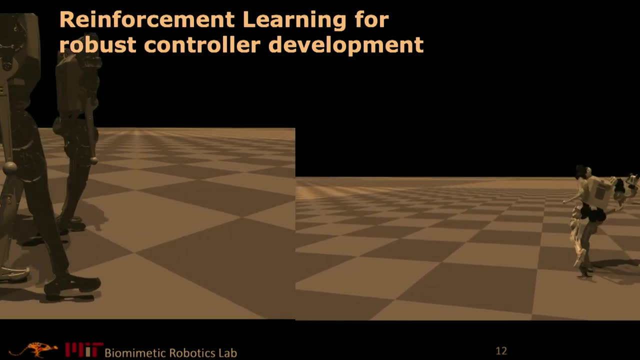 kind of application is so critical. I mean this kind of like performance. it takes like a week. We did that like a years ago- and then my students just do end-to-end in a week. The problem is, that's not all we need to do. We want to do it way more Every time you. 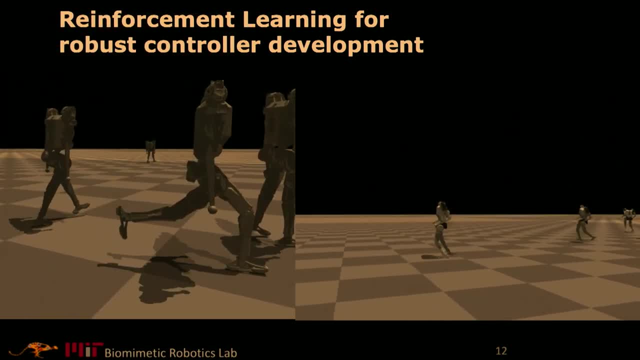 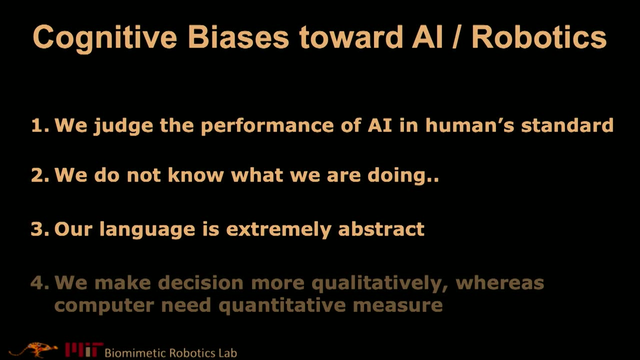 try to change something, Something else break down. we have absolutely no idea. So, um, I know you guys like seeing so many examples where like, oh, we don't need to understand. That is true for the digital world As, if you remember, my talk is about physical intelligence, where we have absolutely 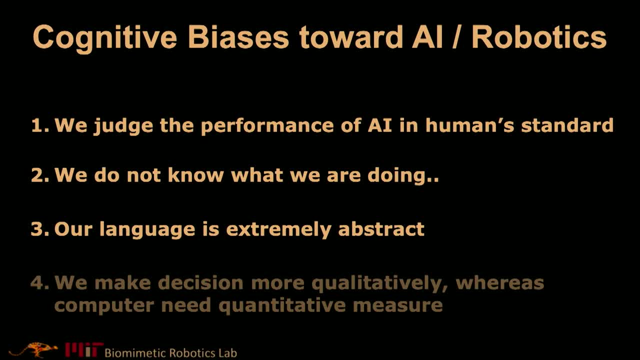 no idea how to collect all this possible data point. If you think about gold chests, even including all these texts in the world, we know how to collect all of them. In physical world we don't even know how to even start thinking about it. I know there's. 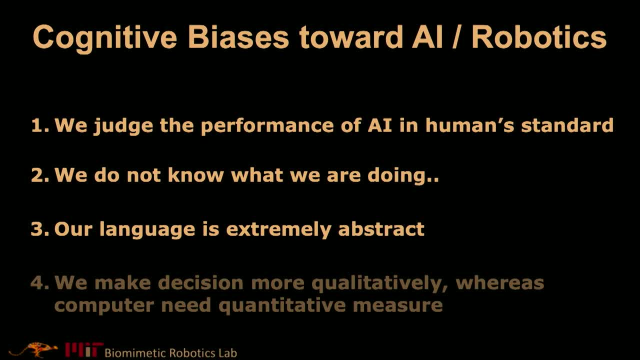 some people started thinking about it in Berkeley and so on. Uh, it doesn't look, uh, doesn't look that promising. And I'll explain why. we are misleaded, misled by all these results, because of these biases. So I'm not, I'm not sure if I can talk about all these biases. 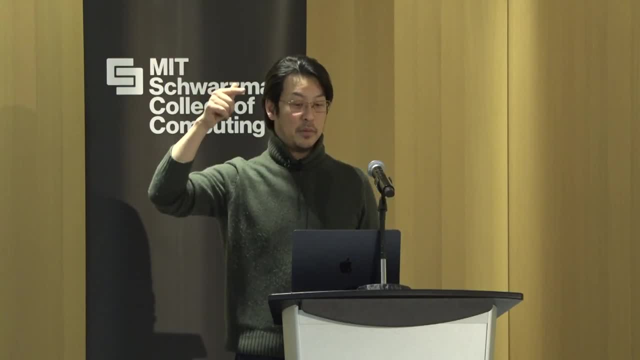 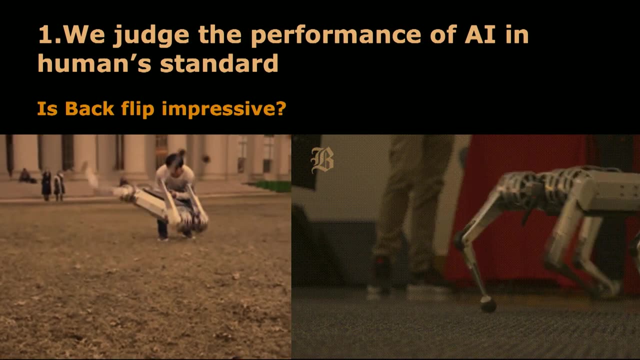 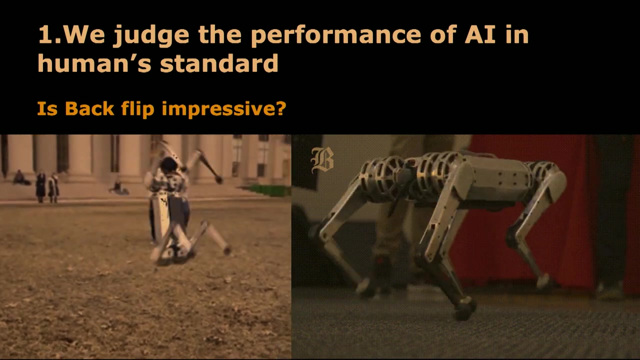 but I'll go through one by one. Number one: we judge performance of AI or any any autonomous system in a human standard. What do you think If I just collect your eye gauging algorithm? and then I'm pretty sure 70%, 75%, either on the left, and then that's where everybody's like whoa, Wow. 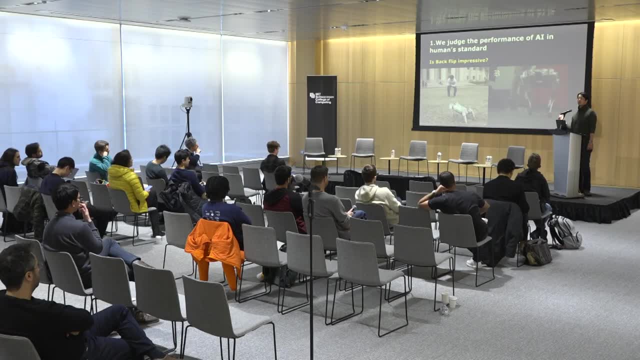 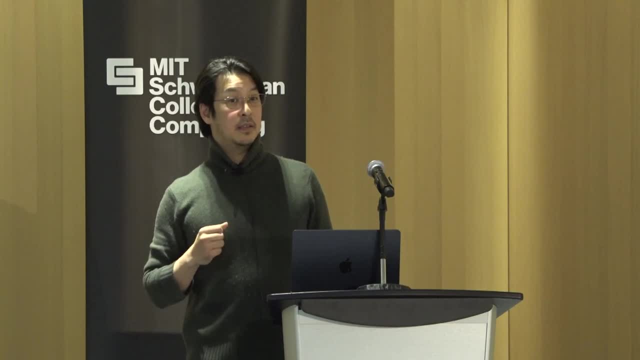 Impressive Guess what. How long do you think it takes to develop that algorithm on the left versus right side? I'll? I'll ask like, oh, just throw random numbers ratio. I have 10,, 100, or then you have to tell me which side is higher. 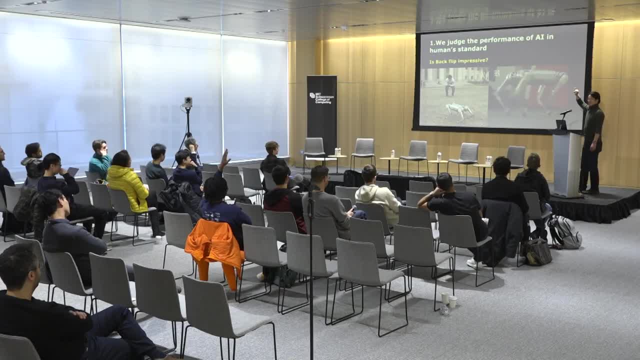 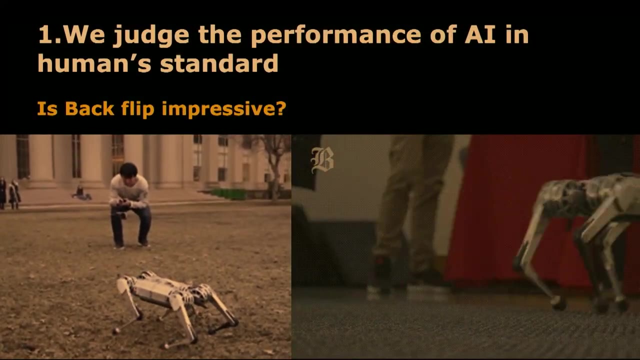 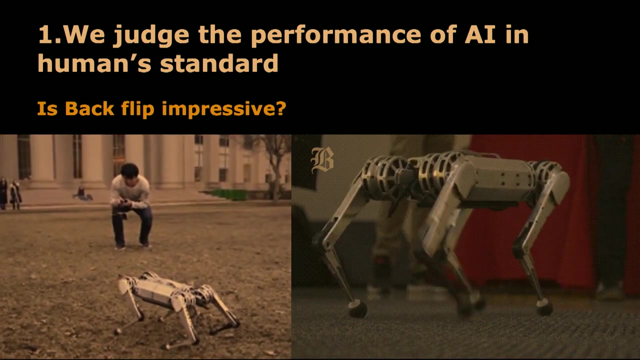 Tell me, Yes, Did you take my class managers? Anyway, that took about a week. from two undergrad class Europe, This one take whole team about ten student, about two years. And then, if you really think about why, when you see any AI performance, 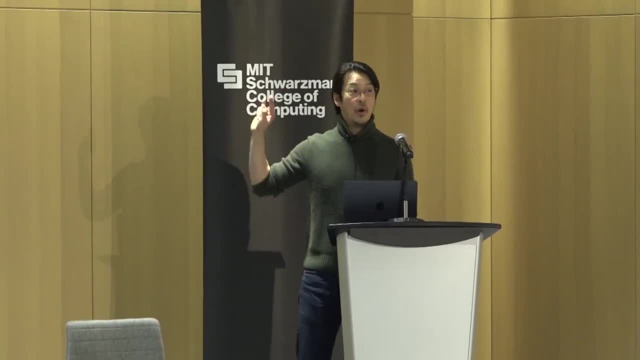 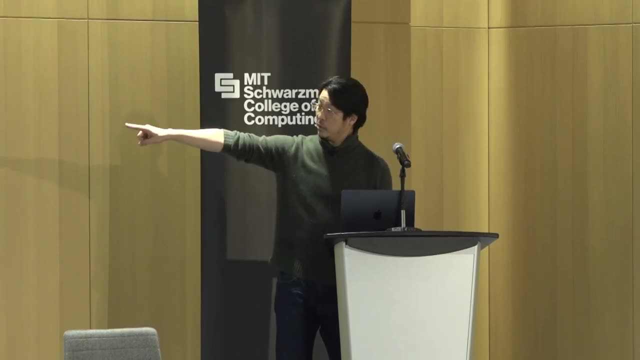 then you see robot doing something. oh, dish washing work. If you think about what kind of performance are those is hugely different. I want you at least to remember that after today's lecture, Most of the time on the left your robot is in the air. 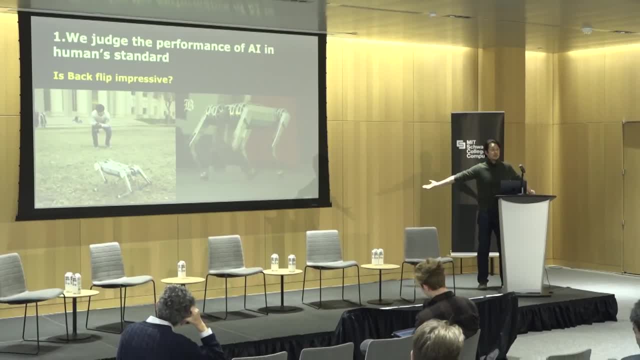 What are you going to do? I don't have fan or wing, right. What are you going to do? You're just feed for torque and then you, just as long as you have a good feed for torque, you're, you're going to be. 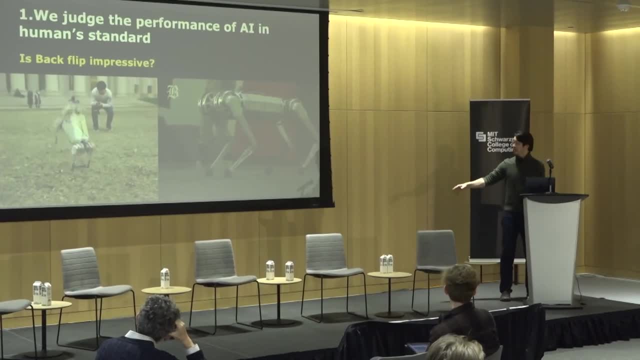 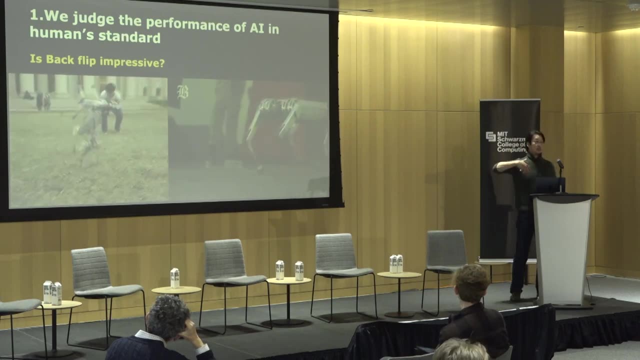 And You might have some controller landing which is simple as a PD control. Here, every thousandth of a second you have to monitor your state And then you need to solve your QP or some machine learning solver to maximize your stability. 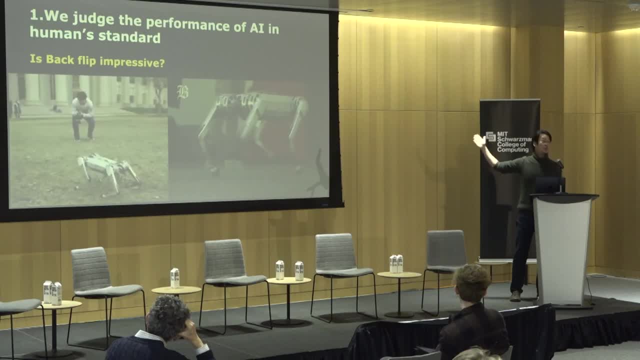 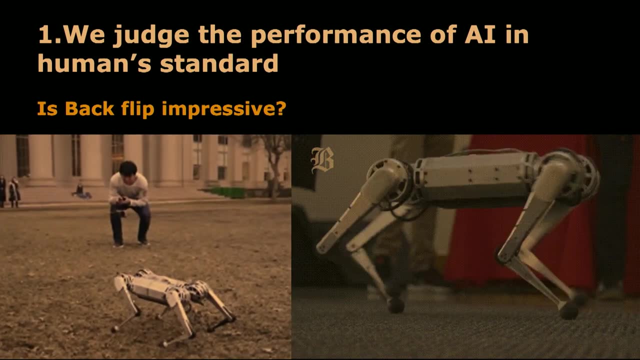 Seemingly it doesn't look that interesting, but that's going on, no matter what. If you pushed or not, QP's running a thousand times in a second, Or this time it's actually much less. But you know, it's constantly monitoring stability. 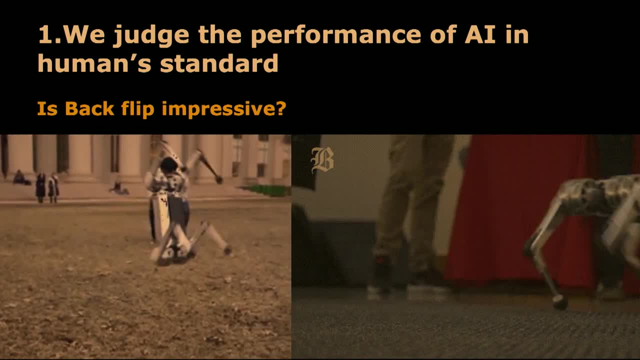 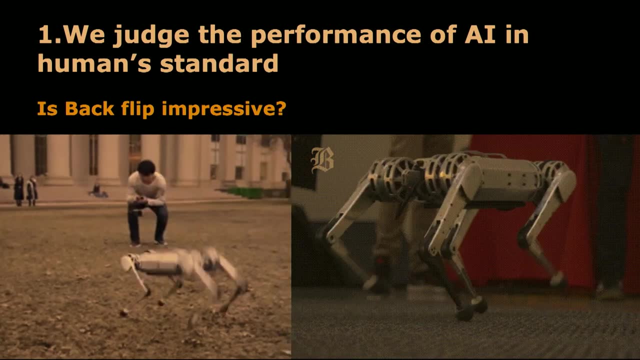 There's a stability issue. There's no real stability issue there. How are you going to define stability on that? If you throw in the traditional control theory perspective, there's no even steady state. Maybe you can talk about landing only, but back flip by itself. 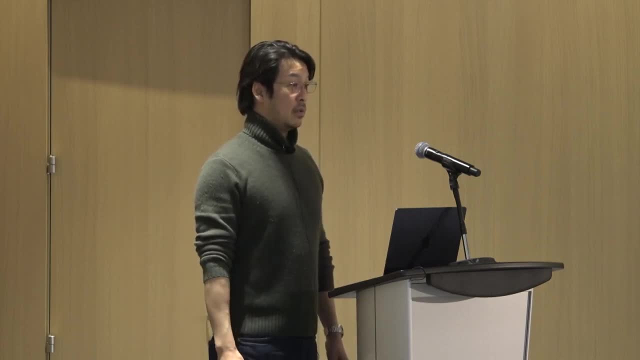 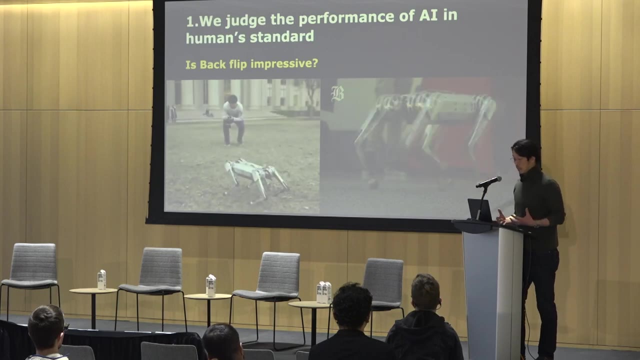 you can't even define standard theory in there Here it's also very, very hard, but at least we can linearize around that point and then we can talk about stability, Which has a lot of limitation, by the way, but at least. 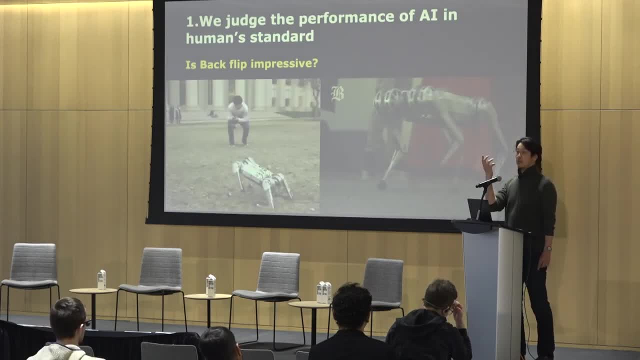 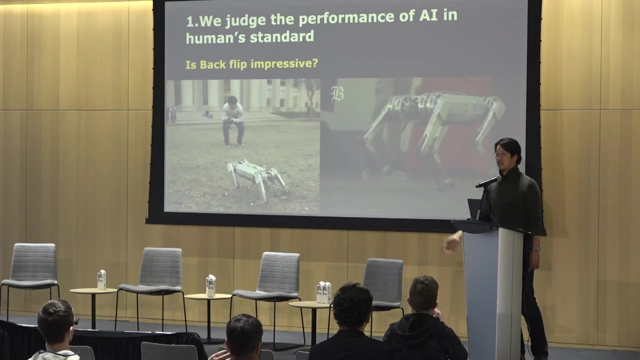 this is my explanation of what I'm saying. So our quick judgment, our reflex power of our brain, which is actually dominating your daily life? by the way, you have a machine learning algorithm and firing answering your solution in a second every hour. 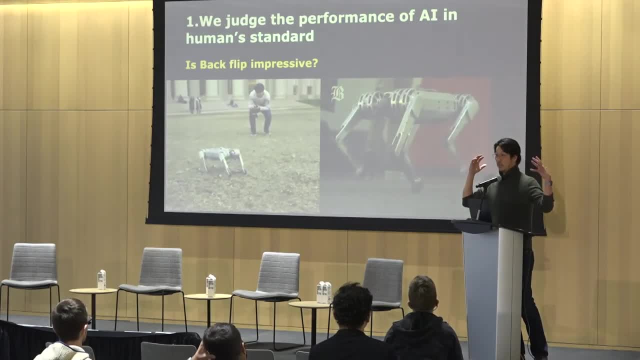 every maybe less than 10 minute a day, And you're relying on that by majority of time. Yes, sometimes I need to think about it. Do you remember the moment? oh, wait a second, I need to think about it, right. 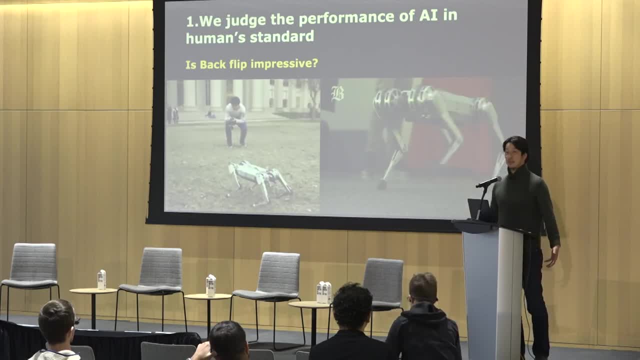 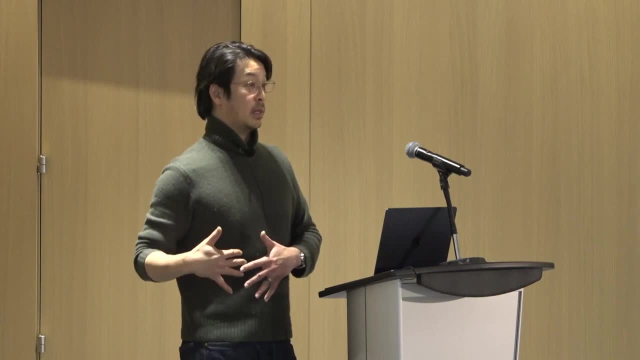 I left my wallet doing this and after that, oh, I need to think about it. right, But if you think about how many times you make decisions based on the reflexive action, brain action versus- oh, I need to think about it- where your 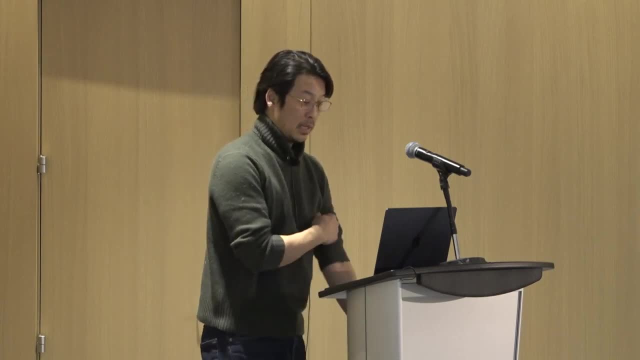 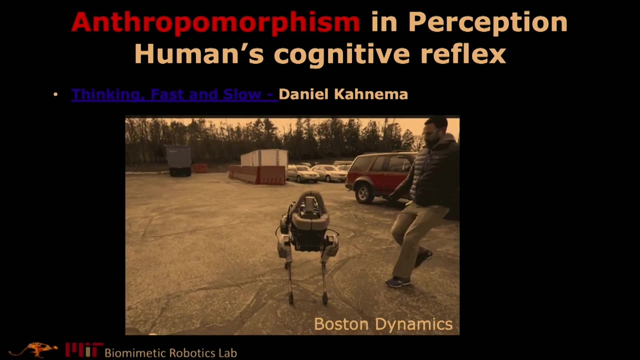 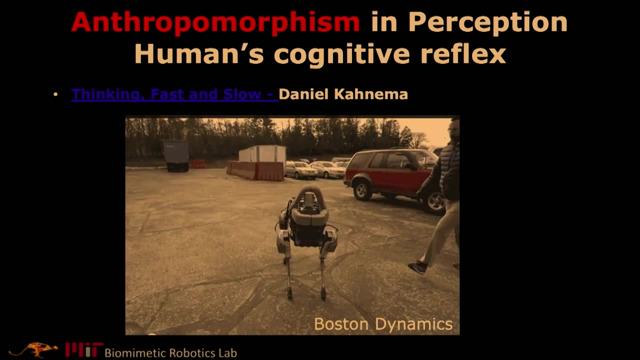 actual brain goes to logical and the reasoning part of it and searching for memories. I'm actually modeling this, by the way, so if you're interested I can talk about it. Another example: I'm not sure if you've seen this video's comment. after this, Anybody saw comments on this video. 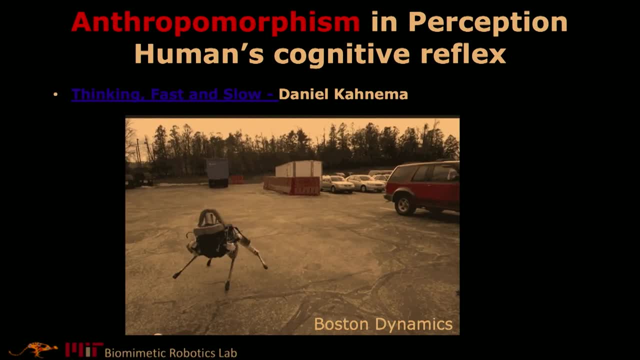 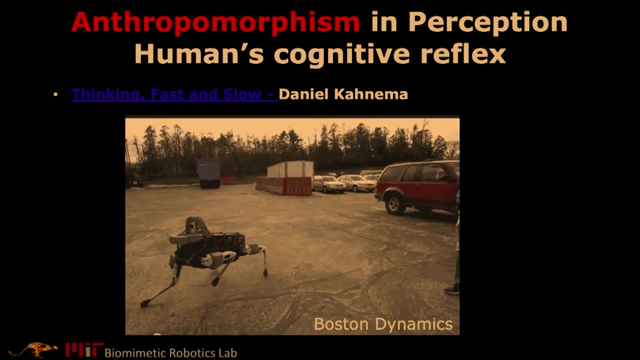 This is a very old video, by the way. You can find at least 40% of comments are like: you're going to be the first person killed by the Cyberdyne when robot took over. Oh my god, you're so mean. how do you do that? 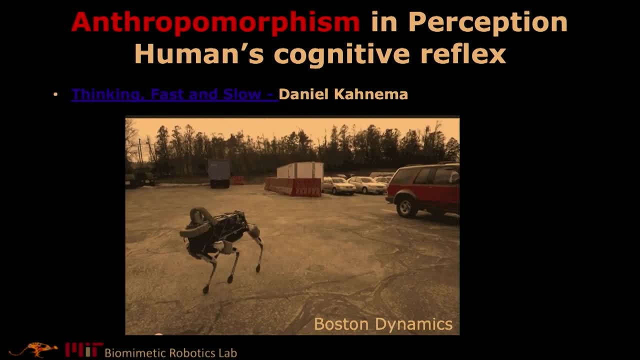 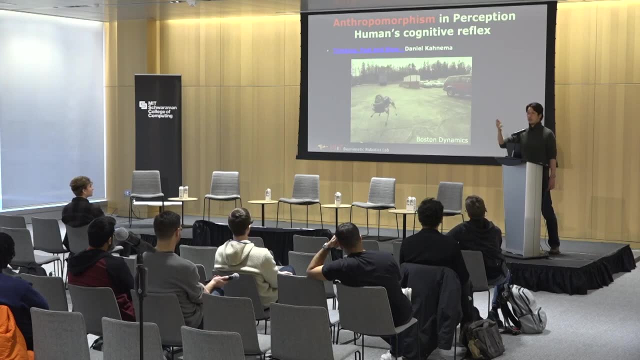 Whoever is not roboticists or not familiar, they will say something like that. I guarantee you anybody who's seen this many, many times saw playing with the robot all the time- like people in my lab who play with the robot all the time- 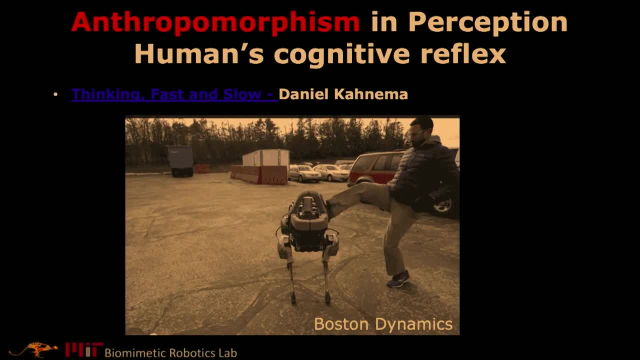 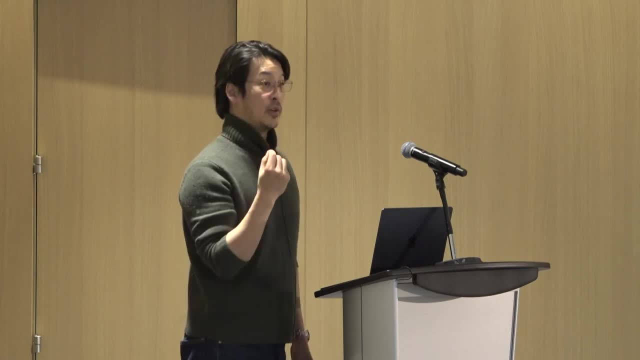 Well, as soon as I showed this video, within a second in your brain: ooh, that was a grab. Why? Because it's a reflex You can't have, you have no control over that part of your brain And of course we think about: oh, that guy was very aggressive. 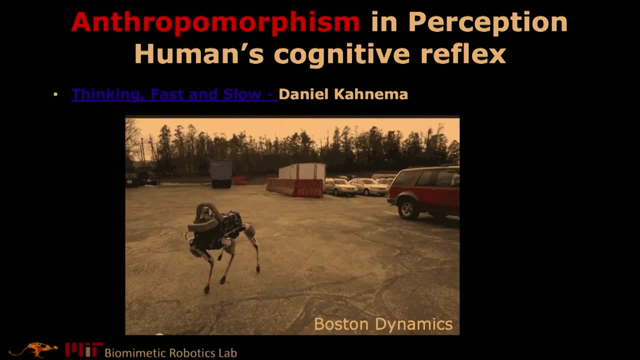 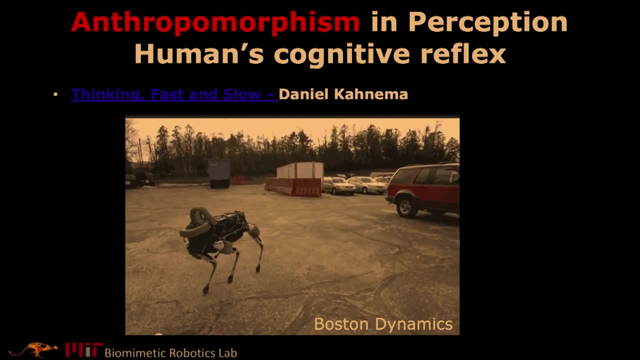 because he has to be aggressive, But there's no judgment, Like, of course, somebody might not even know, that's control algorithm. but human brain is wired because we're still animal. We have to judge quickly to survive in the mountain. 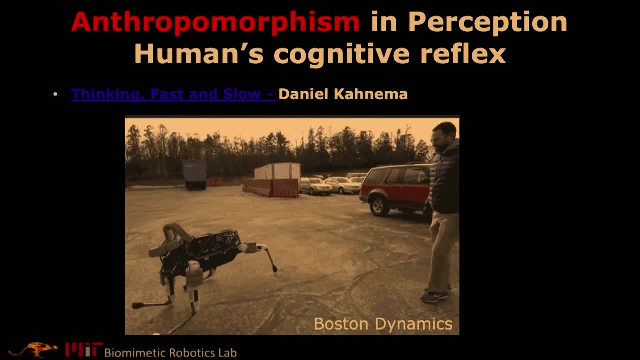 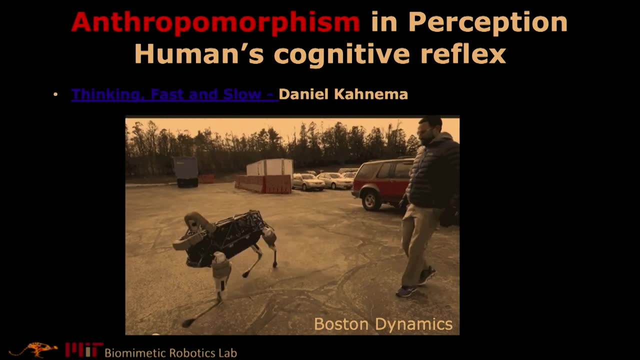 Imagine you're in the mountain and then you saw the bear running toward you 30 mile per hour and like, wait a second, let me judge how far it is. And then, hmm, comparing with the trees, that's about one meter and a half tall. I have to calculate that's about 400. 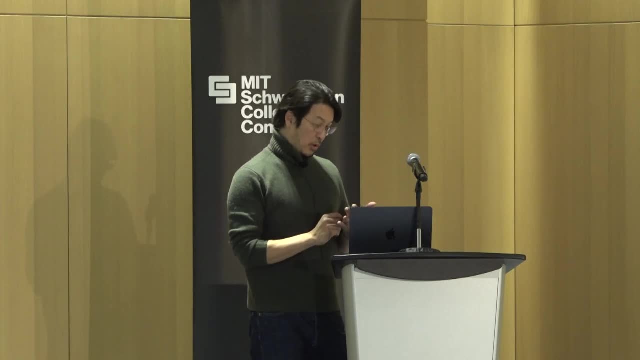 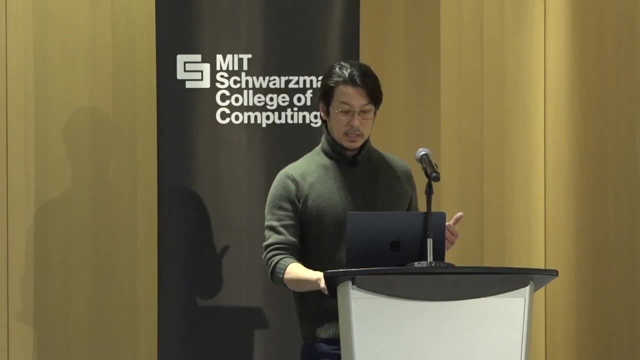 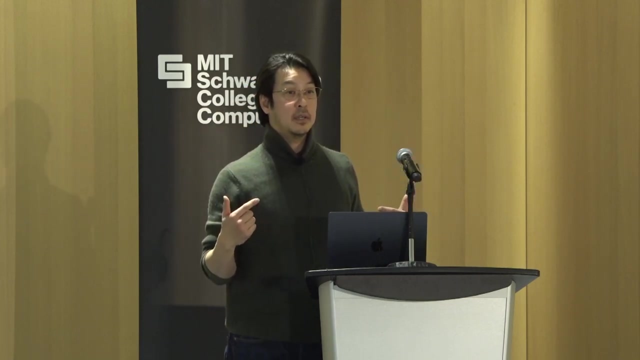 kilogram, running 30 mile per hour, Half times m v squared. there's no time for that. See something aggressive, you'll run away right. This is all relying on human reflexes, which is based on trained, based on human interaction. I saw a robot. 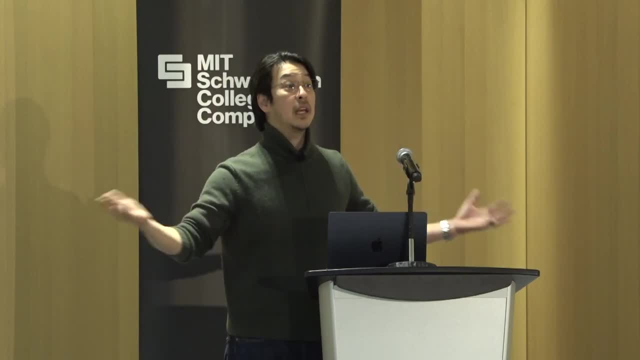 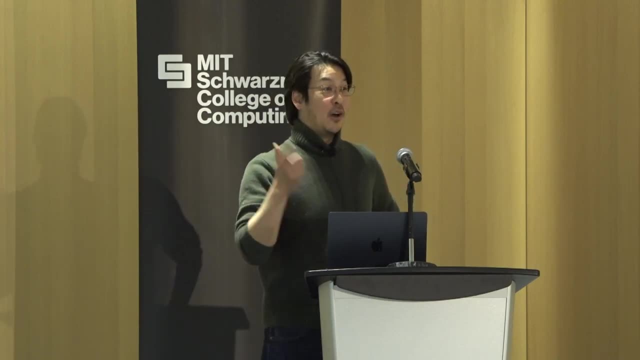 back. oh my god, that robot is so agile, you should be able to run. you should be able to run and walk. It cannot even make a step to stabilize. If you see a person back flip on the street, no doubt right, Would you doubt that? oh that person? I don't know if. 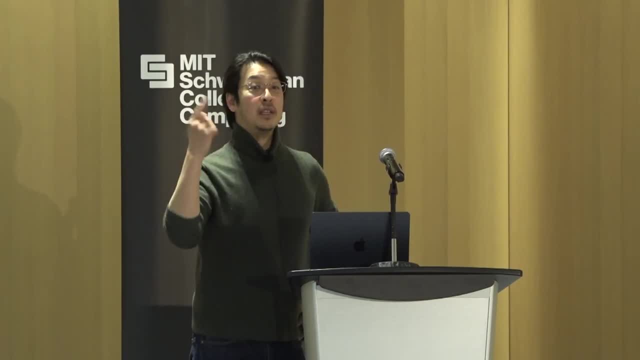 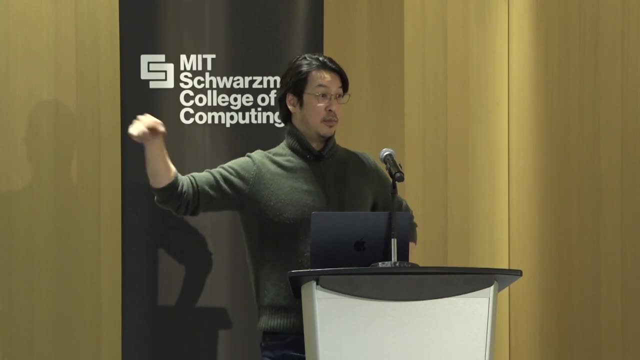 that person can walk. Your brains are trained based on human interaction, human function, but you are still using that part of brain when you judge a robot, as I show you in the back flip. That is happening constantly. I don't want to well. 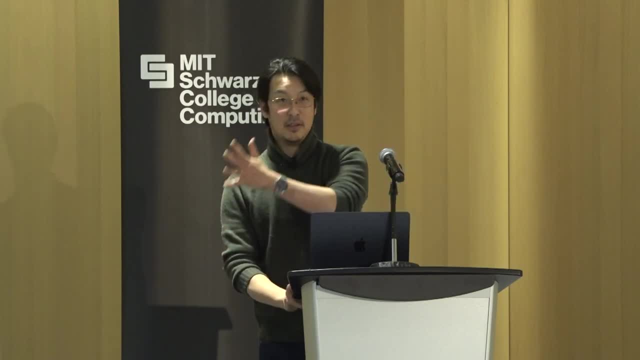 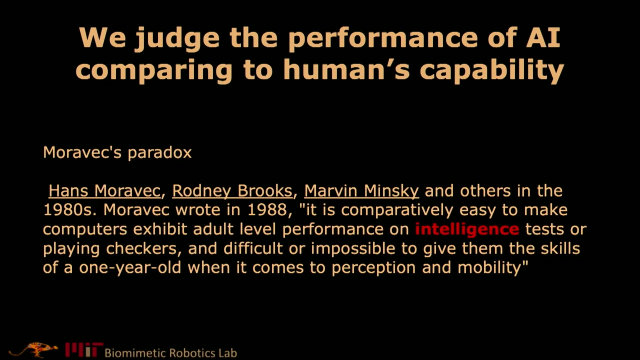 I'll say it: TRI: imitation learning, Berkeley, Stanford imitation learning. wow it does that? Just take a moment and override your reflex. One thing I want you to remember today: override your reflex, because that's how brain works, Even this. 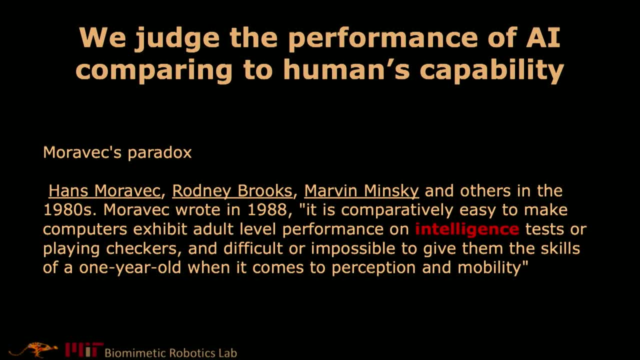 renowned professor at 80s, actually says that, oh Moravec's paradox. like seemingly difficult adult intelligent tasks were very easy, but like it's very hard to do perception of mobility than a one year old. Even they, though, who actually introduced? 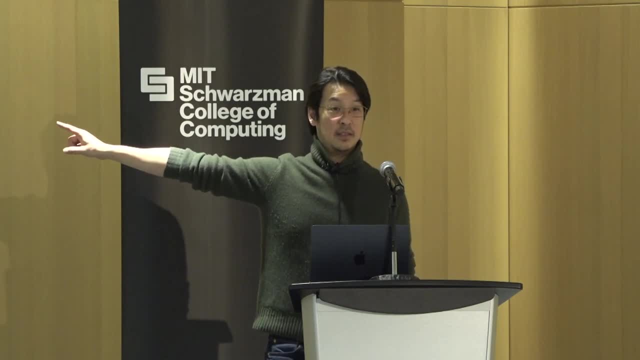 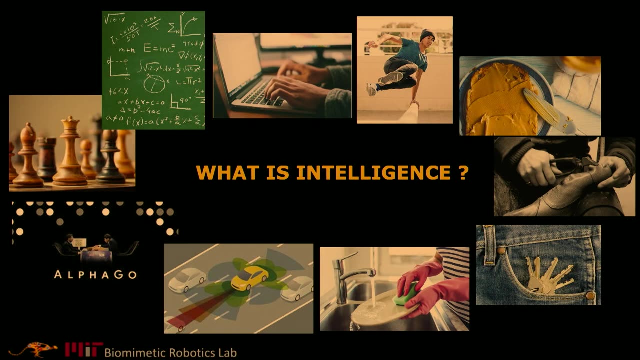 that concept. use word intelligence test for checkers. They are also biased because they think that's intelligent. One year old, walking and playing with the object is not intelligent. Who are you to judge this? Have you sit down and think about what is? 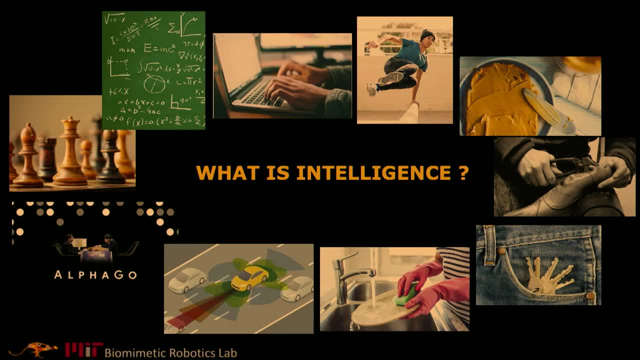 a fundamental of intelligence. If you look at that left, we call the smartest person in the world Whoever write. amazing philosophy book were so amazing. Being able to write or read was the was the criteria to decide that who are smart or not. And now look at that Almost. 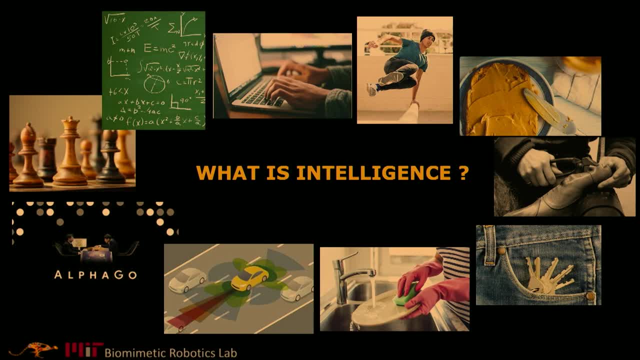 like a. it's hard to clear completely. Later. latter half that we thought is the only smart person can do is already all conquered by a data and very relatively simplistic algorithm. On the right people seemingly like: oh, that's too low for my job. 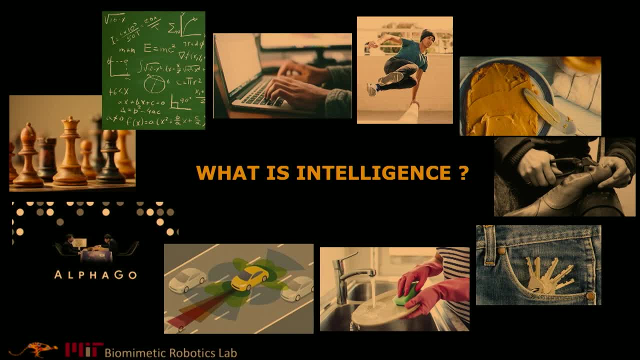 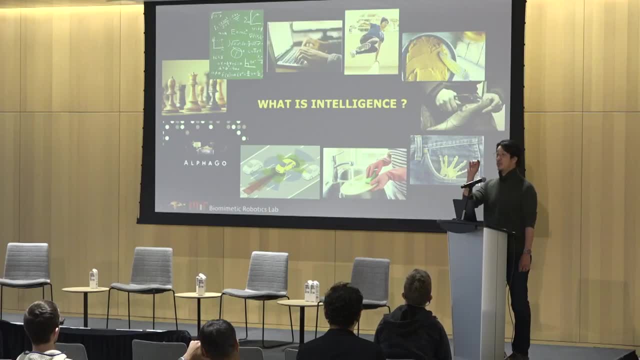 Oh my, my son can do it, My, my baby can do it. None of them even have a any conceivable a possibility to catch up. In a generalized sense, You can, of course. if you carve out that key on that pocket and that pens and that gripper, yeah, you can train and do imitation. 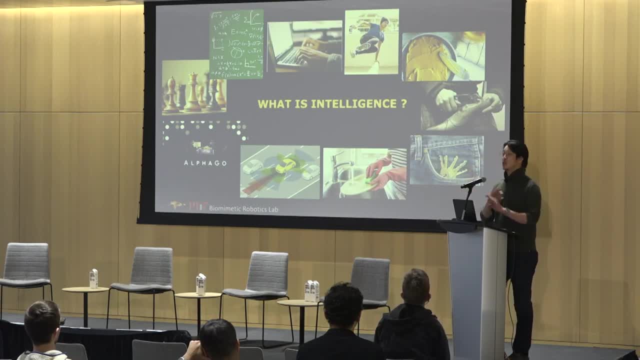 or you can do it. If you change one parameter there, it's going to fail because there's no generalization whatsoever. That's what I mean by physical intelligence. We have to be able to distinguish what is a virtual intelligence, which is all trained by, you know, the, the, the, the, the, the. 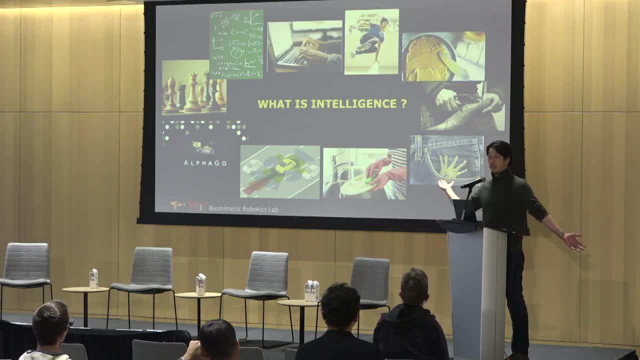 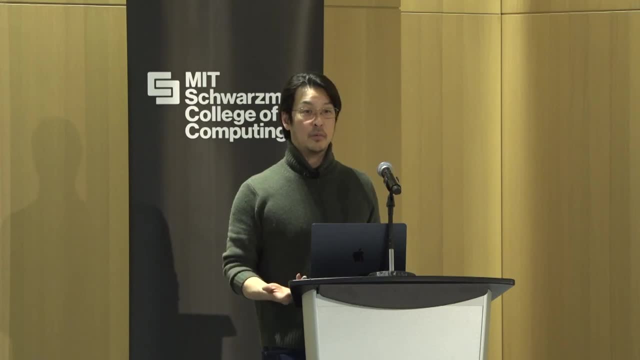 the intelligence which is all trained by the virtual data. It's all available in the web. Whoever have the money, you can just collect them and train. Whereas physical intelligence- what robot you are going to train from? to begin with? how many sensors? 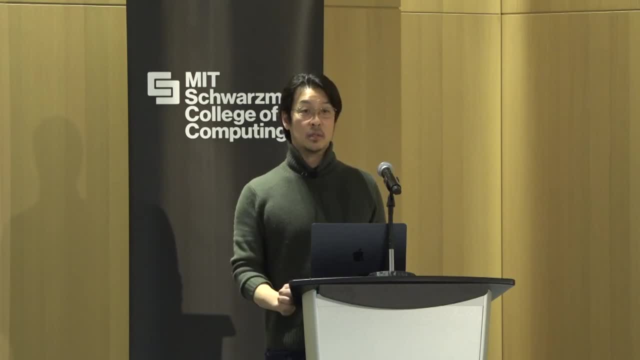 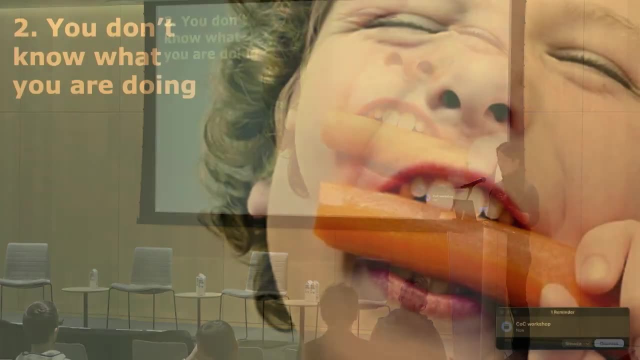 I'm going to have how many fingers are going toDoes. anybody have any idea how to start with? Second, you don't know anything about what you're doing. I will ask anybody: eat lunch today. Raise your hand, Okay. 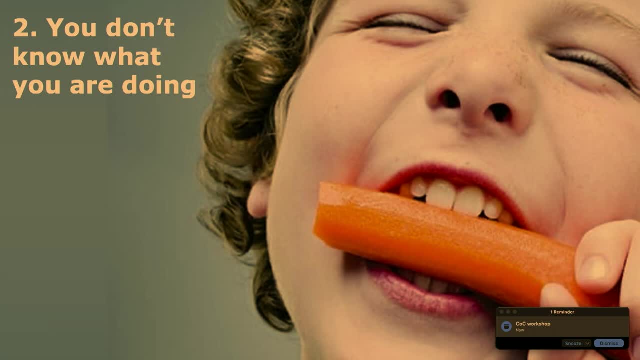 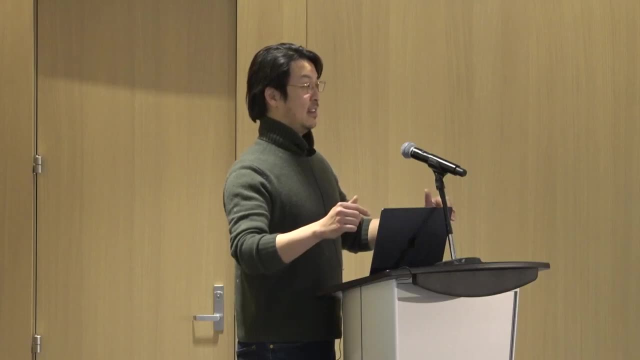 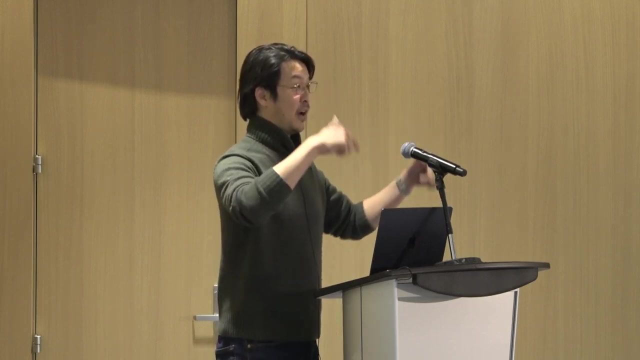 Okay, Do you remember what you ate? Sometimes you don't remember what you ate. Let's say you ate a bite of carrot. Have you thought about eating as a robotic process? What kind of policy you have to train to actually reliably chew carrot and? 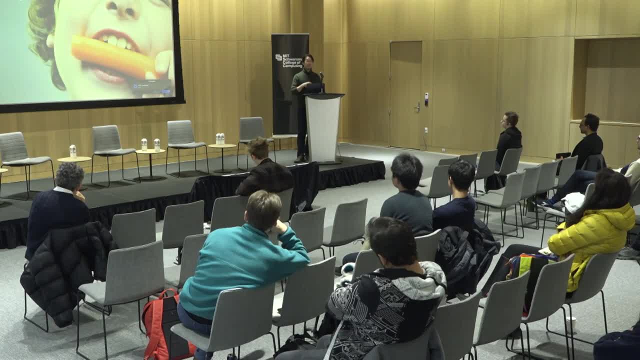 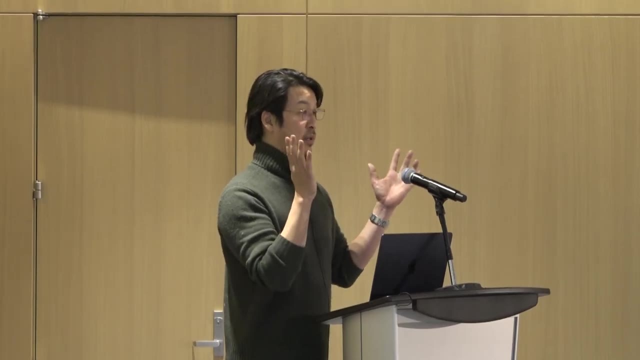 then swallow so that your chopped out carrots are in your stomach and broken down by acid. How would you know how finely you have to chop down? Any of you, by any chance, can control independently- control your individual teeth. It's gruesome to even think about it, right? 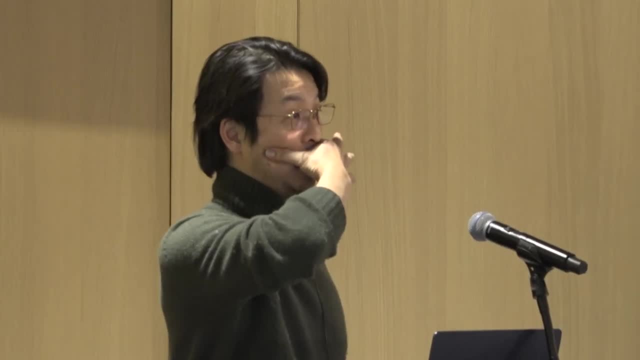 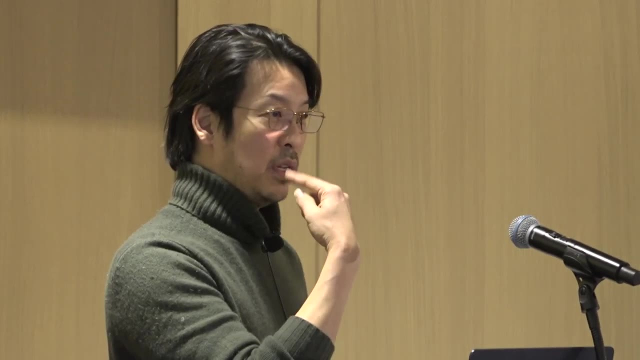 You have one chin and there's one rigid body on top And somehow carrot comes in and then it all dissolve and then go to your stomach. What happened? I have a grinder or something in my mouth. No, I'm talking right now, right? 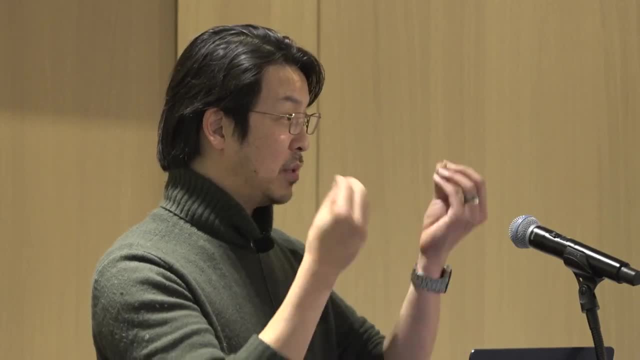 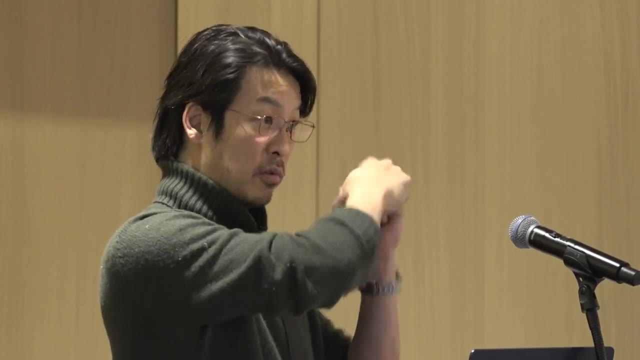 Because I need to have a tongue in the middle. How come those get chopped down? Think about it. Food comes in. I chop down it to a certain size. My teeth are broken, My tongue pushed to the cheek side, And then your molar crushed down and then broke into multiple pieces. 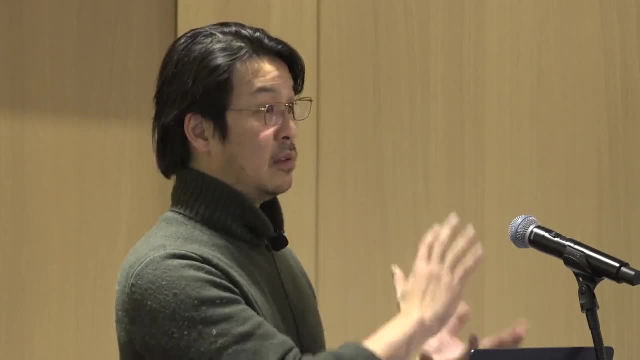 It's small enough you can swallow. Big enough. I had to push back again, crush down again. And while you're talking with your friend right, Most of the time when you talk, what do you use to? to talk? 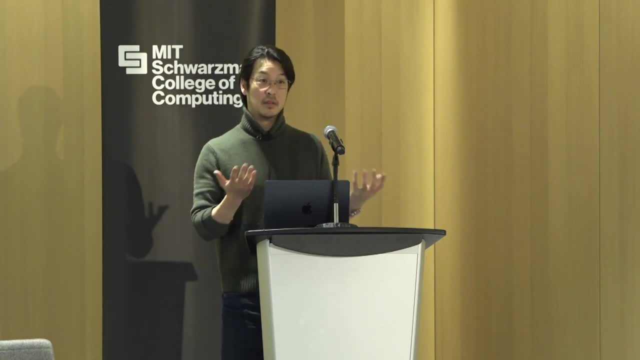 Tongue right, Of course, your lips and everything but tongue is essential. You cannot talk without tongue right While you're eating. are you aware of any of this action, of a fraction of this action, when you're doing it? 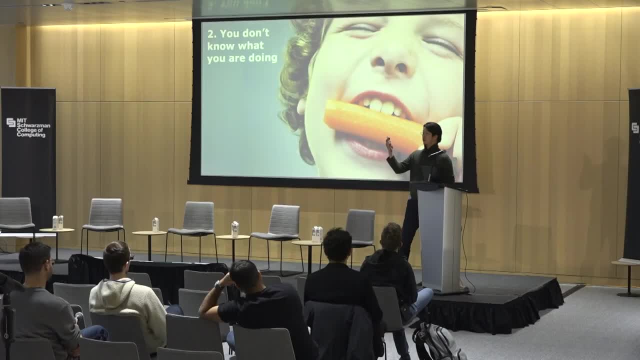 I can give you an example. Can you bring? Can you bring something from your pocket? I have some lip gloss. Can you try it? Try it, Pick up something from pocket. Pocket is actually is quite unstructured right. I don't know how LiDAR mapping help in the, in the in the pocket, right. 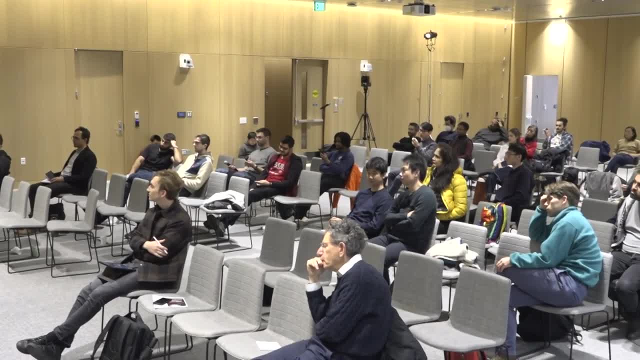 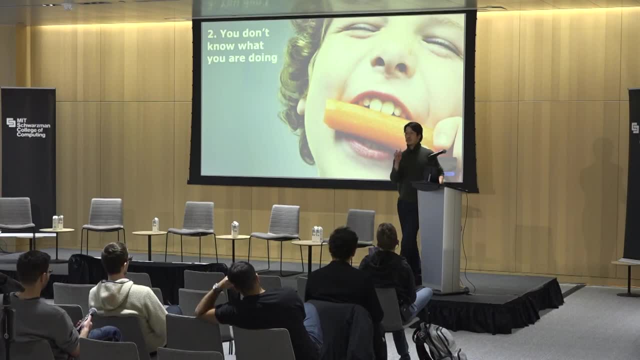 And then bring it up and show it on your face. Show it on your face. Okay, Do you remember a joint trajectory of your, a second segment of your index finger? I believe everyone used index finger. Anybody remember that trajectory? 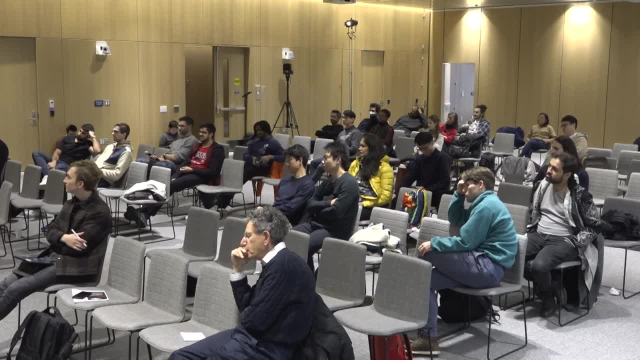 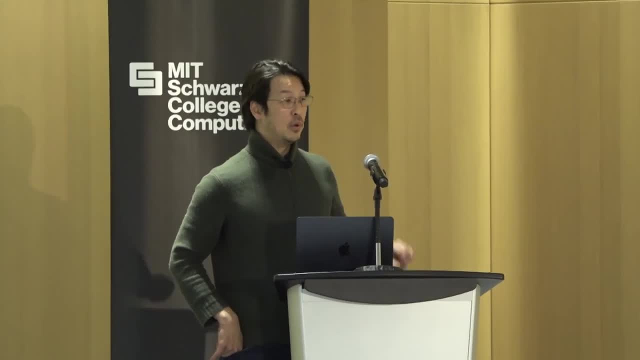 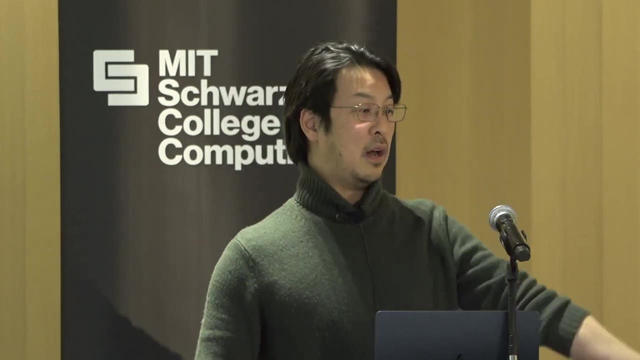 Did you command that? You have absolutely no idea how your body works, as I said about tongues, And how can you even judge a capability of something that you have absolutely no idea, Which happen all the time? You know chairman, president somewhere, and then that department sucks like fire them. 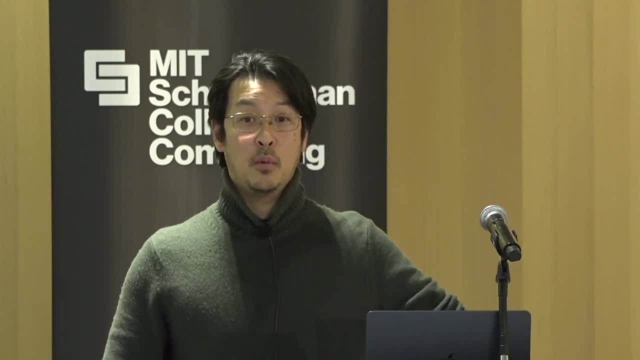 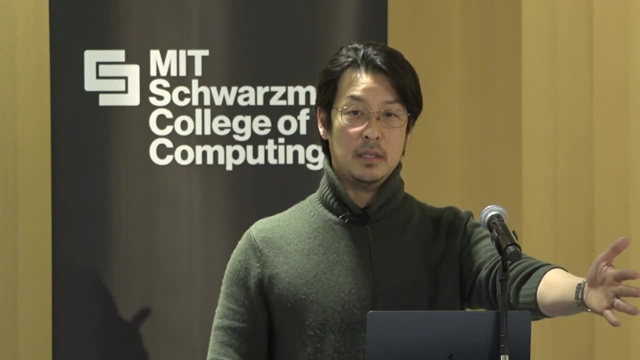 Like they don't even know how it works. but we judge all the time Why? Because it's so easy for us, It's so automatic for us when the robot does it. that's easy, But we don't. we don't even know how it works. 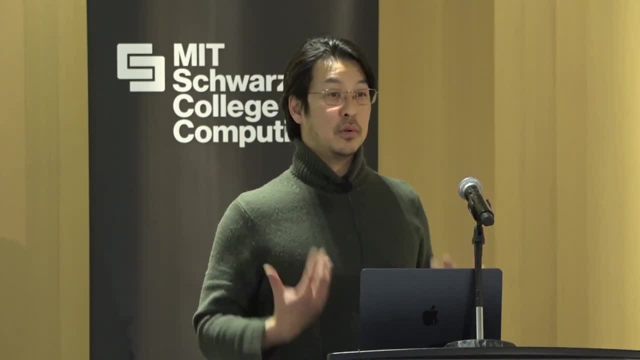 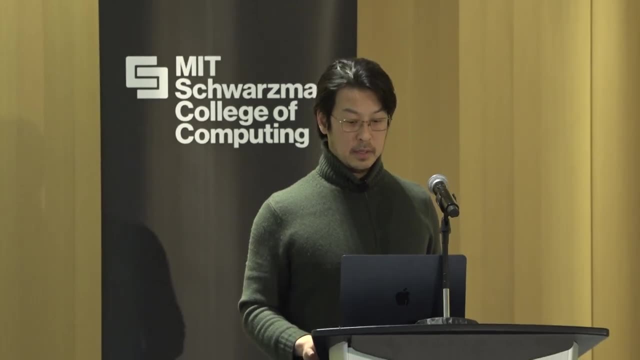 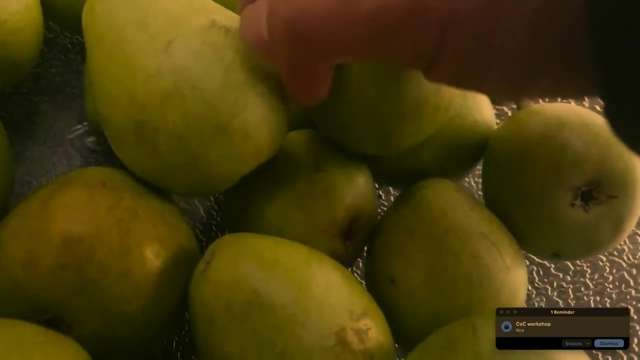 We have absolutely no idea. I searched for every possible neuroscience paper in literature. There's absolutely no understanding because very, very, very hard to even start studying. This is me picking this fruit And I intentionally do that without looking at it, And then it took about 0.7 second. 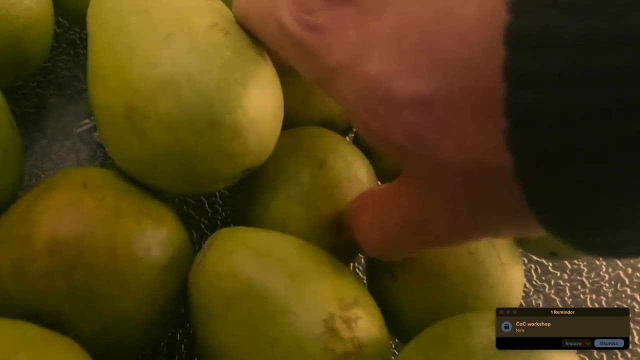 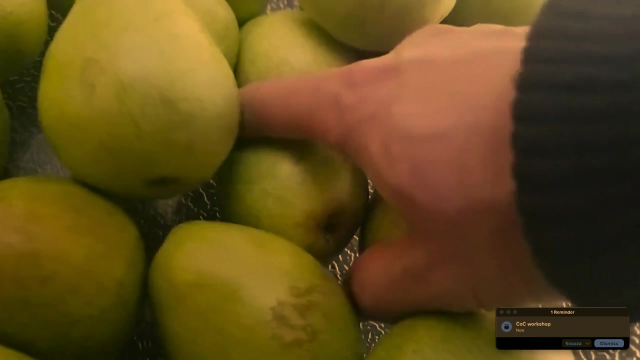 This is all that happened. I throw my hand. my hand collide with it, And then I tried to grasp it and I ended up pushing more fruits. And then I get in touch with the five fruits. I'll show you again: It collide. 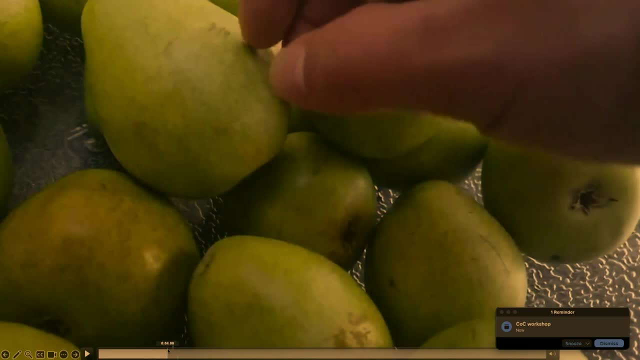 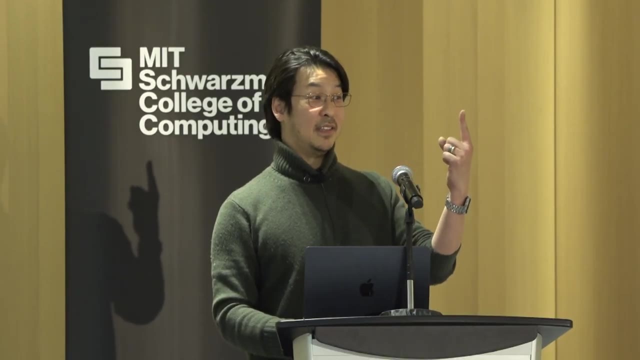 And then if you write an algorithm, somebody to come up with a cost function. but one of the cost functions should be easy to grab. Maybe the height might indicate that should be part of the cost function. right, I will probably pick up one of those, the highest one. 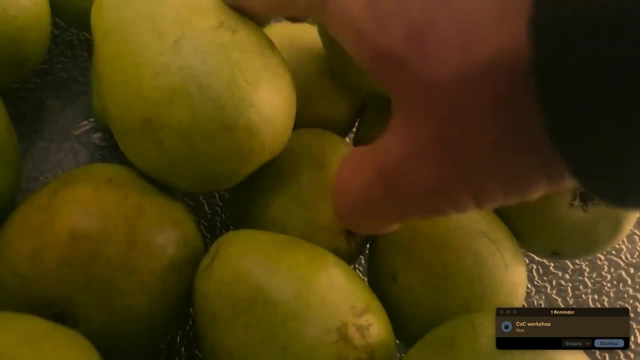 My hand algorithm said: just grab something. And then, while opening my hand, it pushed the most viable candidate And that by doing it, you ended up making more content. Ah, there's more option. And then, even here, if you write a control algorithm, 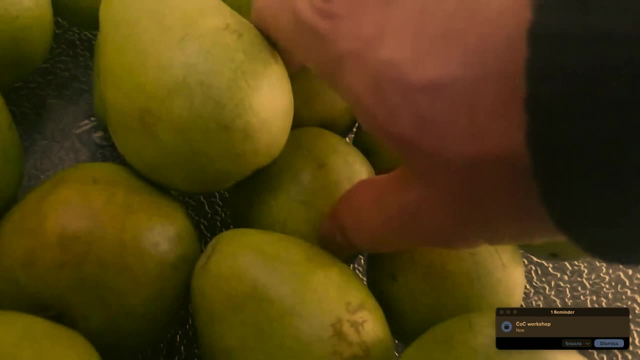 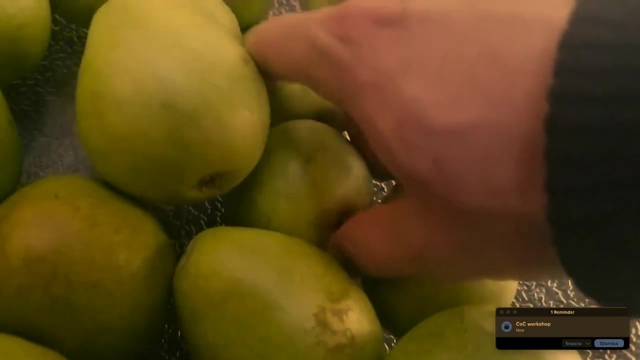 or optimization algorithm, base algorithm. you choose one of the top right. My arm was disappointingly much dumber than that And ended up choosing the worst possible choice, And you have to dig your finger through it, And then you still decide that. 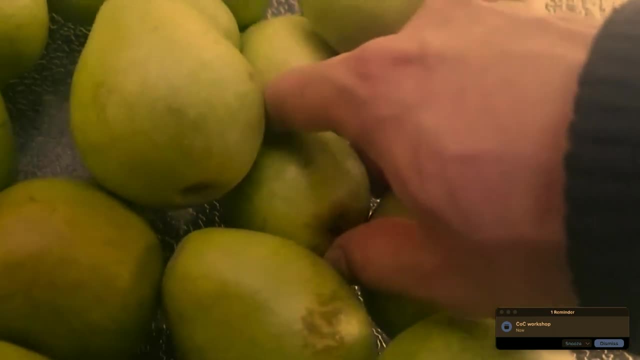 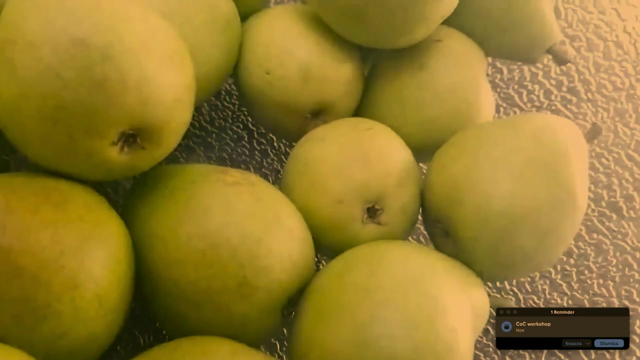 oh, I don't think I have a guarantee to have a firm grasp. You push even deeper And then successfully coming out. Do I remember any of these? Absolutely no idea. Try that at home. Just open the cover and then grab a cup. 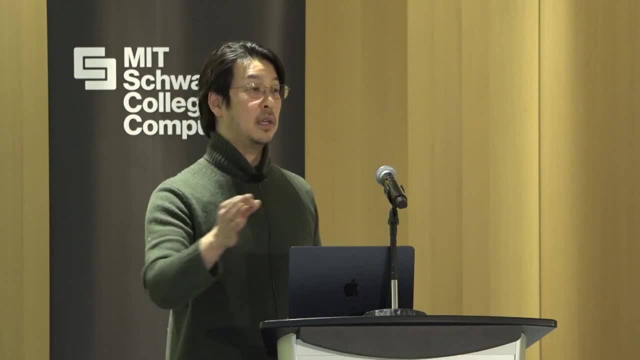 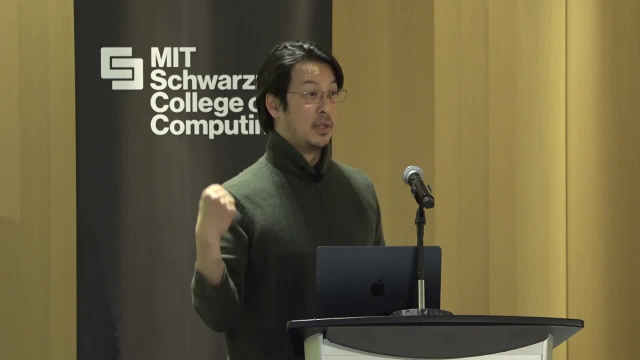 Do you remember any of this? Absolutely not. You have no idea. what kind of policy does this dumb thing but super reliable way? If you open your cover and then grab the cup out of it and close the door, what is the success rate? it will be there. 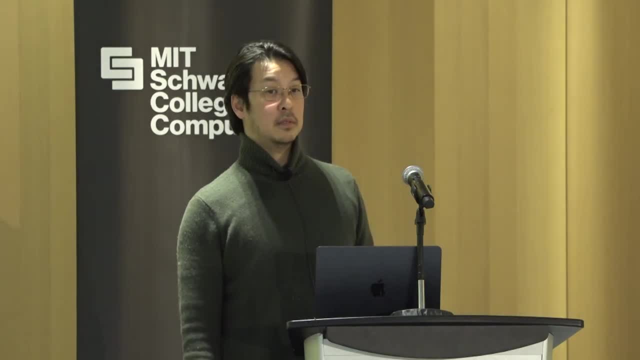 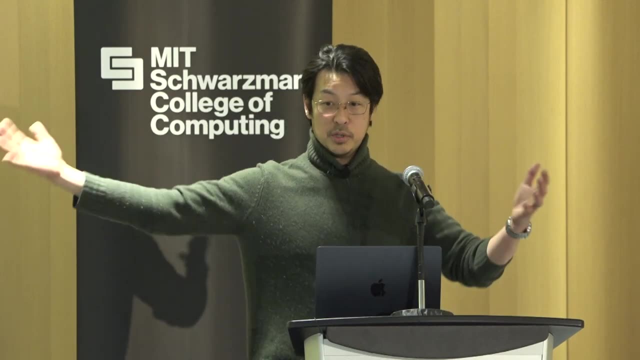 If you do that 10,000 times, what will be your success rate? Or this: move the apple, grab and push down a bushel like 10,000 bushel. What is your going to be success rate? I guarantee you it's going to be 100%. 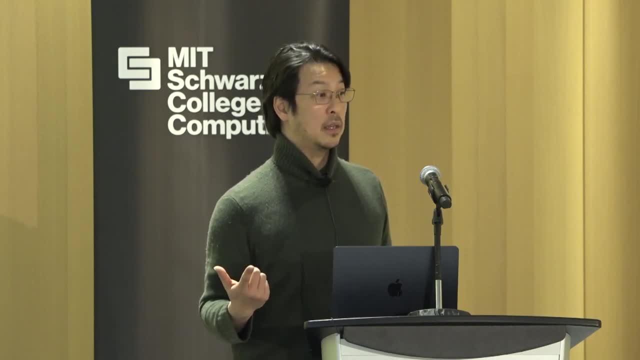 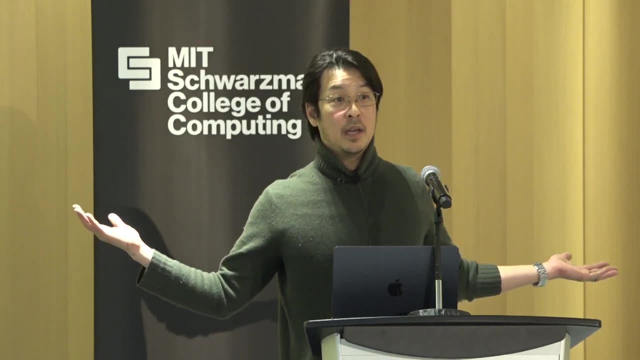 because even the failure you can recover from. that's a policy. I'm not imitating anything. There's a policy over policy over policy, Policy structure trees going on. I have no idea How can you judge things we don't even understand? 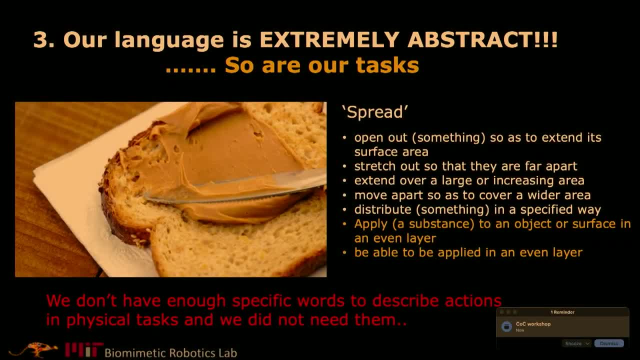 Language people. some people are lucky or lucky. I'm good, I'm weird, I'm insane, I'm shocked. like has to change the research direction, maybe lost jobs. some company collapsed after language LLM come out. It was a blast for me. 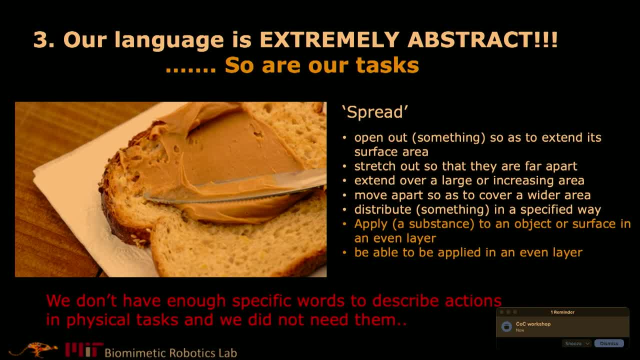 I've been trying to conceptualize what is physical intelligence, physical intelligence- And then I came out like, oh my God, so easy to define. now, Whatever LLM cannot do is a physical intelligence. They give me the draw, they give a boundary. 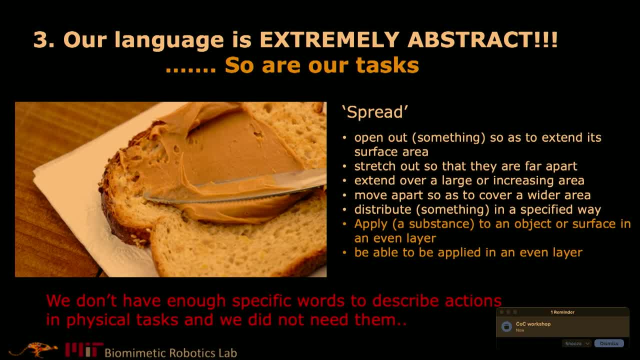 So easy, because language, if you really think about it, unless you go to the jargon jargon is like a carpentry jargon. They have their own language. We have no idea what they're talking about. Plumbers have their own jargon. 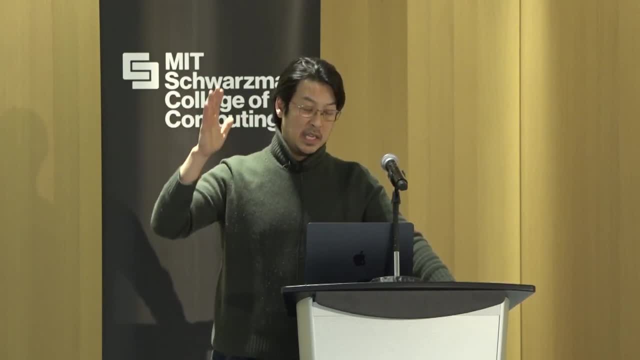 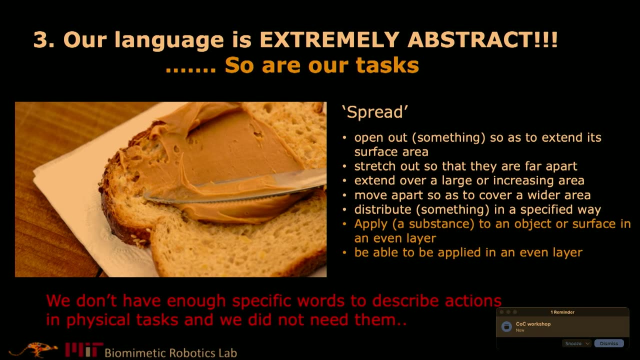 Let's stay out of it. I mean, LLM has all that jargon, but even those jargons are not detailed, have a high resolution enough that you can just plug in to make a robot work, because it misses all the nitty gritty. 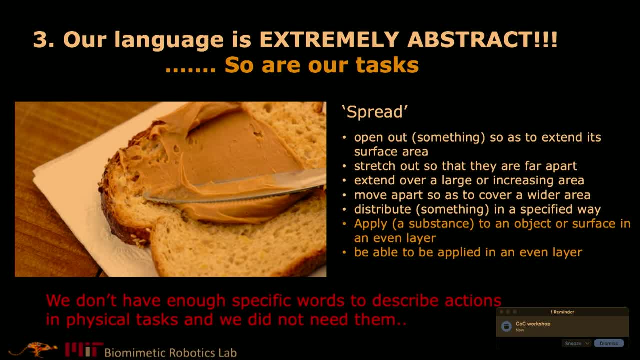 low level control where actually complex policy live in. We think our languages are so concretized and then you can describe, you can do everything, I'll guarantee you. how would you teach your younger sibling or son if you have how to spread out? 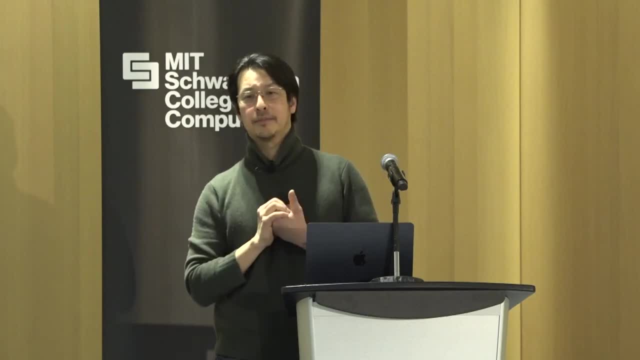 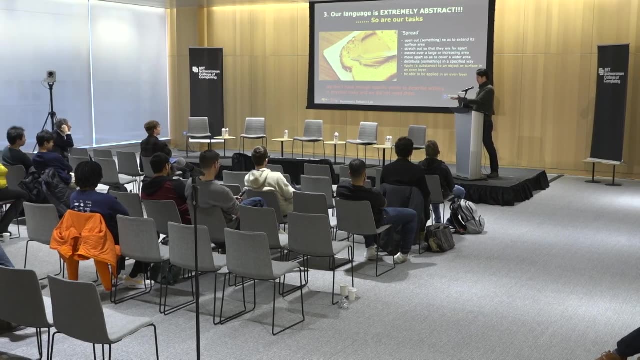 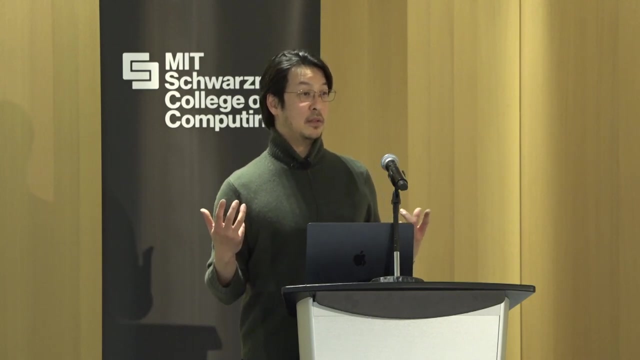 spread a peanut butter on your bread. How would you describe it? This is what I would do: Grab a bread, grab a knife, scoop out the peanut butter and then spread. well, See, you're done. How many bites of information did I give it to my son. 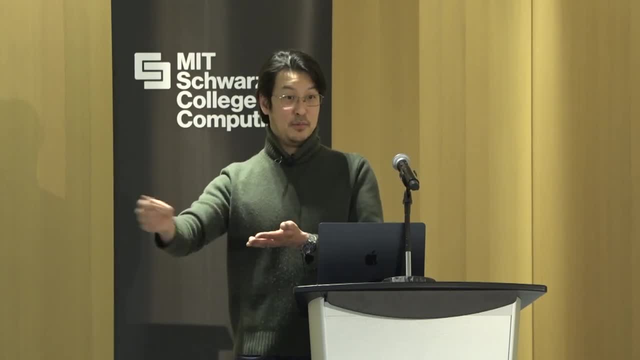 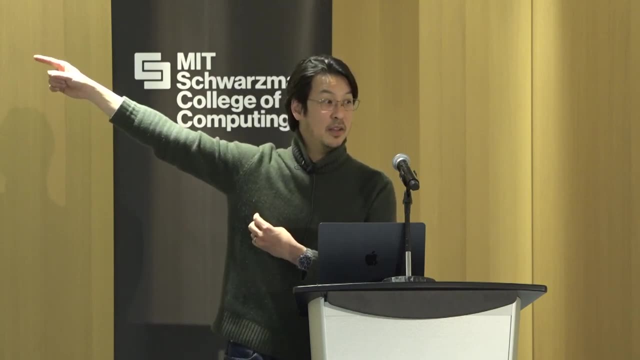 Do you think that's enough to create a policy reliably? grab a bread and then put down peanut butter. Do you even know the trajectory requirement or the force requirement? Do I even know the temperature of that peanut butter or the stickiness? I don't know. 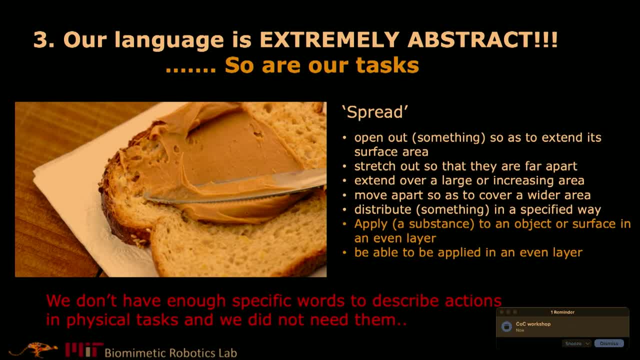 I just adapt. Those are policies. Those are not imitation trajectories. Oh, I must learn through many, many trajectories. No, no, no. Your son can learn in less than five trials because his built-in policies are doing it. Are we aware of it? 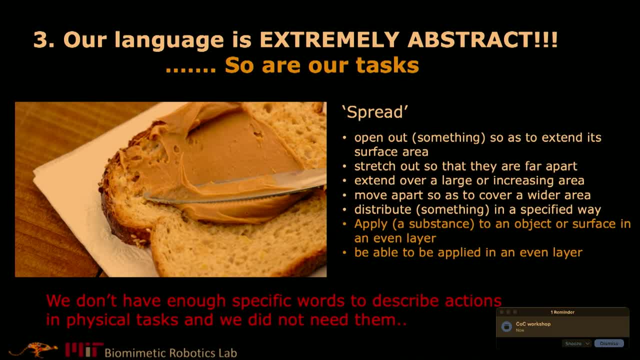 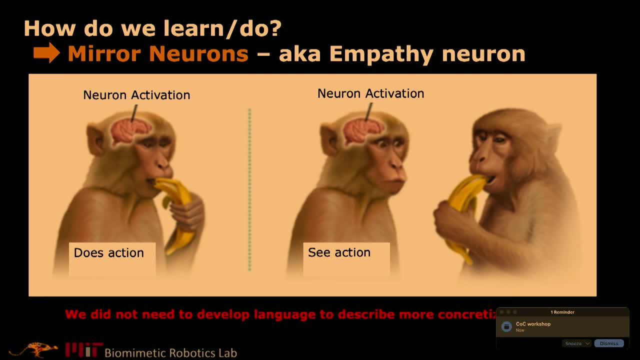 We have absolutely no idea. We think we know everything because language is describing everything, but language is not everything, because we have a mirror neuron. I'm not sure how many people know about mirror neuron. Okay, good Many people know mirror neuron. 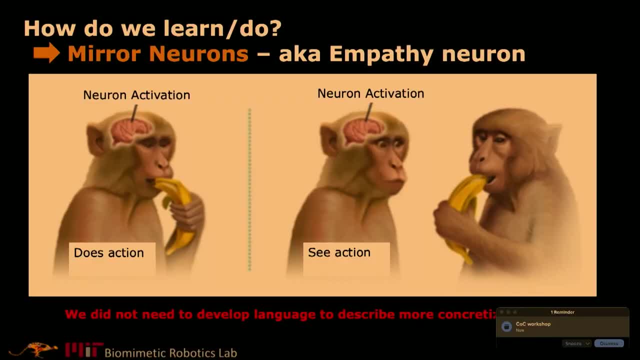 Mirror neuron, if you. the mirror neuron is called the empathy neuron. This is why we watch basketball. we get excited because when you see some other animal, other similar animal, you're human, human, other human running, you're pretty much copying your same thing happen. 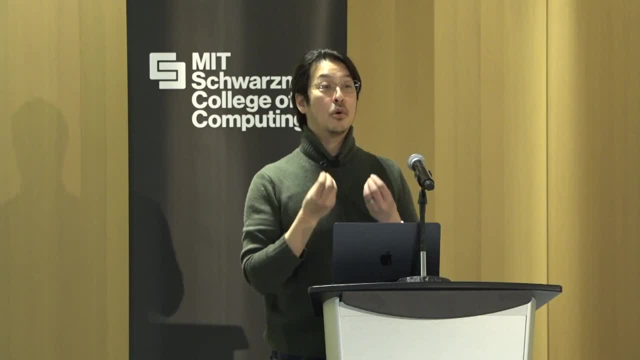 That's how we can learn things so quickly with a very low resolution information, because a mirror neuron take care of everything. Grab, like this brush, like this, a little harder. Oh yeah, good job. good job, Now you know how to do it. 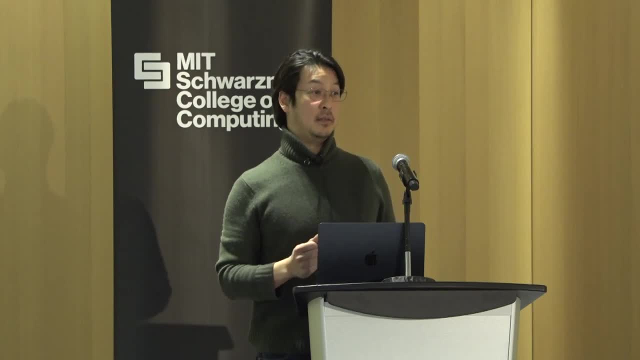 Takes a few second and then people learn policy Mysterious. I don't even understand how mirror neuron works and I don't even dare to copy this, but that's why our language doesn't need to be that detailed. What is the purpose? 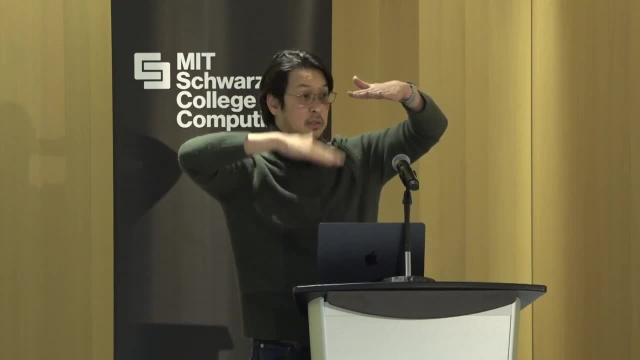 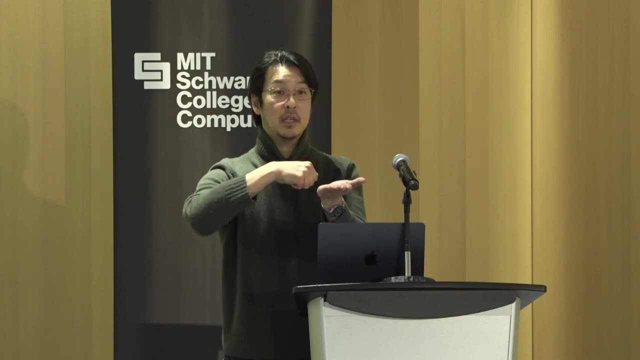 The purpose of language to communicate Below this abstraction level. all these detailed policy level mirror neuron take care of it. Why do we even develop a language? That's why we don't have any expression about how to put the peanut butter jelly to the bread. 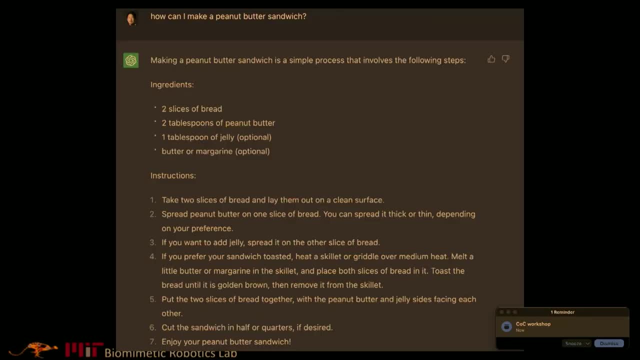 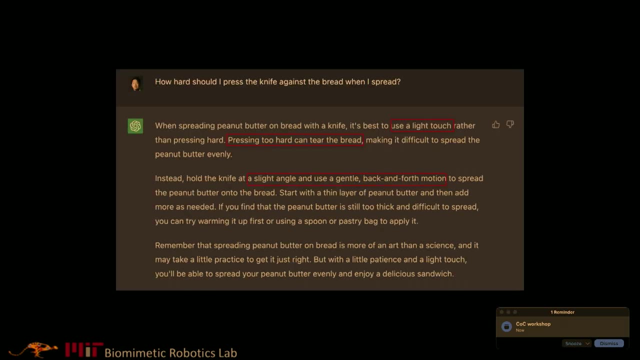 I guarantee you, if I ask you to write down instruction on peanut butter jelly sandwich, nobody will do better than LLM. So I push really hard. I keep on saying how you do it and then what motion and like. what do you mean by back and forth? 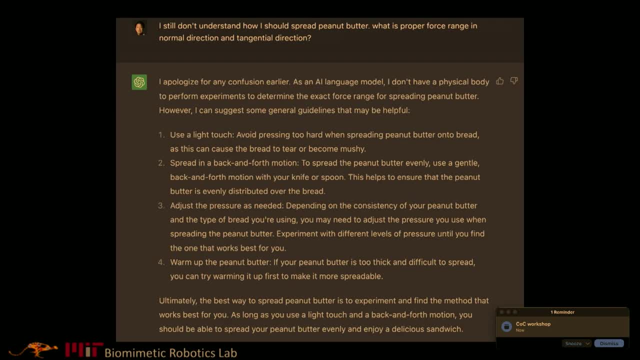 And then, like he says, like gentle sawing motion, You keep on saying something seemingly tangible. It's like I don't understand. Give me the actual like, trajectory or force and like: sorry, I don't have a physical body, In other words, I don't have data. 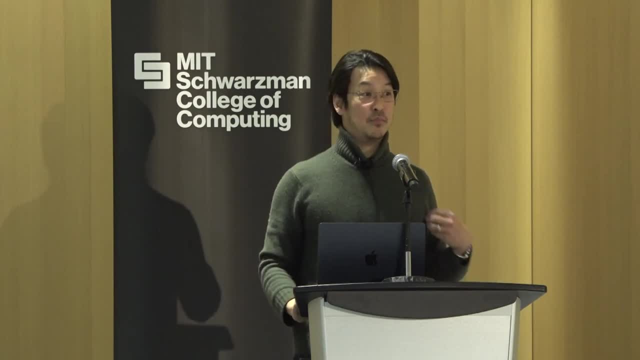 to even communicate with you, right? Does anybody like? pour the data, millions of data, of peanut butter jelly trajectory as a force, considering how firm the bread is, considering the temperature of the peanut butter. So I have a little bit of suggestion. 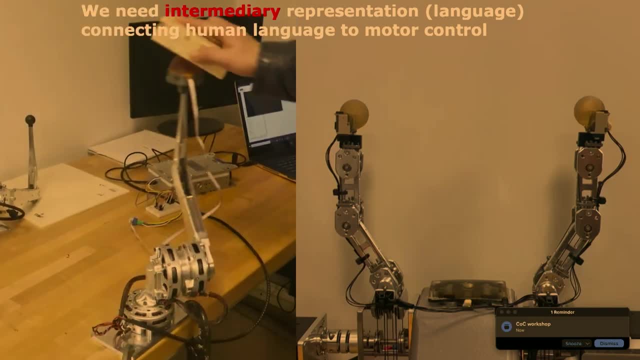 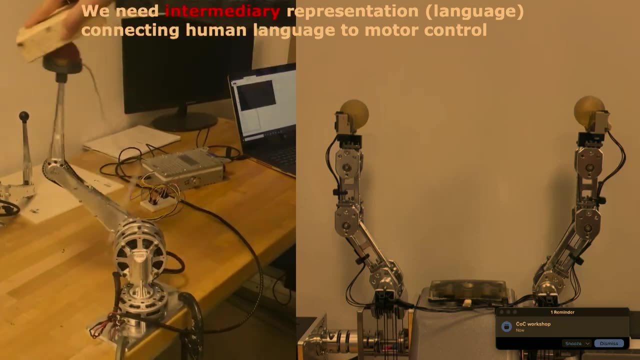 I'm not saying this is gonna solve all the problem. We need to build the layer of reflexes that it's mostly taken care of by your mirror neuron. How, I don't know, We've been building by hand, But at least this is simple enough. 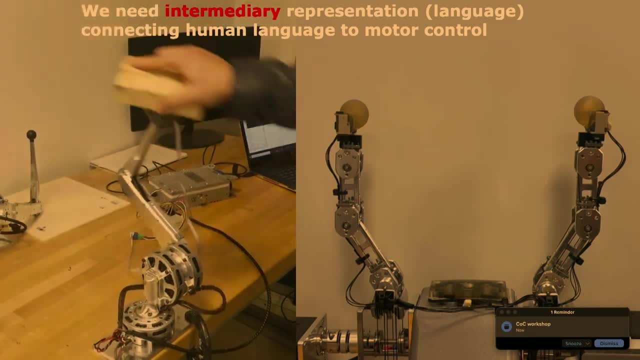 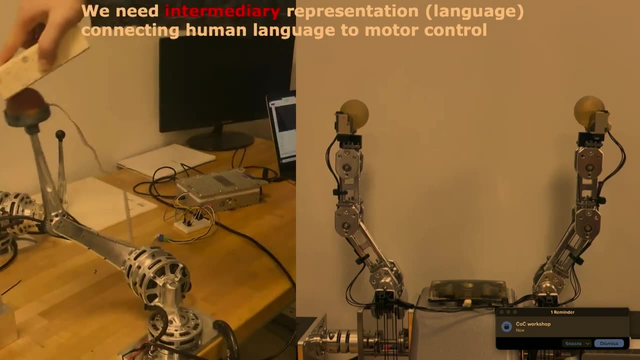 but it's a versatile enough reflexes so we can actually higher level algorithm can take advantage of it. In that way, your high level algorithm or RL doesn't need to spit out nitty gritty- X, Y, Z, position or force profile at all. 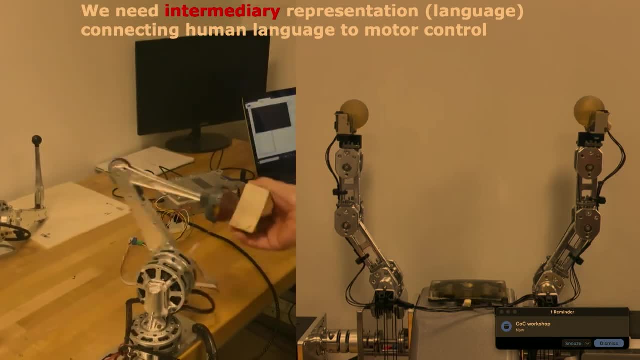 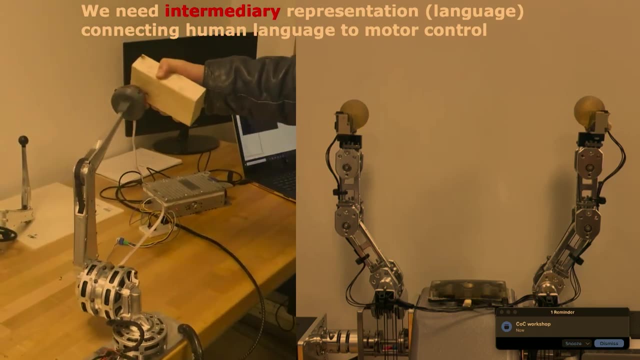 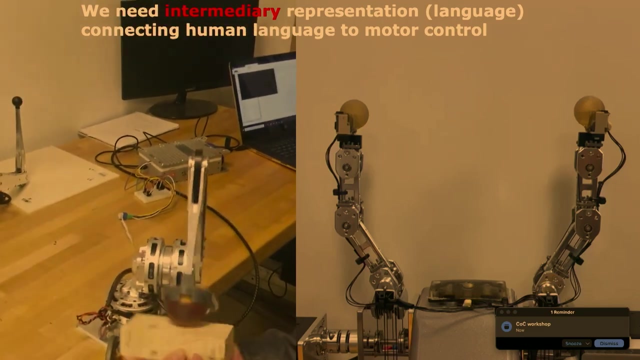 You can deal with the information or policy much more abstract level. Use sticky reflex with the parameter 10 and five. Do it? oh, it didn't work. Try to reduce this number based on your data Instead of commanding PD control law on some rent trajectories and another reflex I can show you. 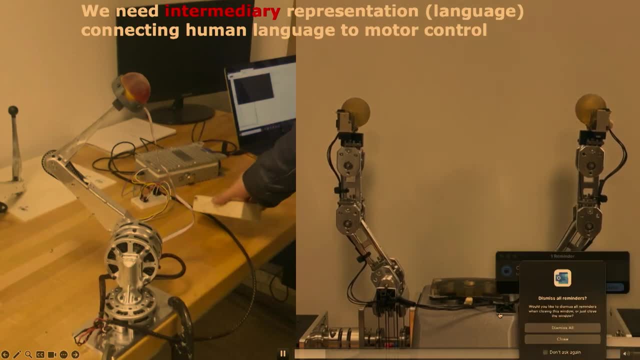 This is. we call that gliding reflex. Oops, This is inspired by trajectory planning for any grasping motion And then eventually you want to wrap around the object And then, if you have this kind of reflex, you don't need to even have a motion planning. 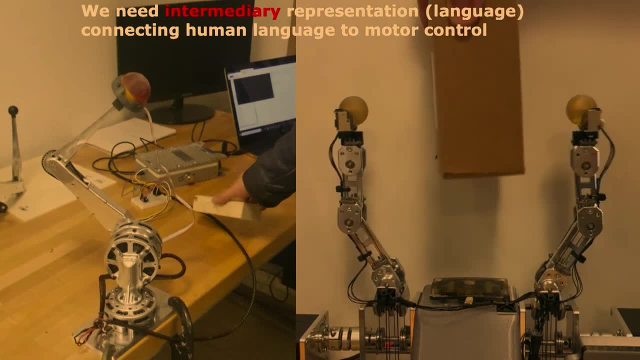 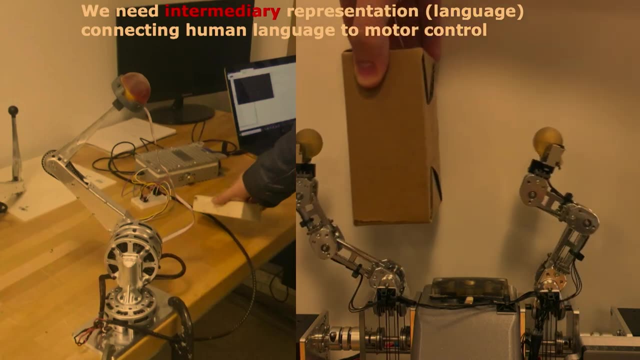 every single time, which will give you a long trajectory if you have any glitch on your motion system or 3D scanning. your perception issue: I heard somebody's talking about perception. right, You probably missed that talk, but perception has a lot of challenges still. 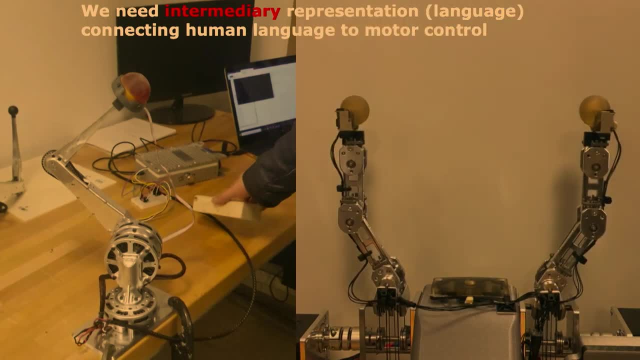 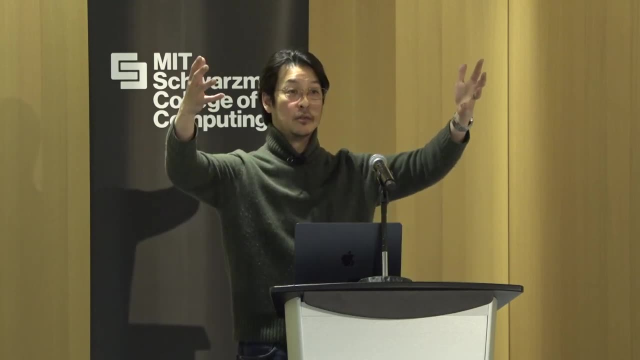 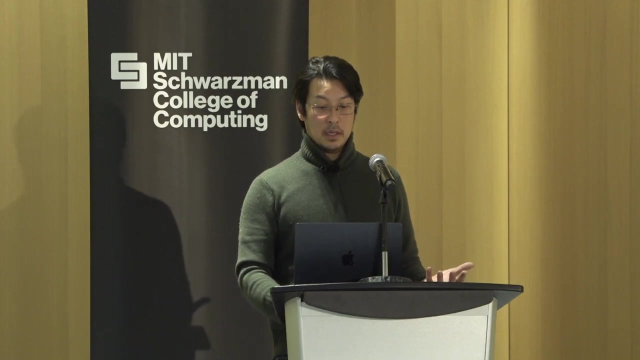 So we're trying to mitigate those high noise brittle system by having more reliable, a predictable feedback loop at a lower level. So your RL training doesn't need to command all this high resolution information and policy training. And then, if you combine a few reflexes, 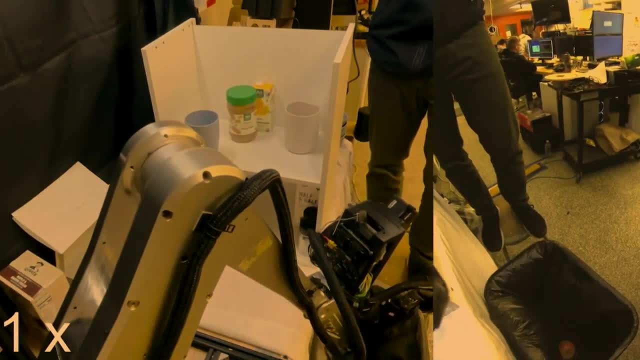 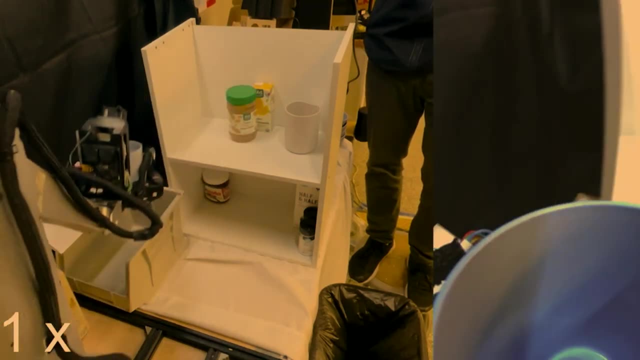 you can do things like seemingly simple, but in the human speed, this is one X And then adaptable. we move the object and it still follows: Is perception. is that fast? No, the perception is not even involved once the arm is moving. 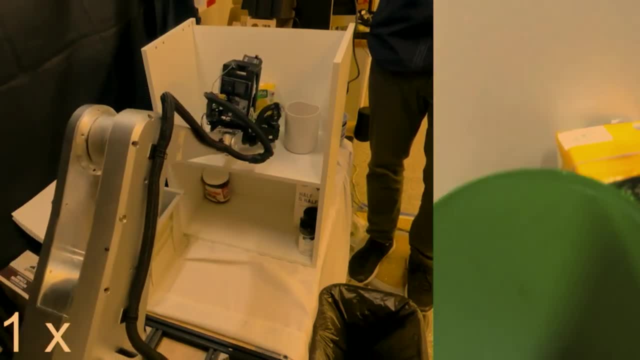 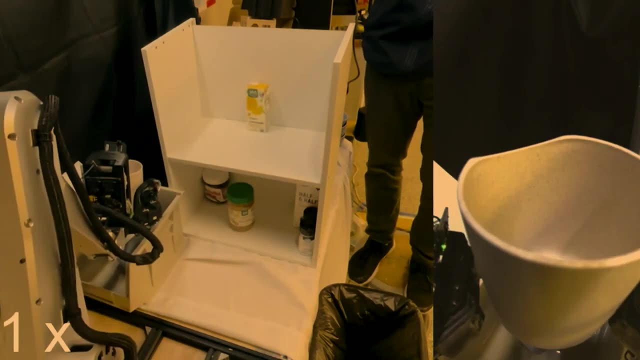 Perception, knows where the object is and go, and then he's take a slip And then reflex take care of the rest of them. It's simple demonstration, but potentially this can actually transfer to even more complex thing. There are a lot of challenges. 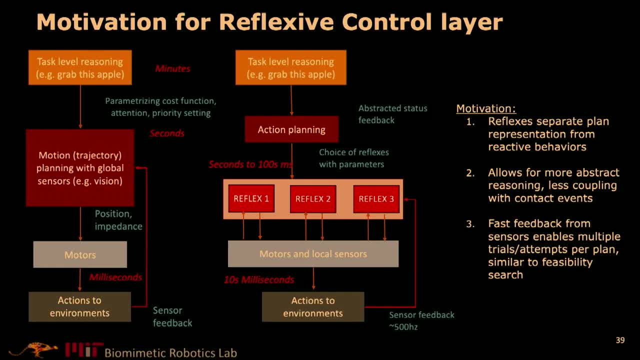 but at least this give us hope to execute things in the right bandwidth and right speed, Because almost every possible algorithm, structure or things that happen in robotics world, there's a one gigantic optimization RL. just command every single nitty gritty decision. It's not hierarchical. 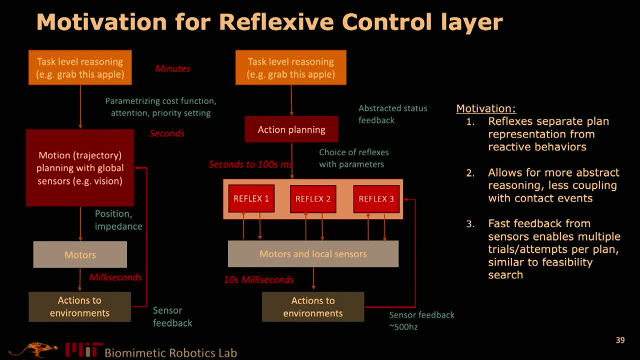 which is analogous to if you have a big company and then, if you have fire in office, you're calling CEO to make a decision, basically Considering every parameters you know. tell me what to do to put out this fire instead of: oh, I have my own policy, I'm going to take care of it. 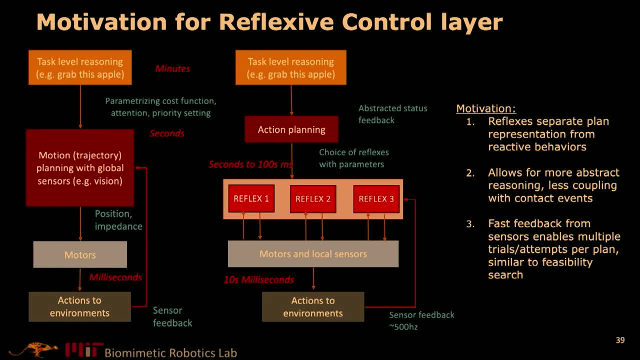 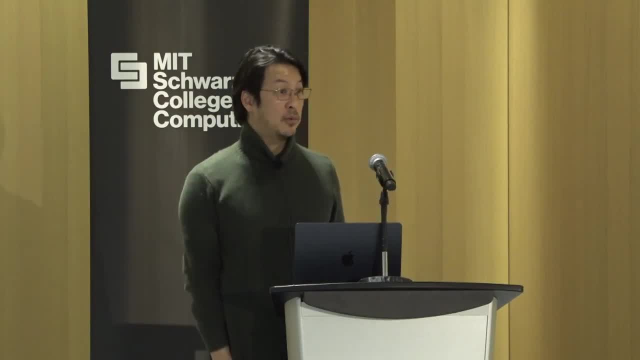 When common sense is it optimal? I don't care If I wait. something much worse is going to happen If you pick up something like you. just pick up something from your pocket, right? You don't want to wait and then get the command. 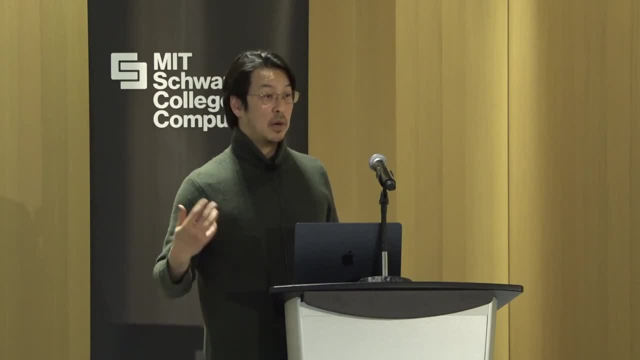 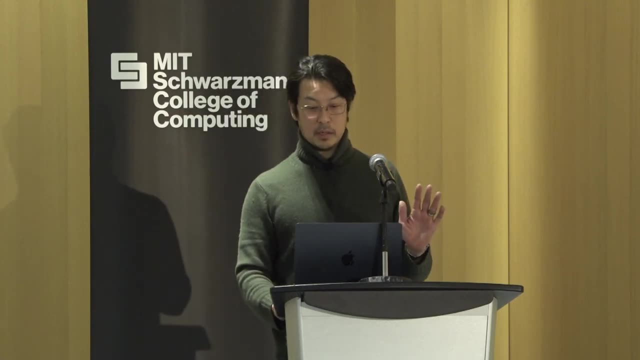 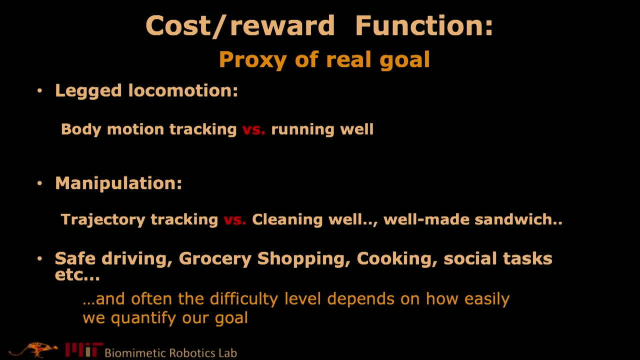 from your cerebral cortex. give me optimal solution. Your object is on the ground already. if you react quickly enough, We can have a whole thing about optimality and cost function which is just coming up. I don't think I have time to explain all this. 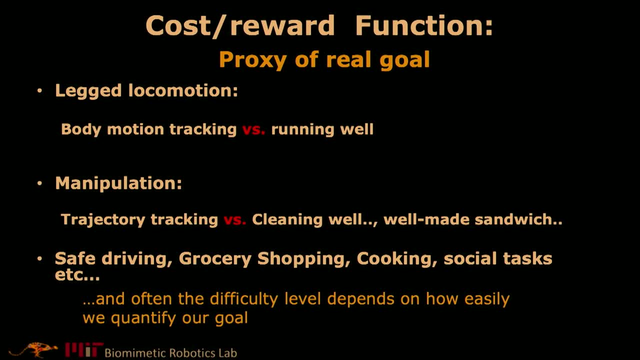 but optimization is not the only solution, and sometimes they're good enough. execution is much, much harder, and then we still don't know how to do that. well, And if you don't have a cost function, nothing is going to work in the real policy world. 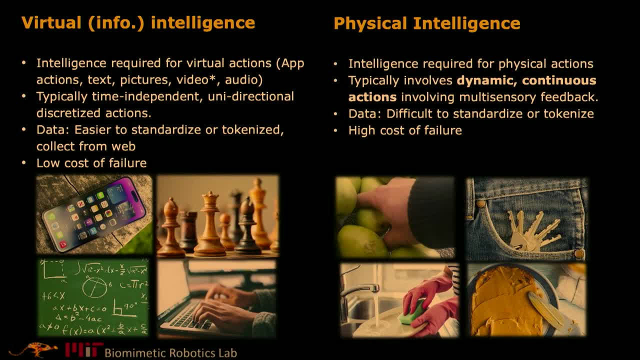 And I don't think I have time for this, but you can probably guess, based on what you listen, why virtual intelligence and physical intelligence is so different, where everything is free forward and static, It doesn't even have a dynamics between information. 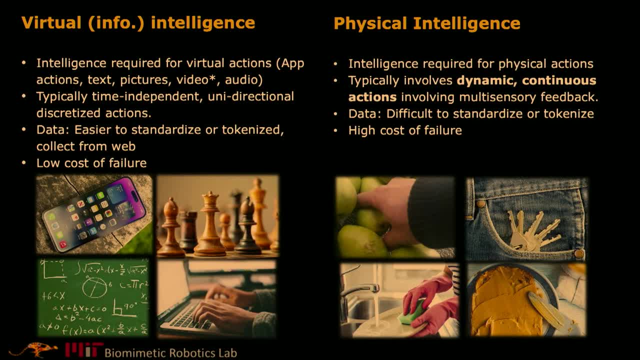 I have a launch or I have a launch. There's not much difference in information. In physical intelligence, everything matters: Dynamics, speed and a lot of times this is in subconscious level in our brain. we just don't know much about it. 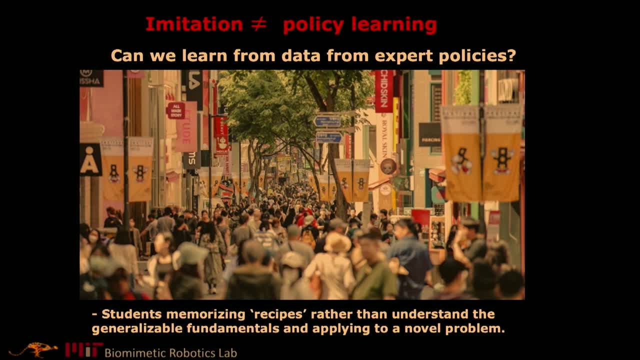 We don't know how to judge about it. I already talked a little bit about it, but I want you to think about it after my talk. Can we learn from millions of people walking a million hours if you have all that motion capture data? 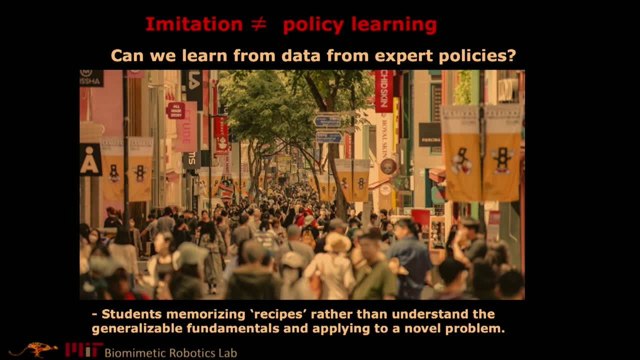 can we learn walking in humanoid? We have tons of data. we have a lot of people. Can we train our humanoid to walk very reliably based on that data? I want you to think about it. Otsukawa is nothing to the roboticist, say this. 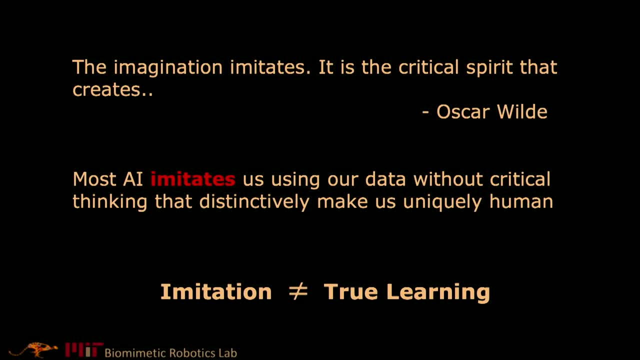 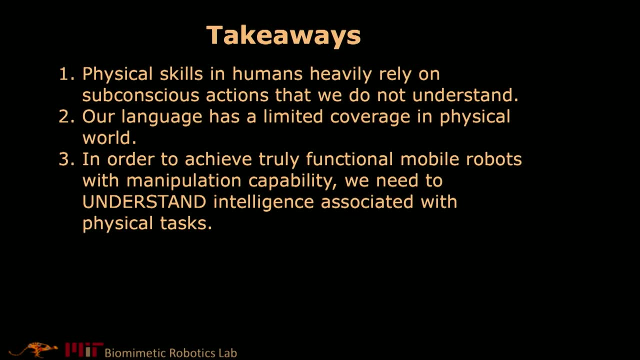 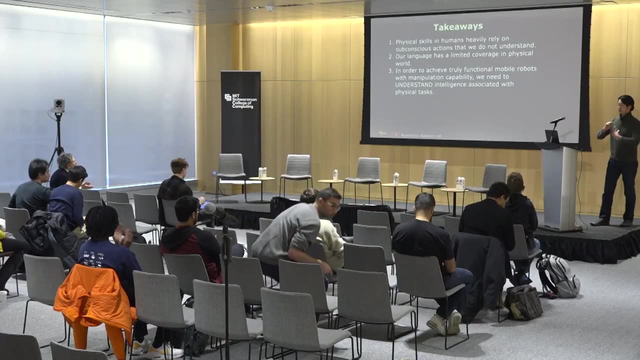 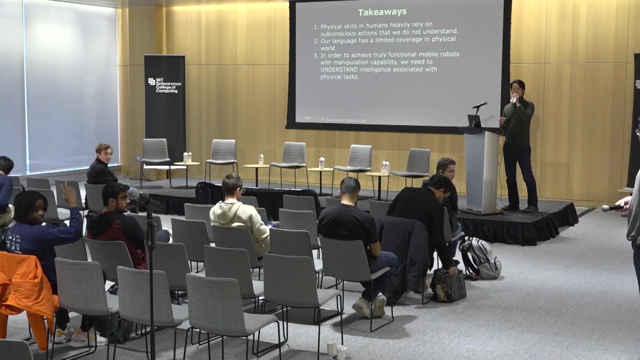 Imagination, imitate. it is critical spirit that creates. I want you to think about it. If you are any working on machine learning. I will conclude my talk and thank you for your attention. Any quick question? Yeah, Thank you for the talk. 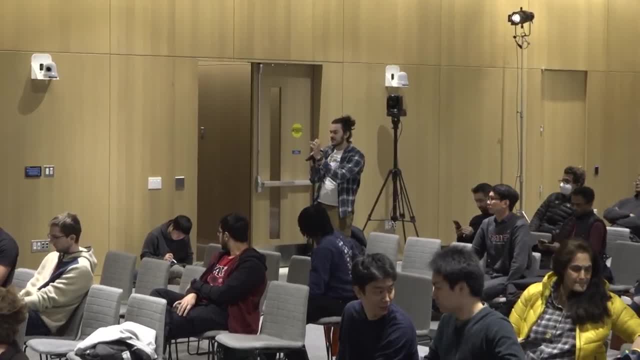 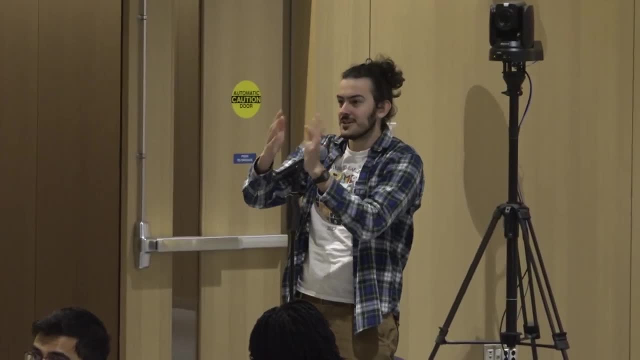 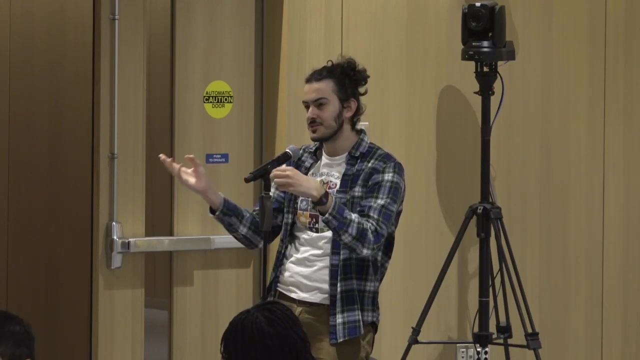 I was wondering for those atomic reflexes that you showed. you showed two examples. What's your approach to? well, two things: How do you decide what is a reflex to create? And then, do you create them or do you let them be trained by machine learning? 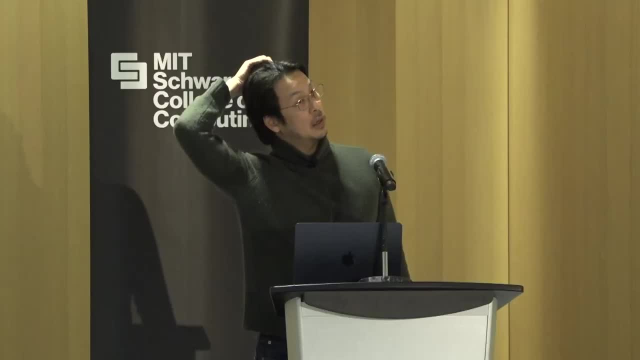 things like that. I think some reflex can be trained, but we plan to make at least four or five reflexes and then tune and then each will have some parameters. But we choose based on how useful they will be in some target performance. 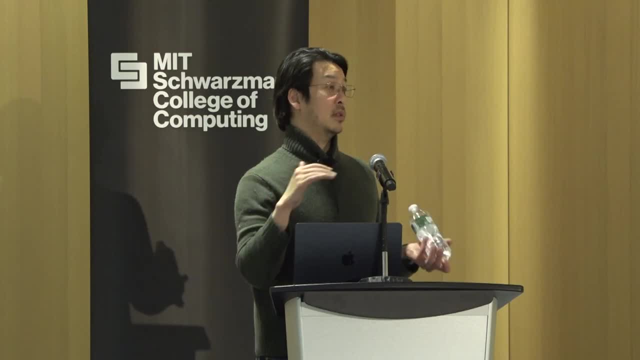 In our target performance is pick and place. So in that case, what will be useful? reflex, Independent from the situation, independent from the object. So I'll train that first, and then some reflex might have to be trained based on RL, But it's a very slow process, as you can think about. 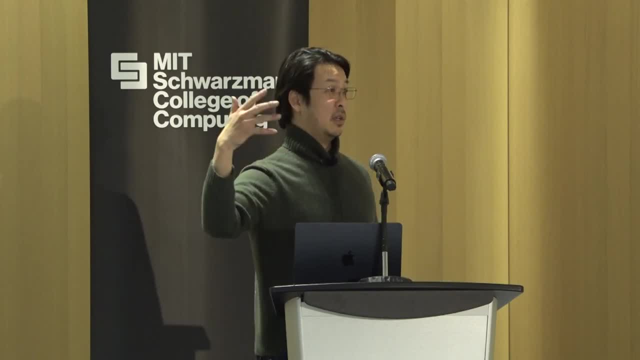 We are heavily working on simulation right now because we can train based on real hardware data And then we need to recreate digital copy of the reflex in the real simulation As anybody play with the simulation. all the models, the content models are crap. 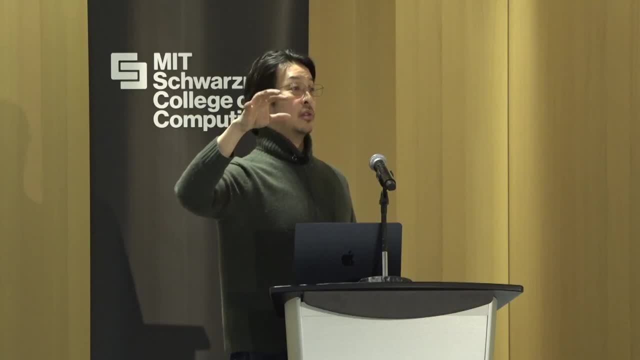 And most simulation tool doesn't even allow us to change. So we're actually working on one tool that actually at least have some glimpse of custom ability. So we're actually working on that. Once that is working reasonably, we're going to have a digital copy of this. 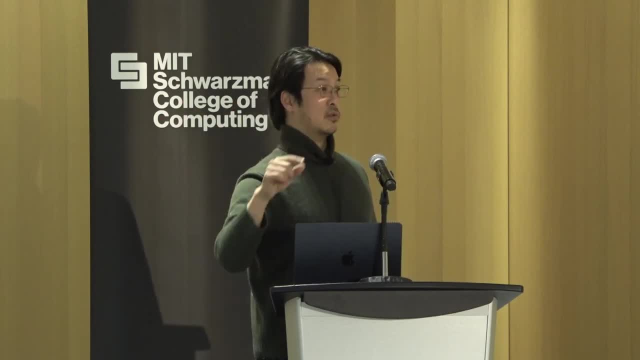 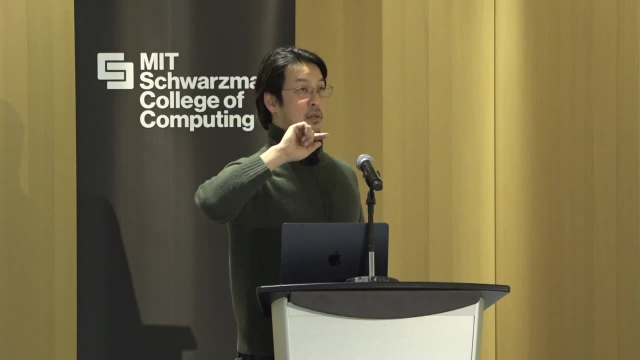 reflex on virtual world and then we're going to train it. But that's a really important and critical question. A lot of people have trouble creating a target task because what would be the useful skill robot should do is very, very hard thing to decide at this point. 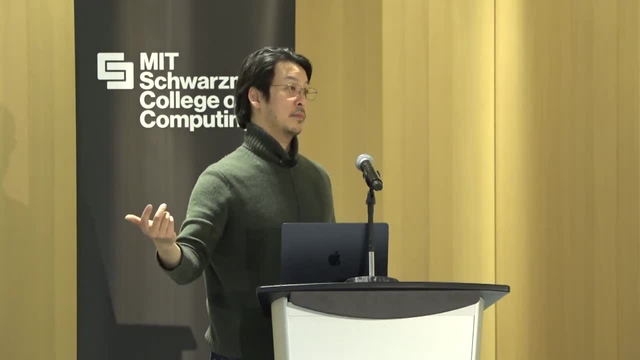 And that comes with like, what reflex would be useful? So we are playing those two together. So whether like: oh, I don't want to create a boundary so that we don't need gazillion reflexes, We want to do with a minimal number of reflexes. 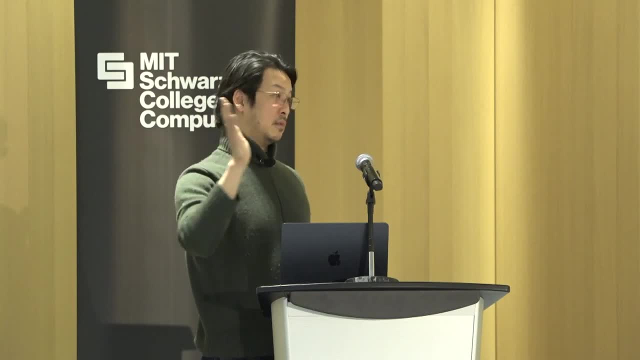 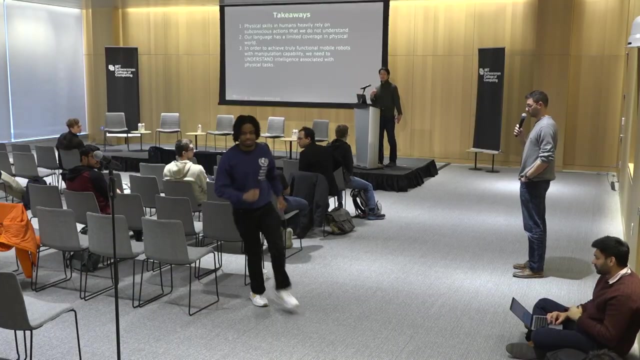 Oh, maybe then we can cover this Still ongoing problem. It's very hard and that's why it's not scalable, But again, I don't think we should build a robot that can do everything. Thank you, Yeah, One more, and then we'll wrap after this. 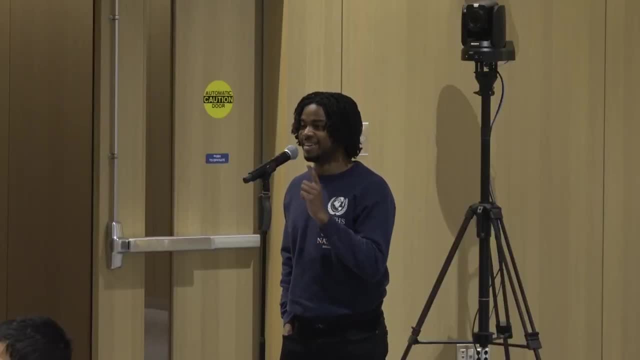 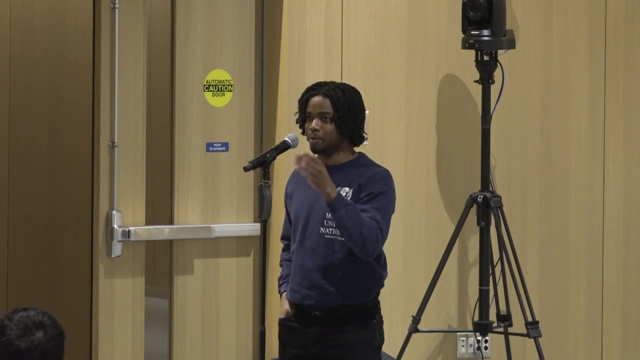 Thank you. Yes, to answer your question, I took 2007 last spring. Do you think that we would reach like better physical intelligence faster if we were to have some breakthrough where we can just stick a bunch of sensors on robots and we have more cheaper sensors? 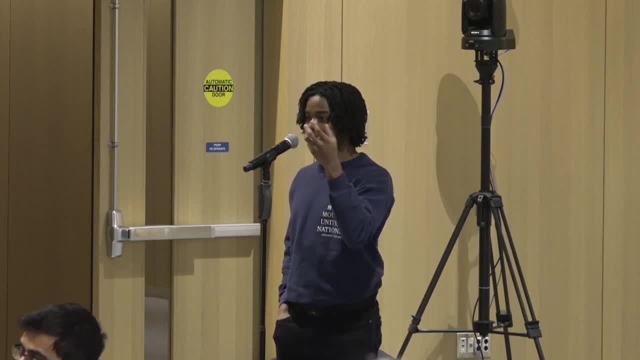 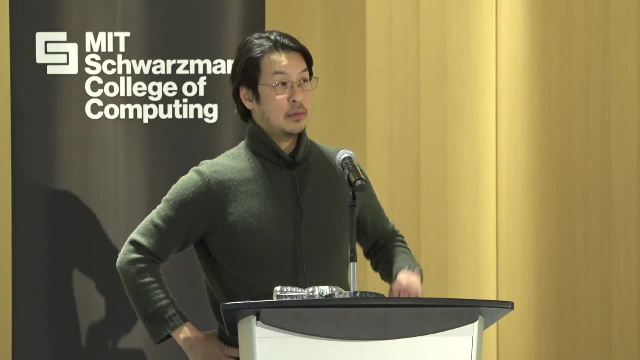 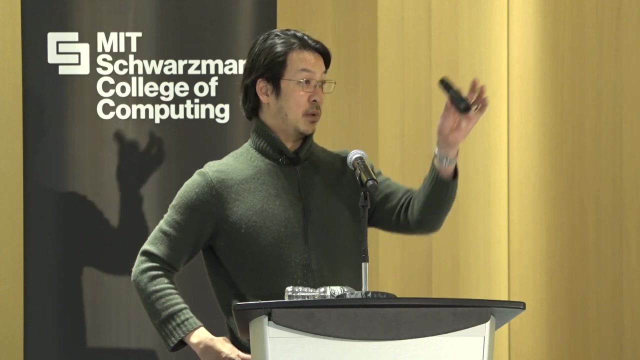 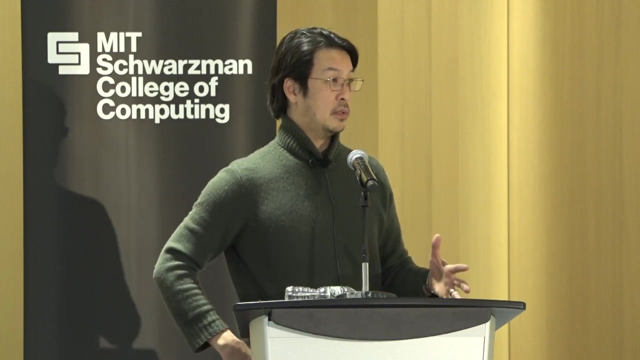 Or is it? there's some like underlying way that physical actions are represented that we just don't understand yet. So if I ask you to do some absurd task you've never done before with this, then you would do it. And then you can do it because you have a full knowledge of dynamics, or we have. 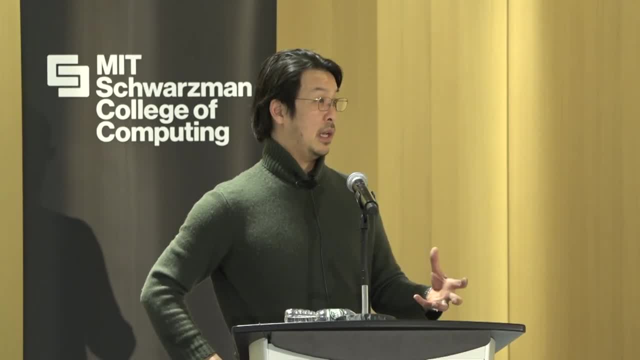 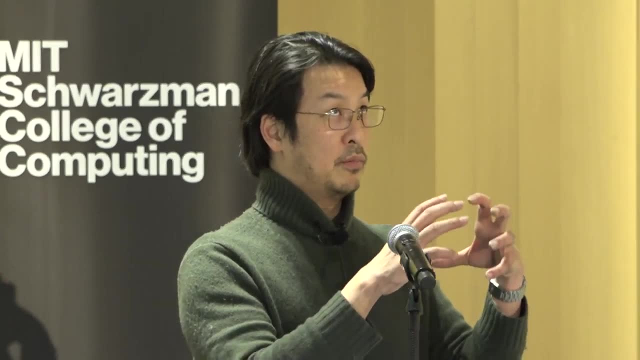 some understanding, Some understanding of the dynamics, And if I ask you to do it, if somebody else do it, they will do execute differently because you're a model of predictive. most probable model of this is actually different. Similarly, you learn free by dynamics. 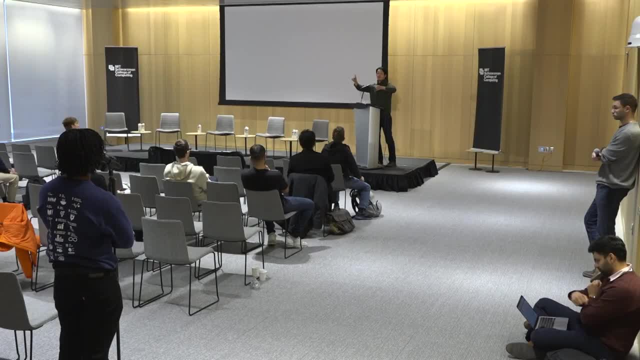 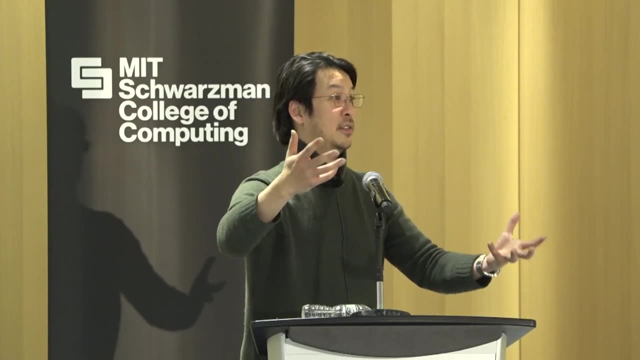 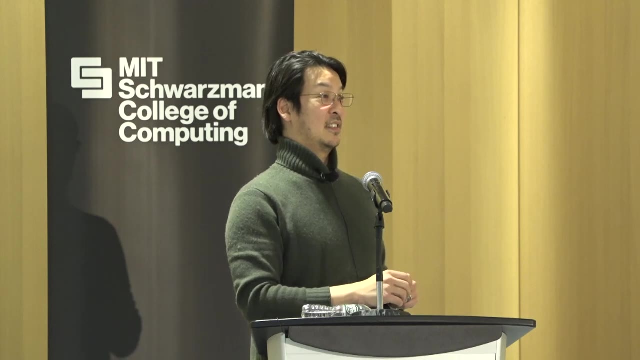 If I teach free by dynamics, everybody build a model of free by dynamics differently. So that's basically a understanding process. The thing is, how do we tease out and then evaluate That understanding? So physics understanding and theoretical level is very different from oh do. 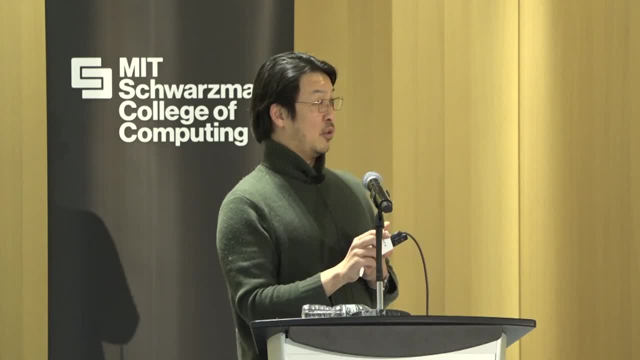 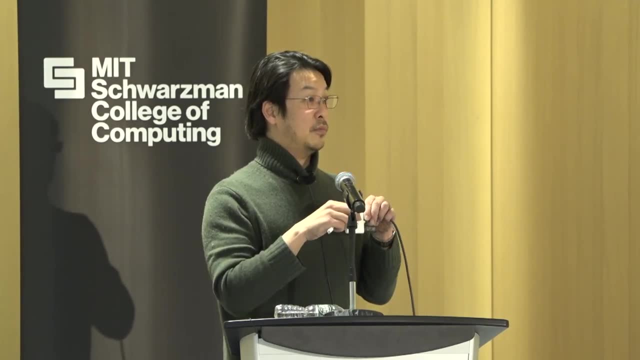 you know how to plug this in. Do I need to understand FQMA? No, no, no. You just need to understand the predictable physics between this USB or HDMI. If somebody's done a lot, he has a better model, more detailed model. have a. 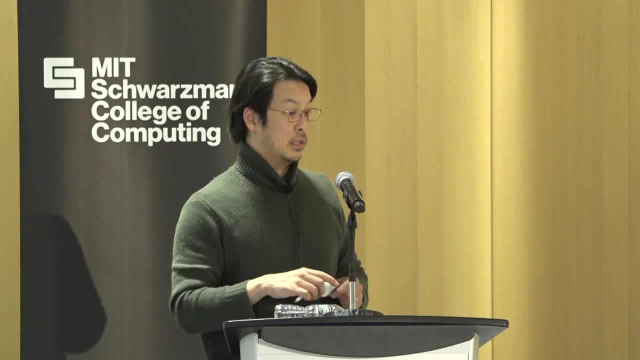 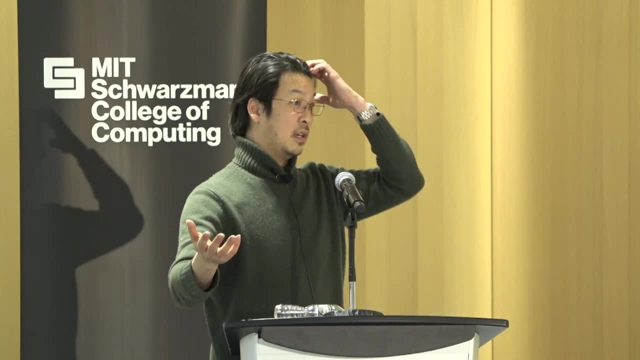 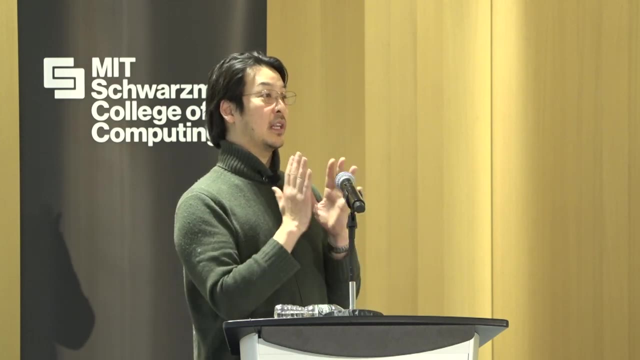 little bit of data driven policy built in right. So people debate about the collected gazillion data, So hopefully it can create its own reasoning, physical reasoning as general as FQMA. I don't believe so. I think we should really target it. 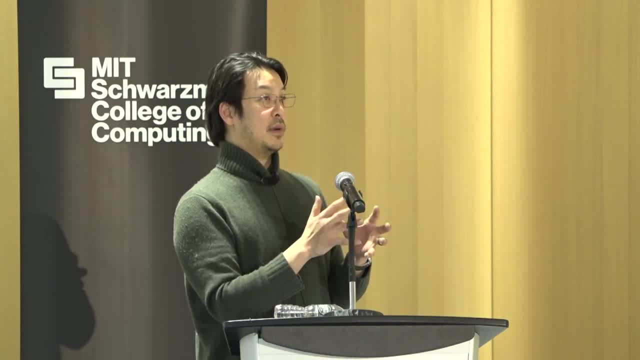 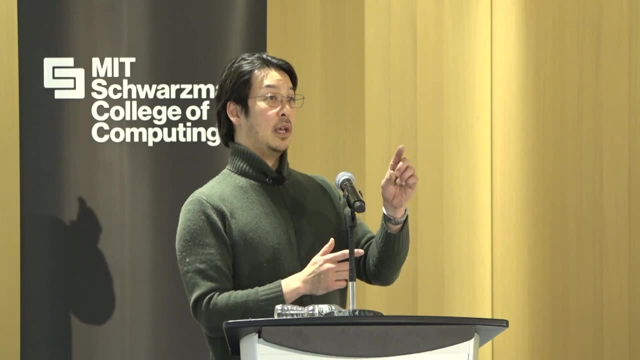 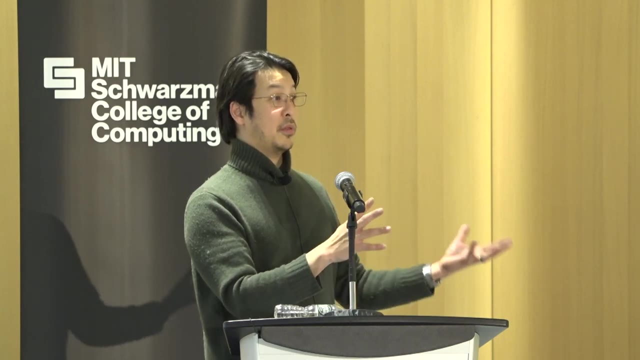 Target task and then try to minimize the amount of data requirement to generalize that task. So I encourage you to watch the Aaron Parnes. He's an Amazon stowing automation guy and he gave a talk at Stanford a few months ago. He's fresh new. 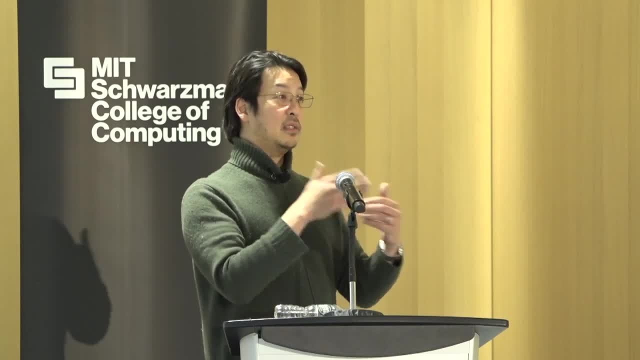 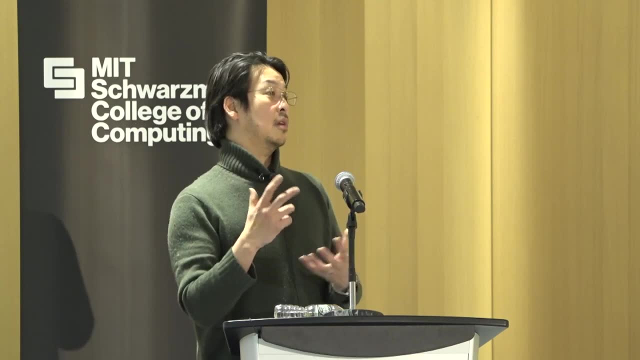 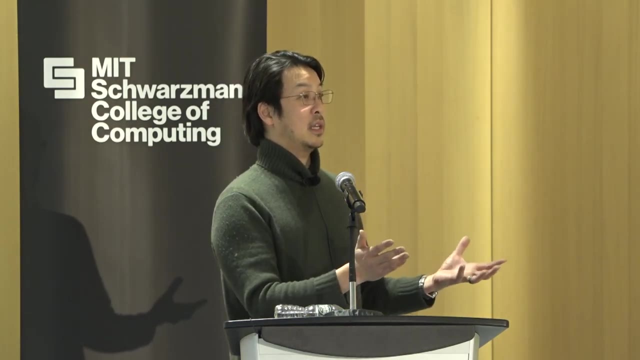 He's that's kind of like very few, like tangible automation application using machine learning, vision and everything. He doesn't use any of this common sense. He code as much as possible and then leave very little for machine learning, because again you have to hit 99.10 nines afterwards. 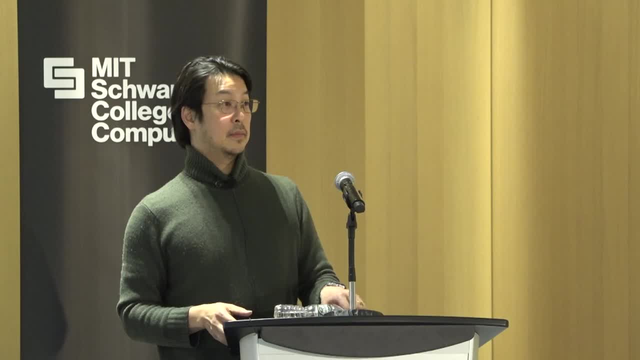 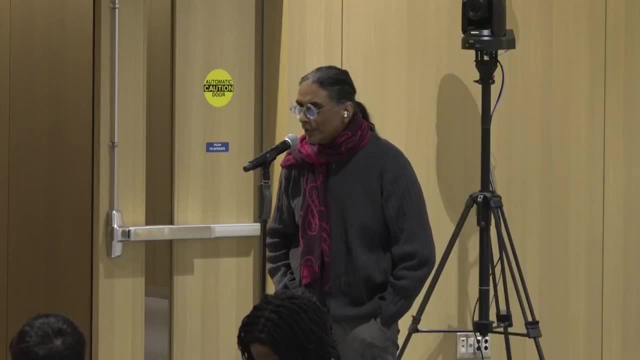 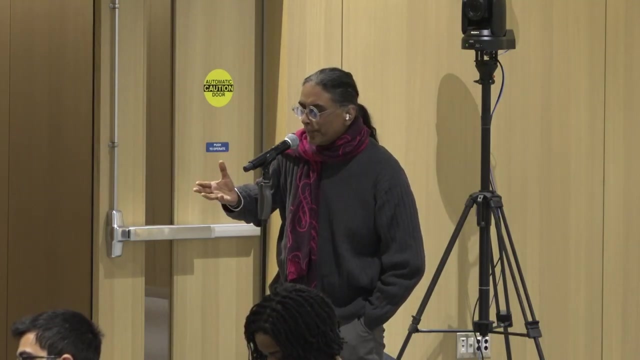 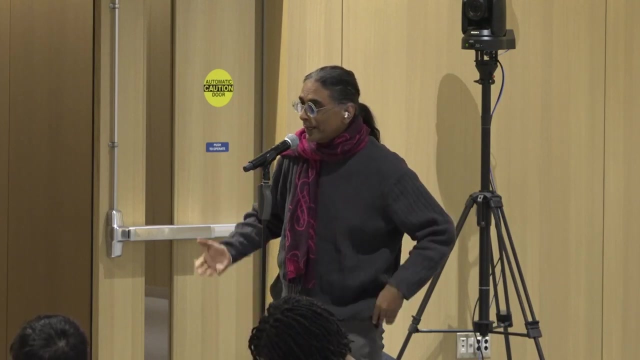 So thank you. Yes, So in something like Amazon, when you're doing pick and place on objects. so let's say the basic idea, we know, but if you have a person, the person usually wears a hard hat, wears boots, where eventually something's going to. 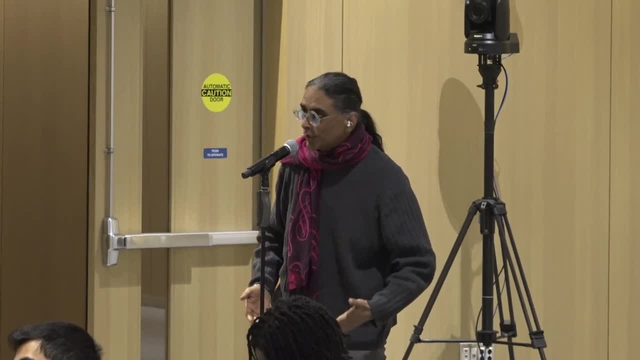 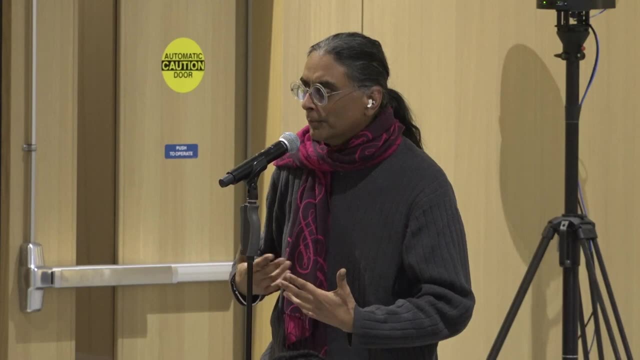 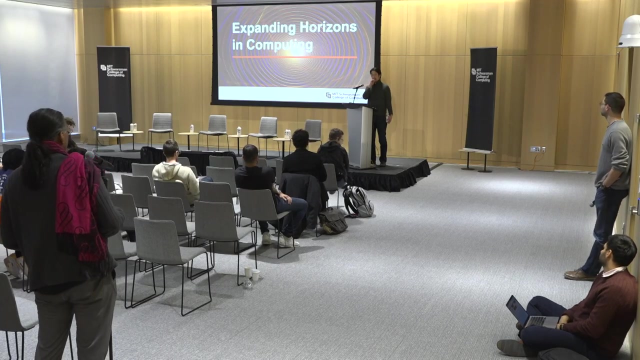 fall down on you and will hurt you and it's going to cost a lot of money and you want to minimize that over the object itself. Do these robots have some sort of? do they incorporate themselves into their model So that they make sure that they don't hurt themselves? 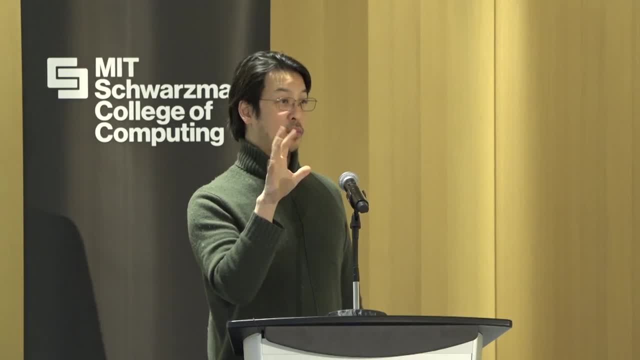 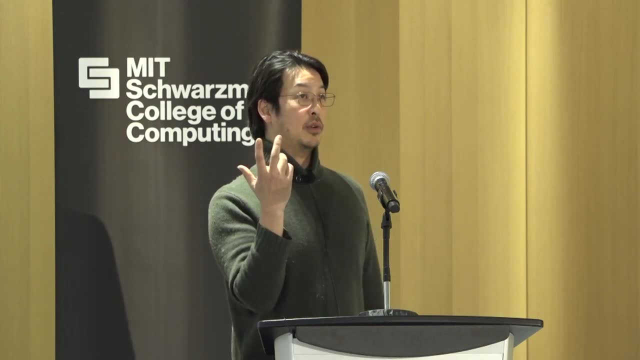 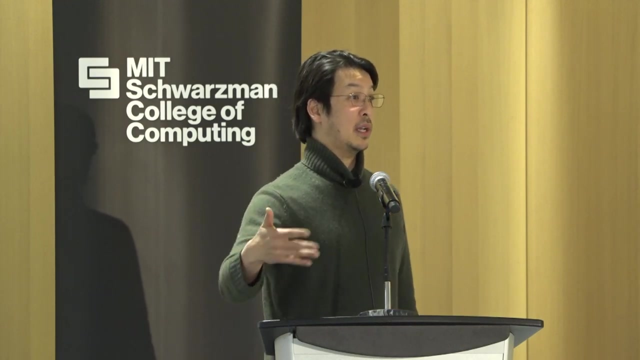 I mean there's a lot of like algorithms that prevent from those actions. But like when I bring my son to some factory, I will say, Oh, be careful, be careful, be careful, And then he will be more likely have a less chance to make a mistake. 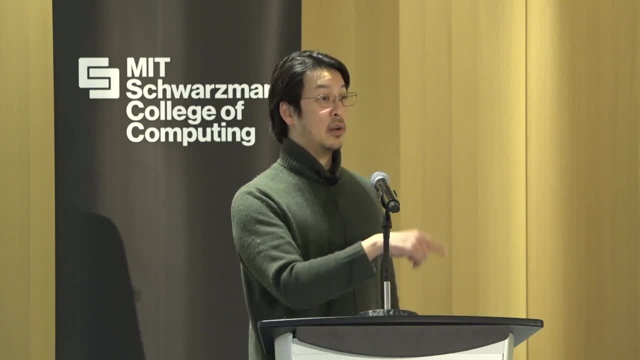 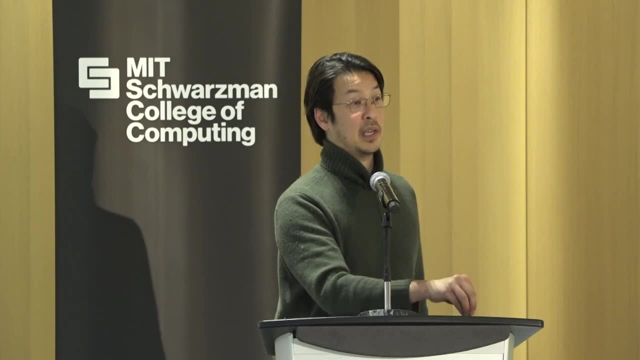 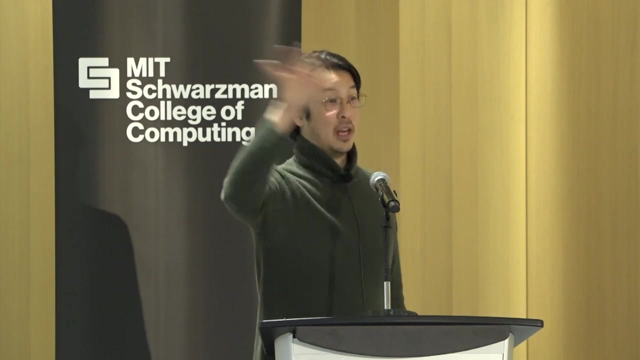 We can't do that to robot Unless generalization of damage. Can we code a damage concept of damage so that we can be careful to minimize damage? How many words that I said. that few bites of information, generalizing, understanding of that. I say understanding again in machine learning world. is it possible in 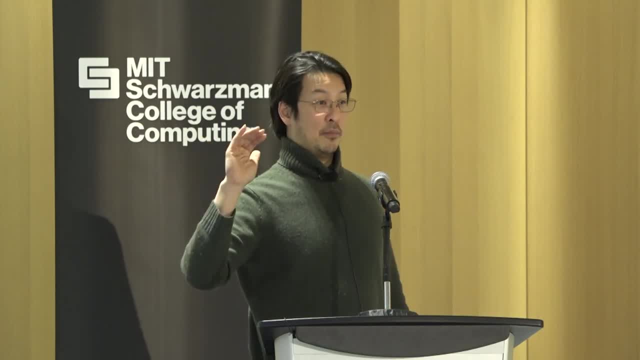 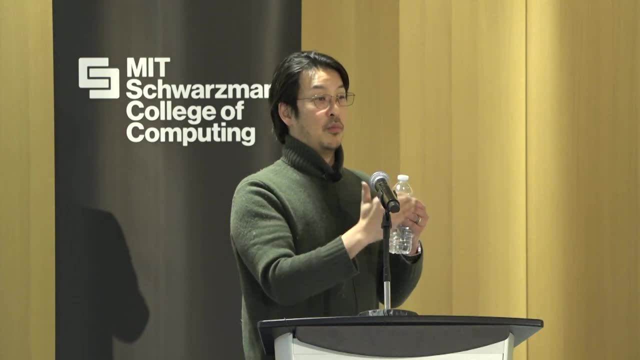 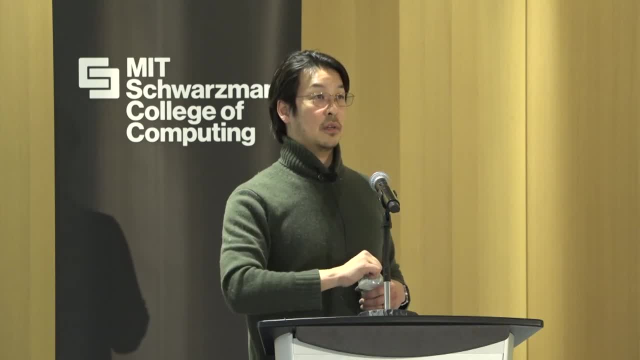 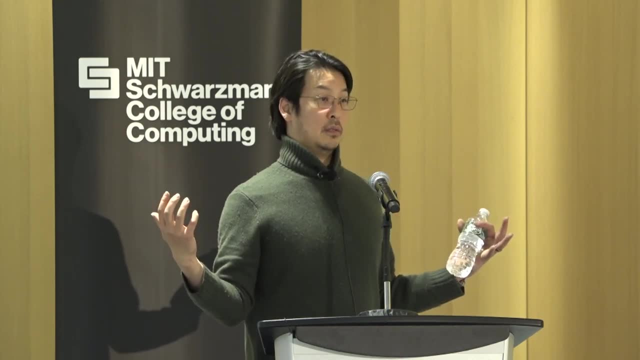 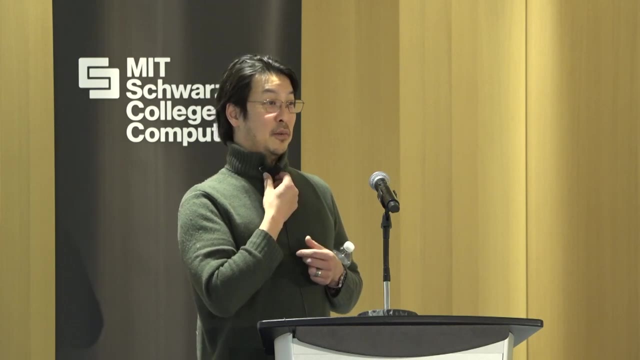 That's how we supposed to move on. I don't believe we're going to have some magic data set will understand every possible physics. Even human cannot do it. So yeah, that's my personal opinion. Who knows? We didn't think LLM is going to come out. 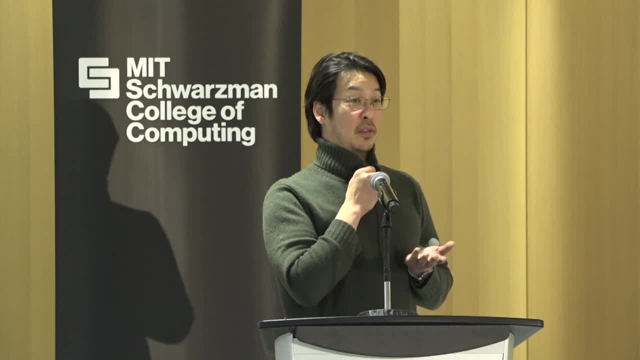 But you can logically think of LLM. the language information was there. It's been there for a long time. Yeah, All right, Thank you very much and have a good night.